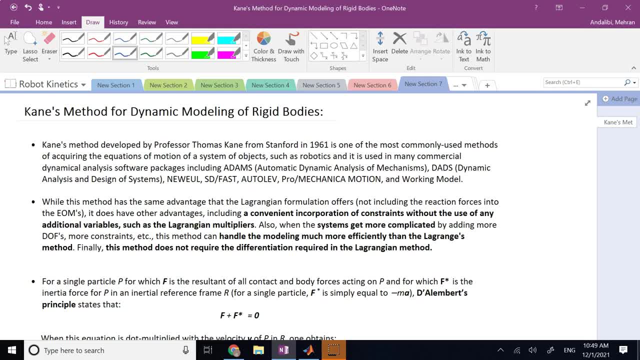 The Lagrangian multipliers. In this method we don't need to do that. So that's why in many commercial software packages for dynamic analysis of rigid bodies, robots and so on, you see this method is used specifically, like in Adams working model, the pro or mechanical motion right auto lab and so on and so forth. So this method really is an interesting method, efficient method. 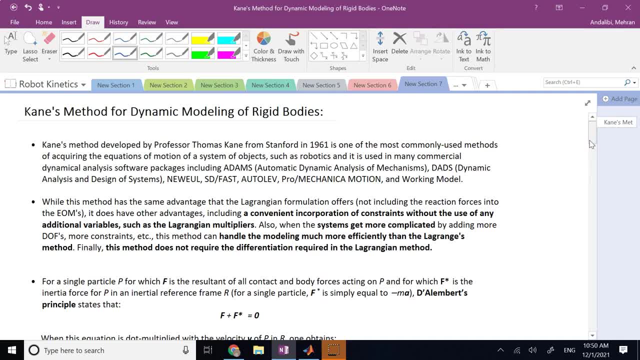 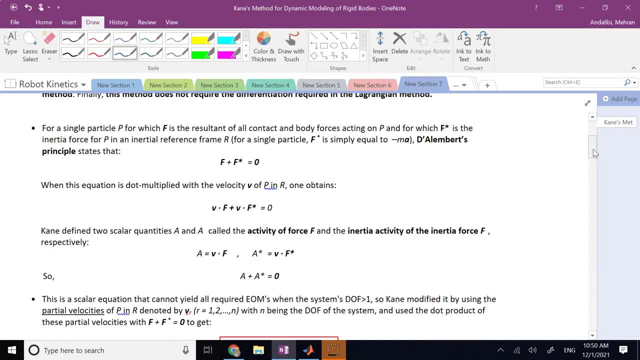 And I decided to include that, aligned with the two others. So what does this method do? So it starts with the D'Alembert's principle. that in D'Alembert's principle. basically, if I want to put it very simple, instead of the second law of Newton that you say F equals ma if mass is constant, you say the second law of Newton is like this: 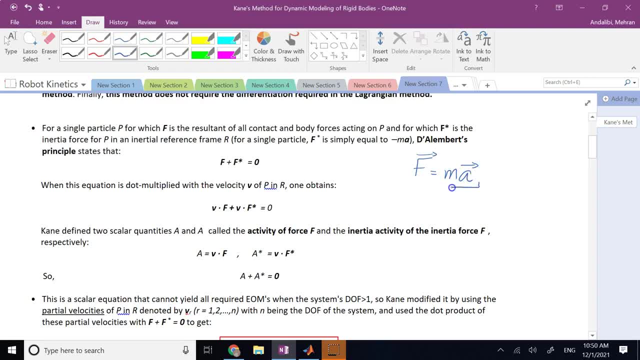 The D'Alembert principle says that Let's call this mass times acceleration a force, and we know it is called an inertial force, right? So it calls that F star the inertial force. And then the D'Alembert's principle says: instead of saying F equal F star, you can also say: the system is like in an equilibrium where the F and the F star are kind of constant. 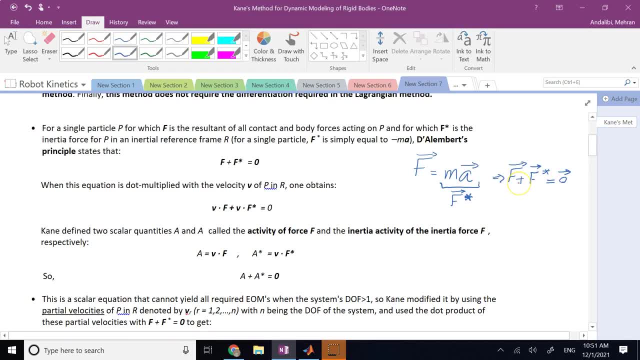 So it's like a constant canceling each other. So another way to describe it is to say: F plus F star equals what Zero, where F is the actual force applied to the system by the external environment and F star is the inertial force in the system due to the acceleration of components. 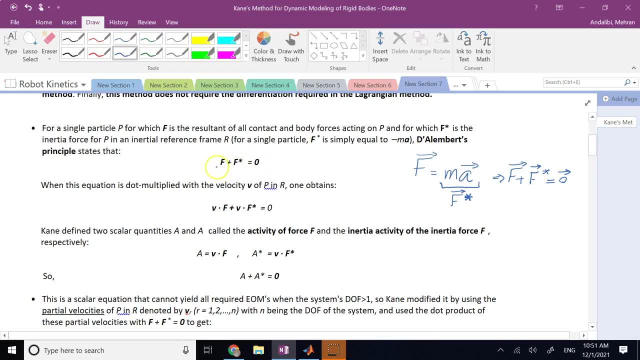 So another way to write Newton equation is this Good? Now, here we are dealing with vectors. In order to go from vectors to scalars in the Lagrangian method, we multiply F by what? By dots, dr, and we make it a work term. 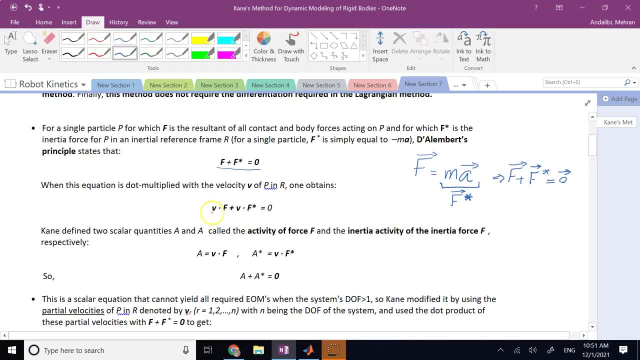 In here. it dots product both sides by the velocity, So it says V. if this is the whole thing is zero, then I can say V dots the whole thing is zero, the velocity of the particle. So right now, as of now, I'm talking about a single particle. 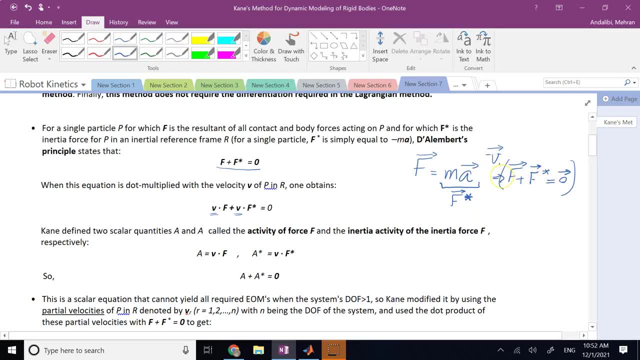 But then we are going to generalize it to include the equation of motion for an entire system. So it says V dot F plus V dot F star is equal to zero. And you know from my lectures on dynamics, or probably your physics, that V dot F is what. 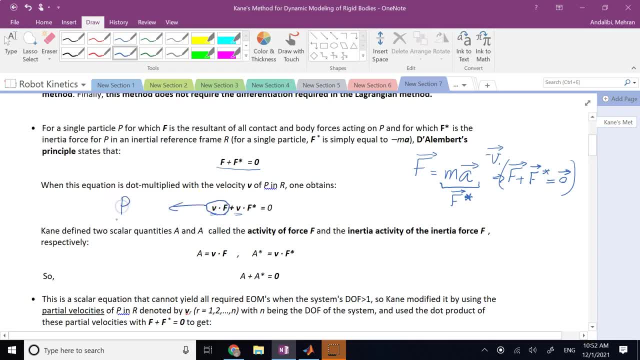 Actually that's the definition of power P right. Power P is V, dot F or dw over dt. Right, because dw is F, dot, dr and over dt. correct. This dr over dt becomes V. So that's the definition of power: V, dot, F. 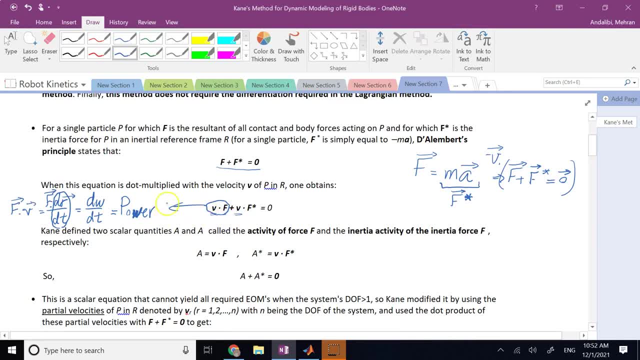 So it says the power injected into the system through the external forces and torques is equal to the power that the system has due to its acceleration or due to the inertial acceleration terms or inertial forces. So this is like power in equals power out, or power in plus power out equals zero. 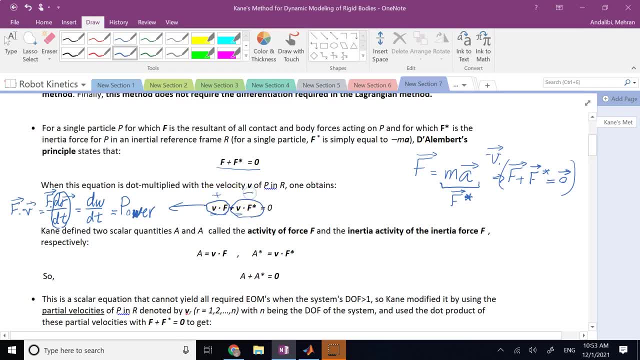 if for one of them you can see they're positive and for the other one you can see they're negative. So it says the power that all of these forces are injecting into the system is used in the system to give it acceleration And velocity. 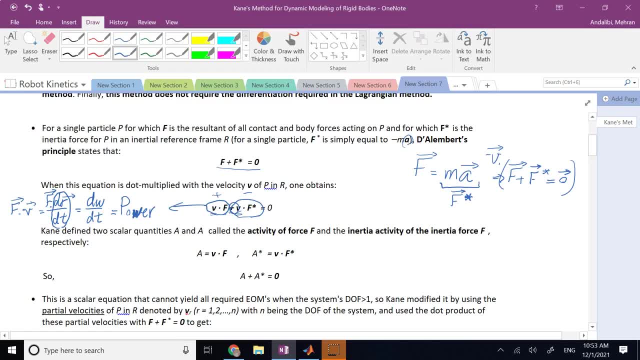 Or just one of them, really acceleration, because velocity is an aftermath of acceleration Chain. instead of defining V dot F as power, call this term activity. So it says: A, which is V dot F, is activity of the external force, F, and A star, which is V dot F. star, is the activity of inertial forces. 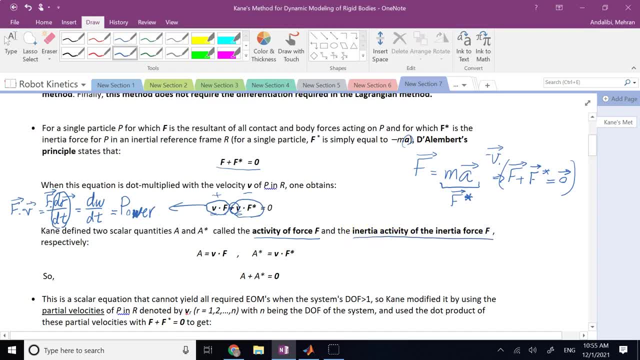 Or you can call it Inertial activity of the inertial force F, F star actually here. Okay, so it says now activity plus inertial activity is equal to zero. Again, that's the same thing, Just you're calling it some new term. 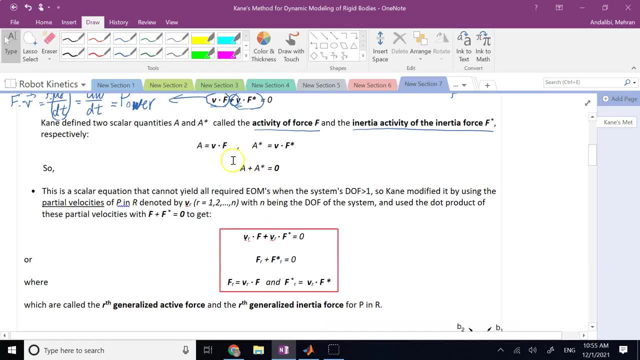 Good. Now what's the problem here? Well, the problem is: this is very good. This is an excellent idea. if you want to describe The equation of motion for one particle right with one degree of freedom, that's absolutely fine. 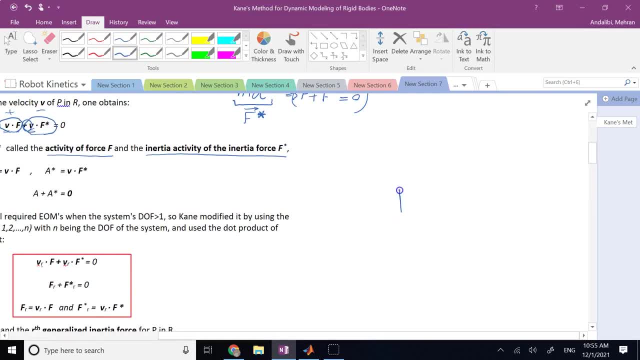 Because if I have a single particle here, let's say moving on a surface right, and I have this external force F, and I have the friction here. let's say FK equals mu K times N, And you know I also have N and MG. 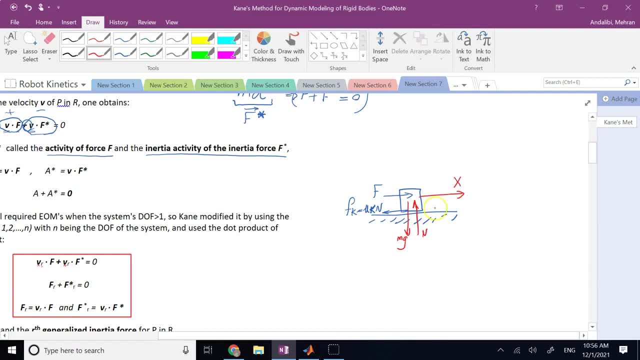 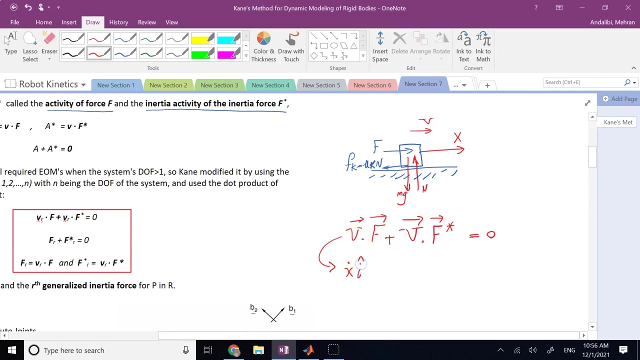 And this plug is only moving in the X direction with position X and or velocity V. If I say F dot V or V dot F Plus V dot F, star Is equal to zero V. here is X dot Times, I F. here can be all of the forces. 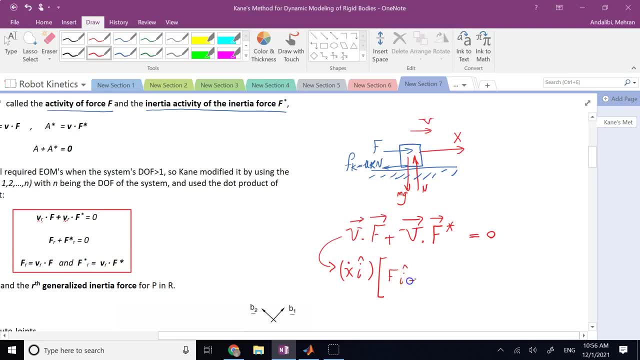 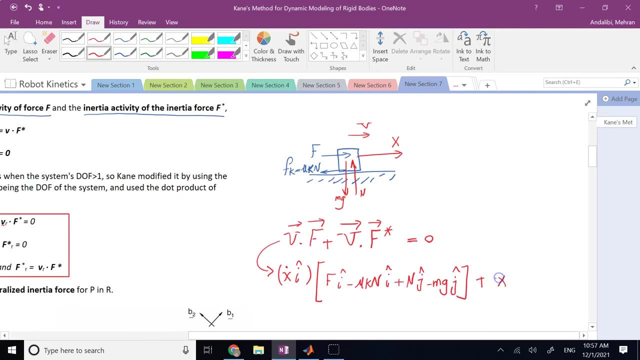 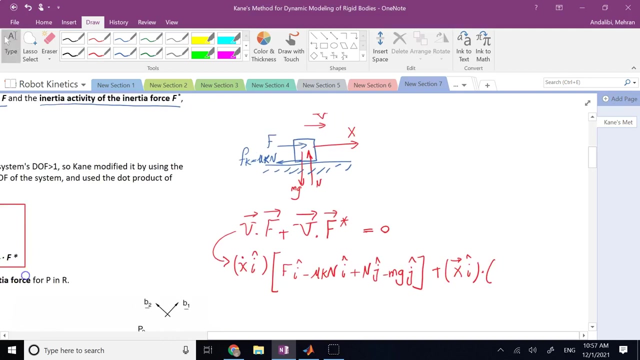 Which is the capital: F times I Minus mu K N times I, Then plus N times J And then minus MG times J And then plus again X dot. I dot the F star, which in this case, in general, can be what? 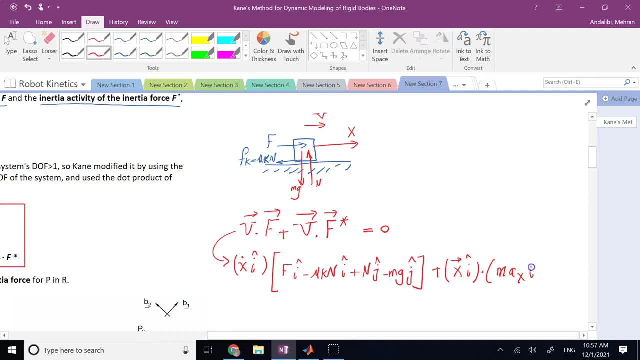 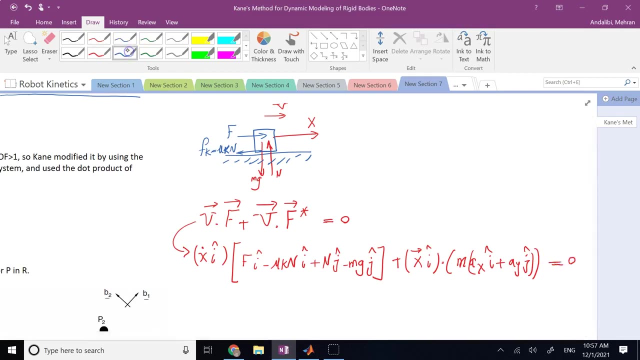 M times AXI, plus AYJ, The total acceleration of the block. This is equal to zero. And the thing is, when you do dot product, I dot I is one, but I dot J is zero. So all you will get down here is going to be what. 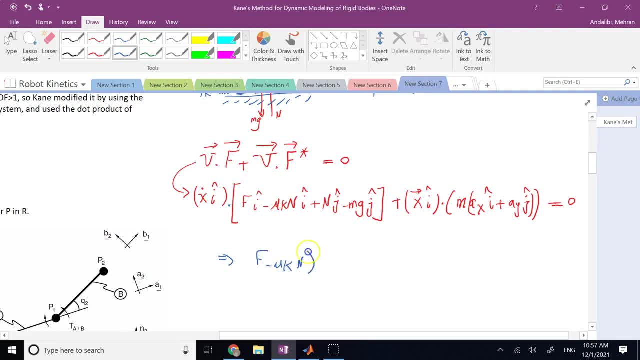 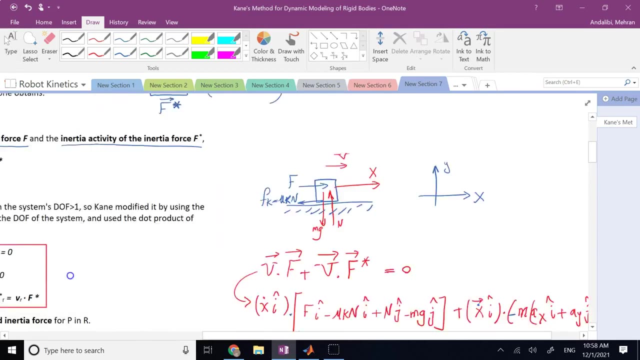 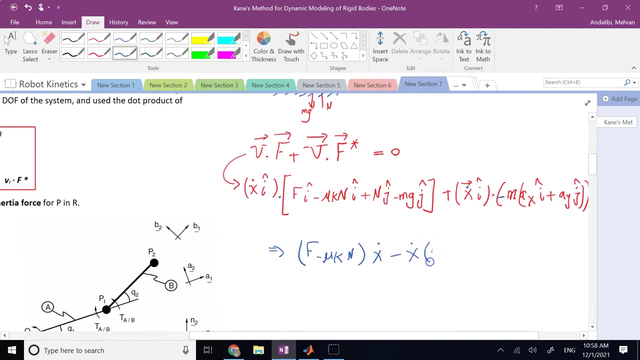 It's going to be F minus mu K, N. the whole thing times X dot. And then here it is going to be. This inertial term has a negative right. It's negative acceleration, negative M times A. So it's going to be negative X dot times M AX. 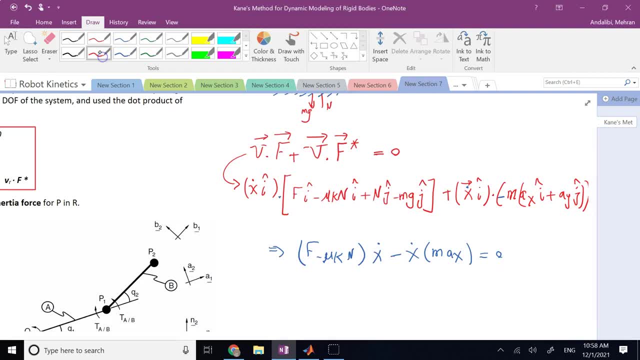 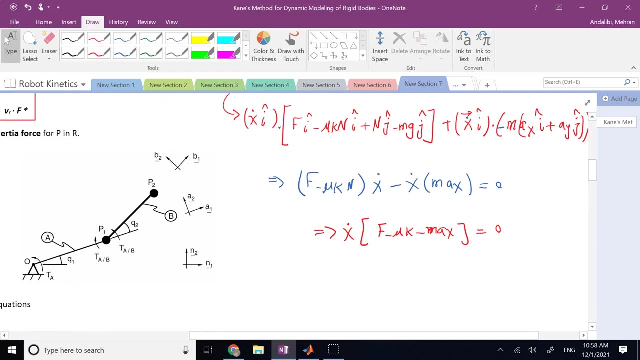 Is equal to zero, And here, if you factor out X dot Is going to be F minus mu, K minus M, AX Is equal to zero, And here, if you factor out X dot Is equal to zero. X dot cannot be zero because the system does move. 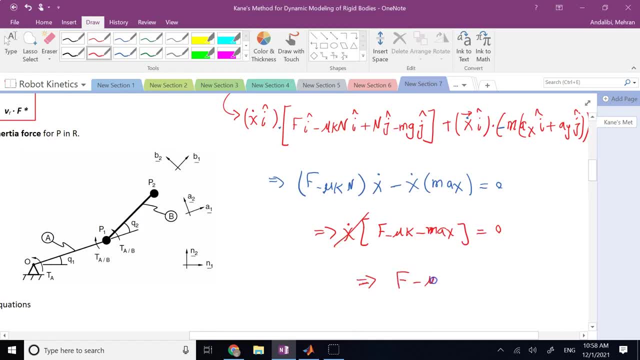 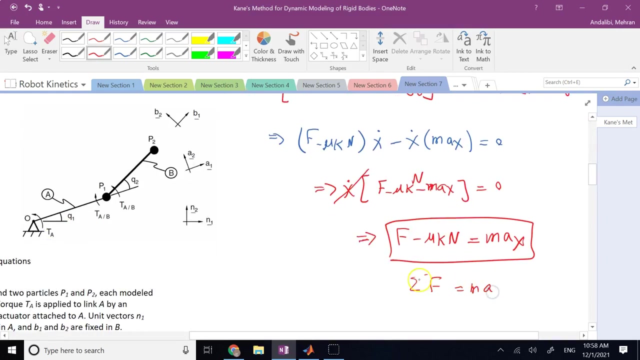 So that means only F minus mu K. N has to be equal to M AX. This is mu K times N, And that is of course the same as the equation of Newton. And you might say: well, why couldn't I directly say some F equal M A, and the life would be a lot easier, right. Some F in the X, And you might say: well, why couldn't I directly say some F equal M AX? And you might say: well, why couldn't I directly say some F equal M AX? And you might say: well, why couldn't I directly say some F equal M AX? 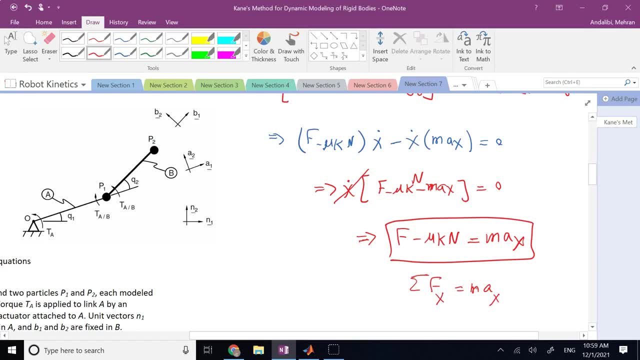 And that would be it. You're right. By the way you know, this N is equal to MG. in this case It is For a single degree of freedom system, or maybe sometimes even two, but most of the time one For one degree of freedom. the Newton method is extremely faster and easier than Lagrangian or Kaine. 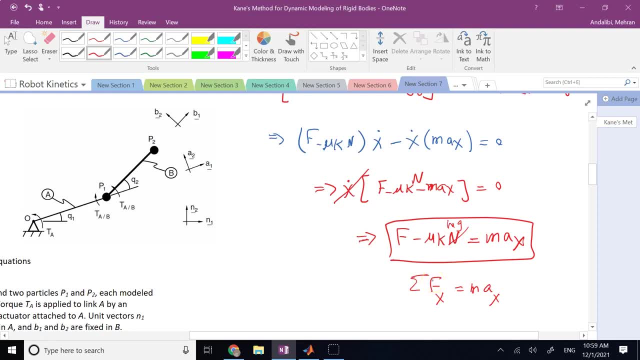 The problem comes when you go to higher degrees of freedom. The Newton Newton is not as easy to extend to higher degrees of freedom without including a ton of reaction forces, And especially when the constraint comes in. Lagrangian and Kaine, on the other hand, are a lot better to handle more degrees of freedom. 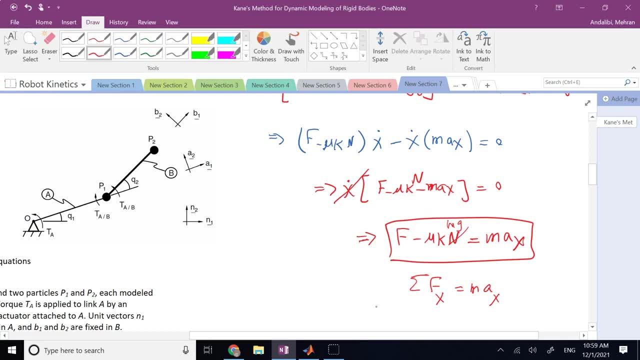 And Kaine is even better when it comes to constraints, Right, So, although one of them might be a lot better in the lower degree of freedom, but when they go up in the degrees of freedom and constraint, definitely Newton, Newton is not as easy to extend to higher degrees of freedom. 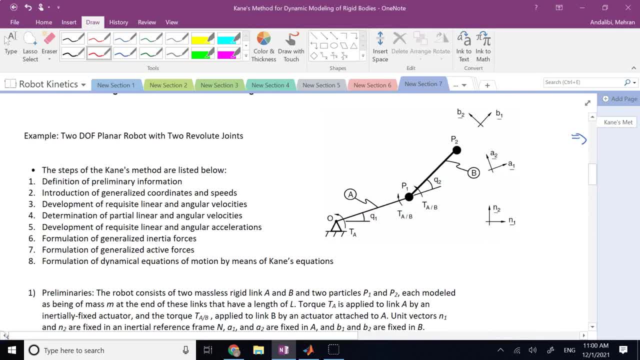 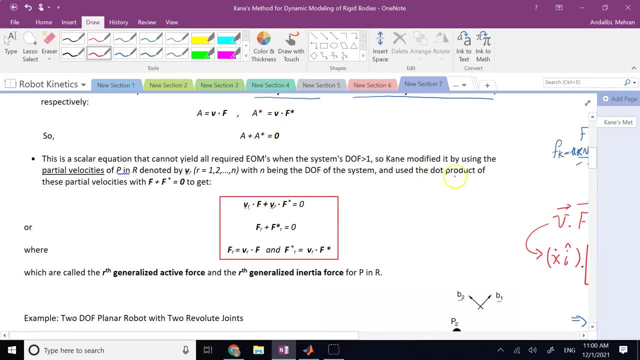 That's why the Newton method falls behind. Okay, So That's amazing, Right, If it can give us everything that it promised- and it will. The problem is this: information included in this equation is not enough when the degree of freedom go beyond one. 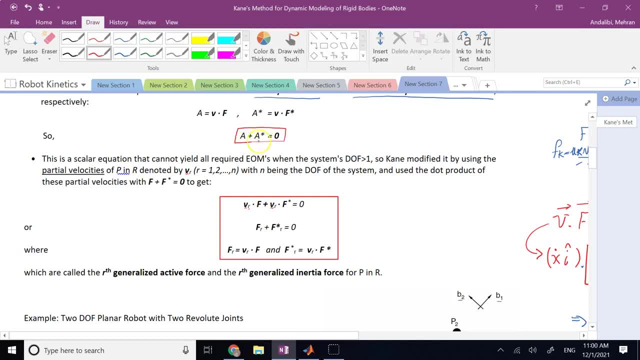 Why? Because this equation is actually a scalar equation. You know, A is the standard And this is the standard, And this is the standard same as power, as i said, and power is a scalar. so when you have one degree of freedom, it's. 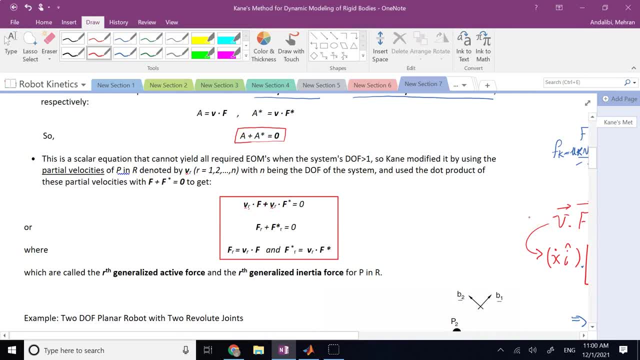 absolutely fine. but when you go more than one degree of freedom, this v in general, this vector v and this vector f or f, star the way that they are written. they cannot give us enough the equations of motion, like when the system has four degrees of freedom. this guy. 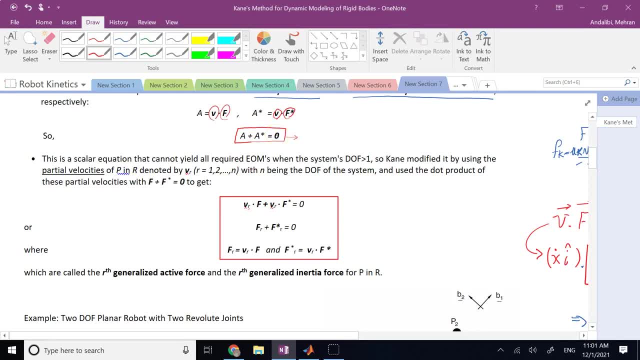 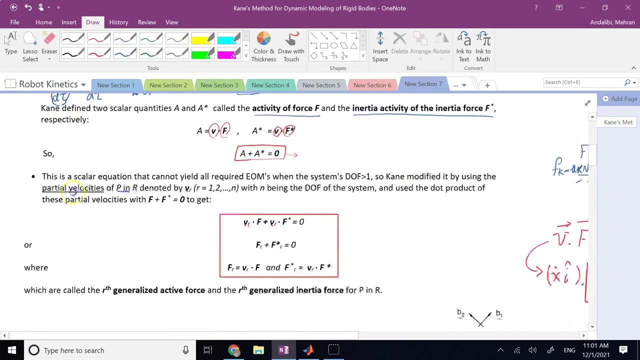 still will give us one degree of freedom, one equation, not four. so kane has to reformulate this to be able to apply to basically more than one degree of freedom. and what he did was, instead of dot product of v with f on both sides of this equation, he dot producted. 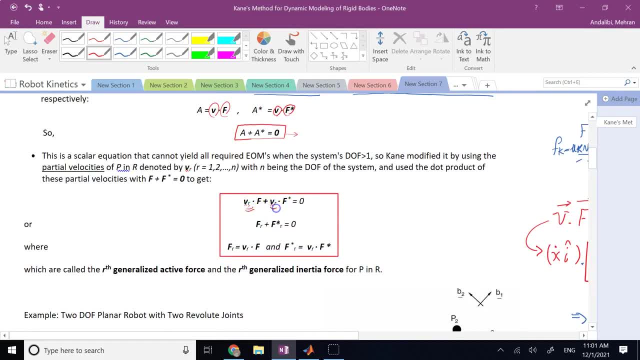 partial components of v, partial velocities, vr, vr, dot, f, where r here is a variable that can change from one to n and n is the degrees of freedom. so instead of multiplying dot, multiply the whole vector v by f. each time he only multiplied a partial, a portion of velocity of v by f, and that allowed him to acquire- because this r goes from 1. 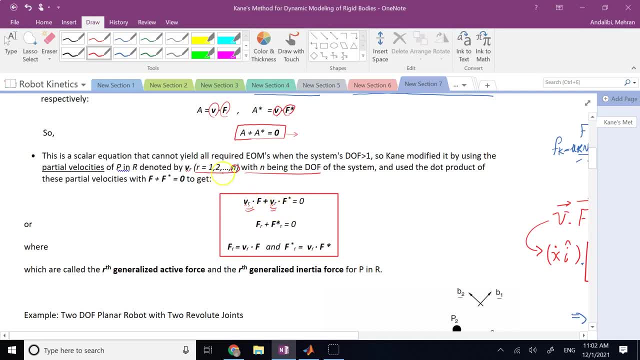 to n this equation. when you expand it, it's going to give you n scalar equations and you have n degrees of freedom. so now you are going to be fine, okay, so definitely, this new method can- uh- oh, that r should actually be there- this, uh new formulation, as long as we 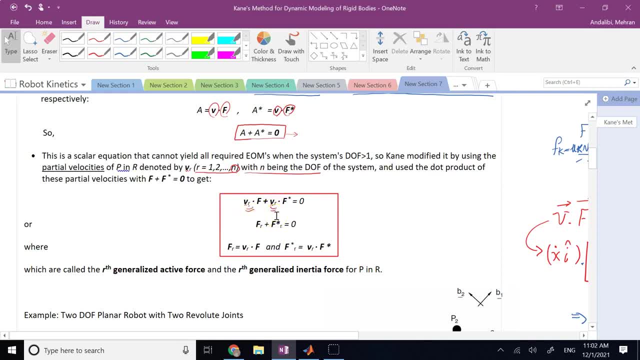 know what vr is can give us enough equations for enough degrees of freedom. so uh, first a terminology, this vr dot f or vr dot f star, which kane showed by fr or f star r. they are called the rth generalized active force or the rth generalized inertial force. 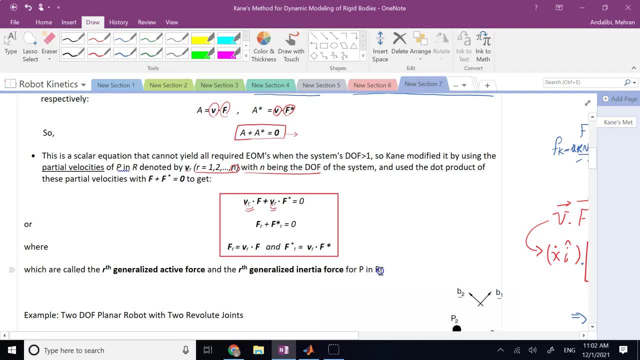 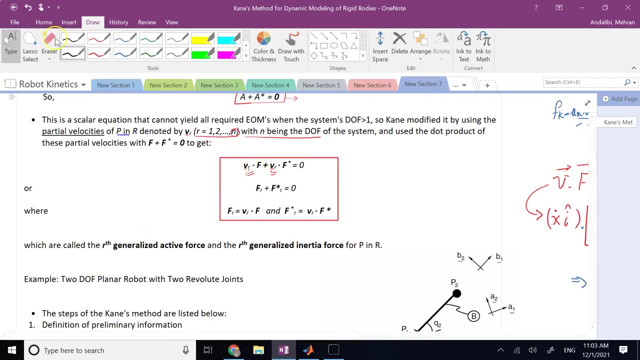 for the particle or the system in the space, in the space, in the tasker space, really. so please pay attention to the fact that, first of all, instead of the velocity, we are using a portion of the velocity, a partial velocity, and here i also call these terms. 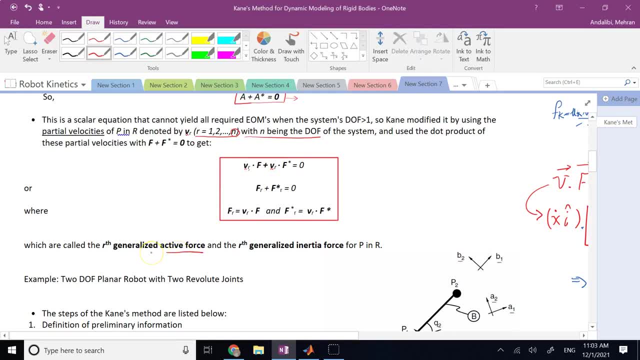 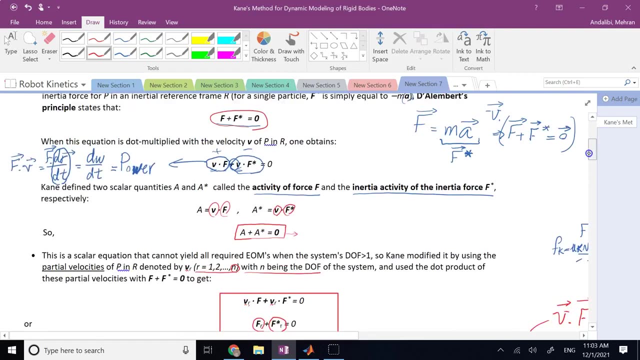 active force. i don't call them activity anymore, i call them active force. why active force? so it seems like this fr and fr star are now of type force instead of of type power that they used to be up there. why we'll see, because the definition of vr is actually not. 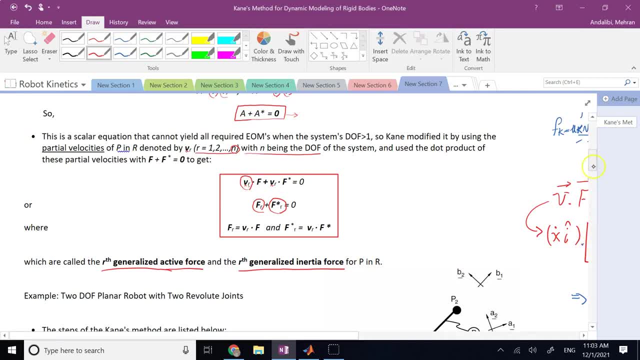 real velocity, it's just kind of like a direction of velocity it doesn't have. this guy does not have the units of, let's say, meters per second. it has the unit of like one. so fr and fr star has the same unit as f and they are really forces. that's why we call them um generalized force or generalized. 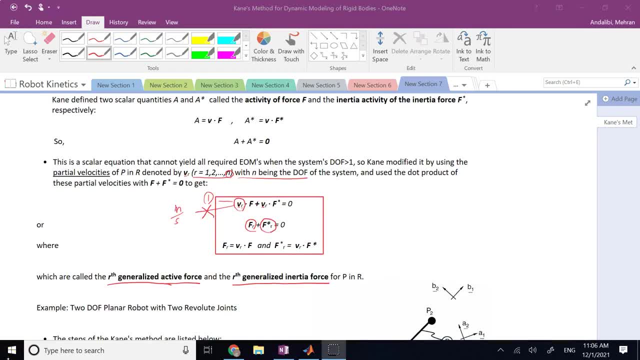 inertia force, and we also call them the rth generalized active force, because, um, they are really for the rth. uh, partial velocity, okay, we have r of these fr or fr stars, good. so now, uh, how do we define this? vrs? right, because that seems to be the major thing. 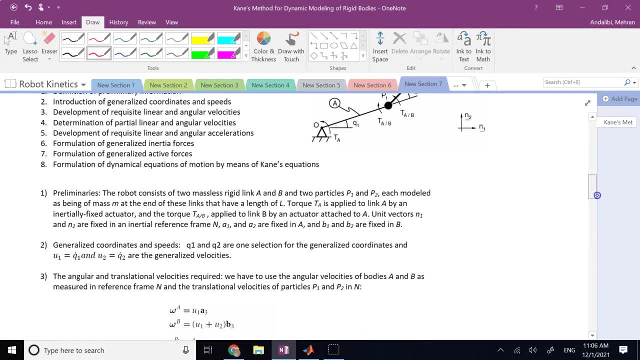 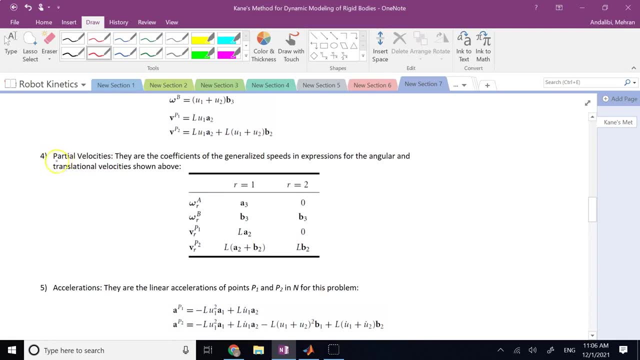 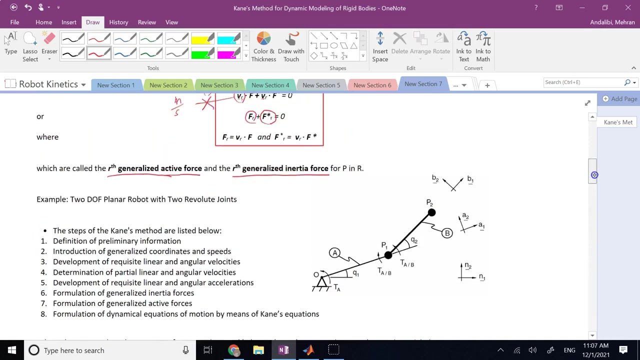 so let's go ahead and talk about the vrs. so, uh, these partial velocities, or vrs, are coefficients of the generalized uh speeds in the terms of angular and translational velocities. what does that even mean? so, in order to clarify that, i need to go through the steps of the kane method for you. 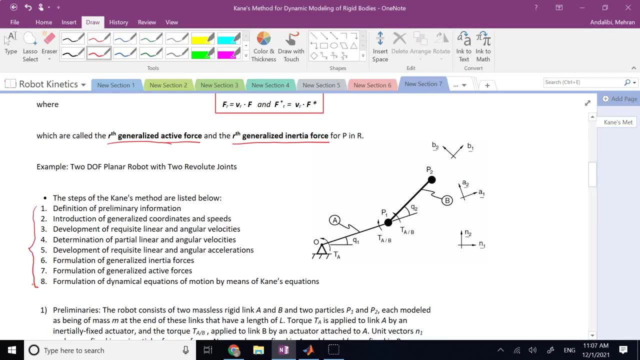 in general, this method has eight steps that you need to take for any system with any degrees of freedom, and i'm going to go through that and for that i'm going to use the two degree of freedom planar arm with revolute joints. right, because, as we said, this is like the simplest thing that we can drive our 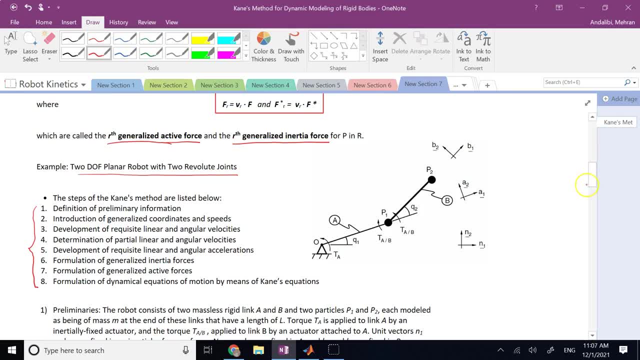 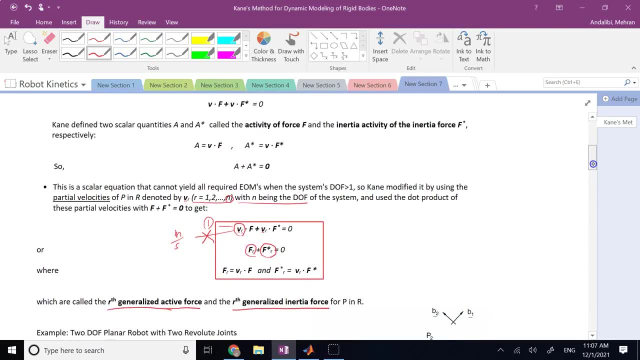 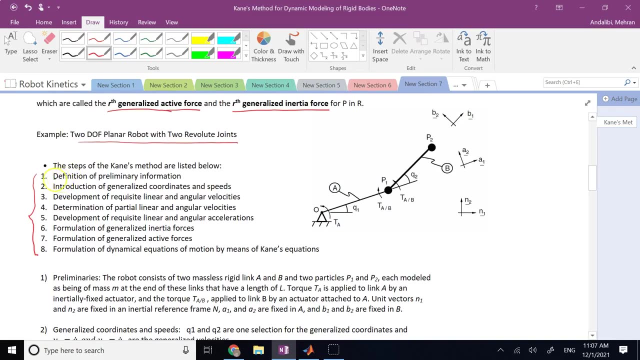 equations of motion for, or one of the simplest at least. so we apply the kane method on this robot and then i exactly clarify for you what is vr. so before we can do that, step number one of the method says: define the preliminary information. what does that mean? 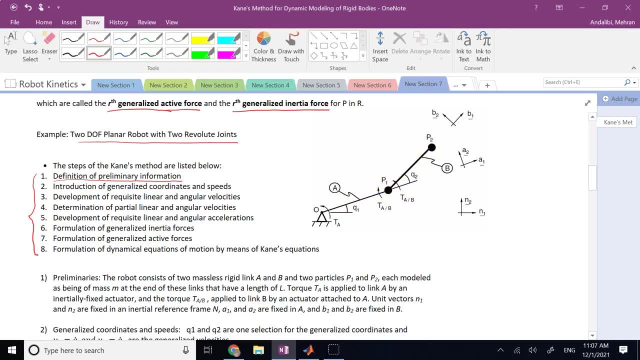 so if this is my two degree of freedom planar arm now, in this case there is a little bit difference with, uh, the two degree of freedom planar arm that i had previously. in this case, i assume that each member here has all of its mass concentrated at 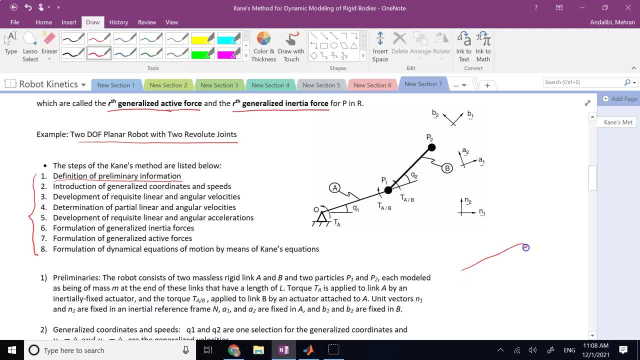 the end. so it's not like two uniform bars where the center of mass is in the middle or somewhere the middle. it's not like that. it's like two pendulas, basically one pendulum with no mass. all the mass is concentrated at the end, followed by another pendula pendulum and again the whole. 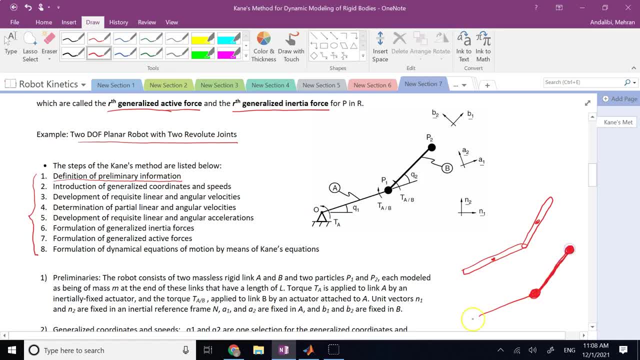 mass is concentrated at the end. so this is a little bit different than a regular two degree of freedom planner or man. you might say: well, what, if i want to really use this one, i'll show you. so we go with this, uh, this example, because this is a little bit actually easier than this one. 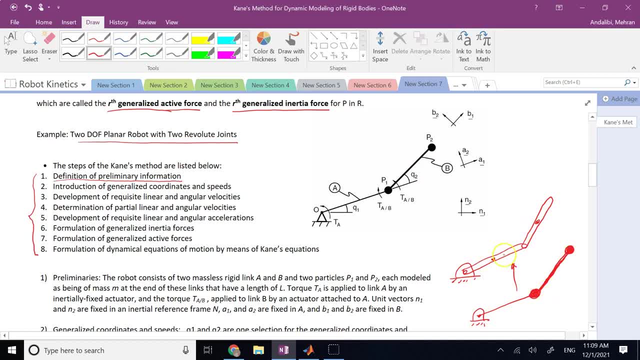 to describe the cane method, if you want, then we'll talk about how to go about this. uniform mass distributions. so here we're going to focus on this example and then what are the preliminaries? so first, describe the geometry we just did. we said this is like two pendulas. 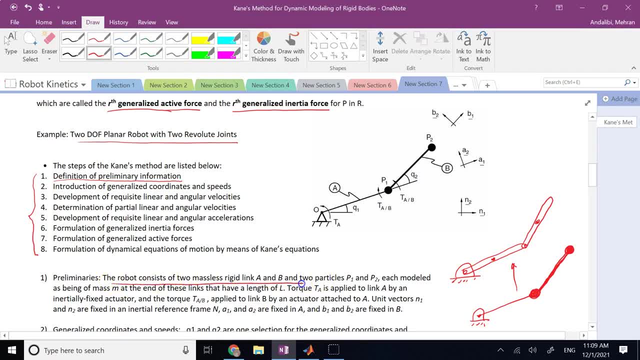 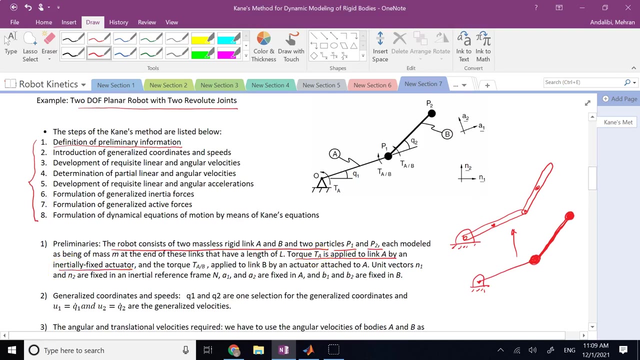 right massless length and all the masses are concentrated at those two particles, two endpoints, which we call them p1 and p2. the torque ta is applied to link a okay and it is measured from their inertial frame, or it is applied by an inertially fixed actuator. so the motor that you 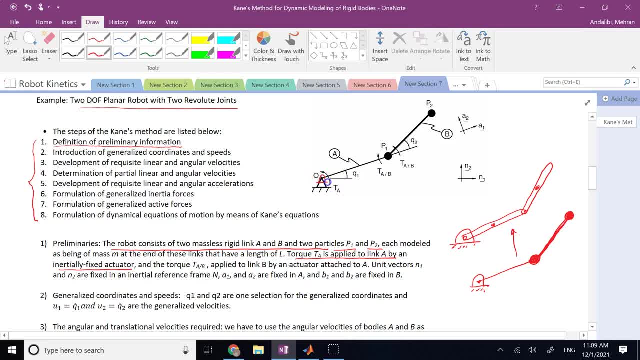 have here the motor that you have here to apply the torque ta, the bottom of that motor is attached to the ground. on the other hand, the torque that you apply to the second link tab, that one, is coming from a motor that the bottom of the motor really is attached to this. 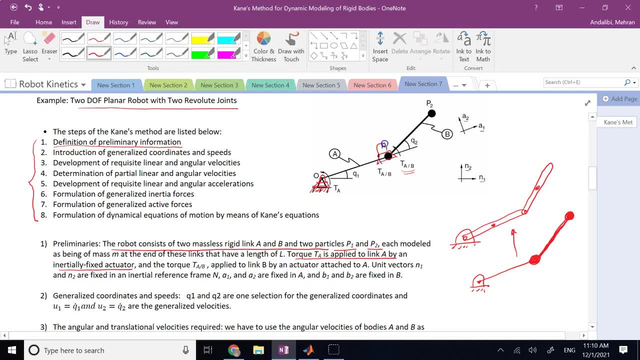 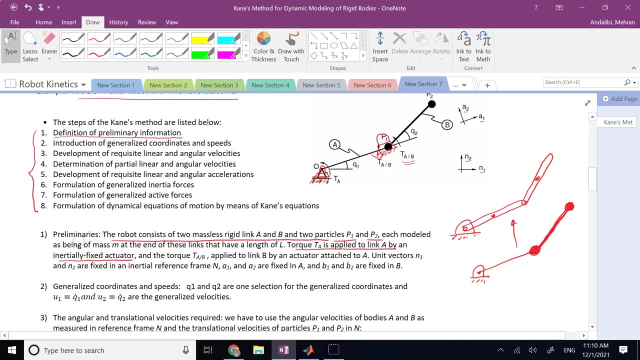 link a or object a. so if you have this motor here, this motor is rigidly attached, as i said, to block a. it's a relative, basically, connection, it's not inertial connection or connection to a ridge, to another rigid body which itself is moving. we are also going to use 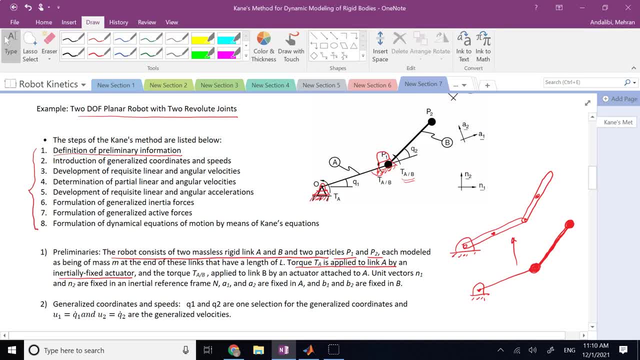 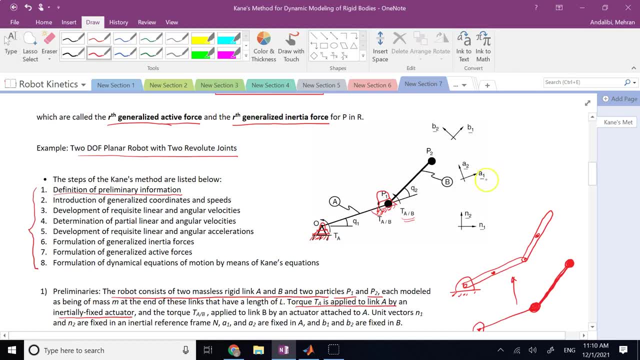 three sets of units, vectors or three sets of frames, just like what we did in the ds convention: frame a including a1, a2 and a3. here, a3 is out of the board, toward us. they are rigidly attached to object a, the first link frame, b1, b2, b3- again b3- out of the board. they are rigidly attached to block b. 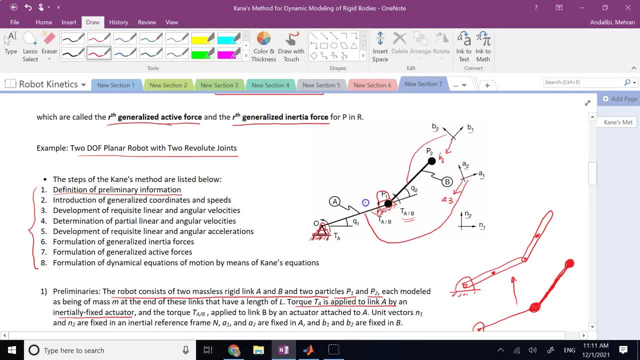 and then we have the inertial frame n1, n2 and n3 and these guys are really the ground, right, they are attached to the ground, they are inertial frame. so, just like the dh method, i use very similar to that or identical to that- a1, a2, a3, b1, b2, b3 and n1, n2, n3, and i have explained all of them. 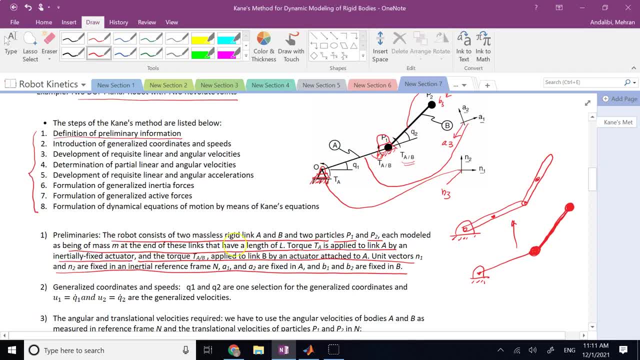 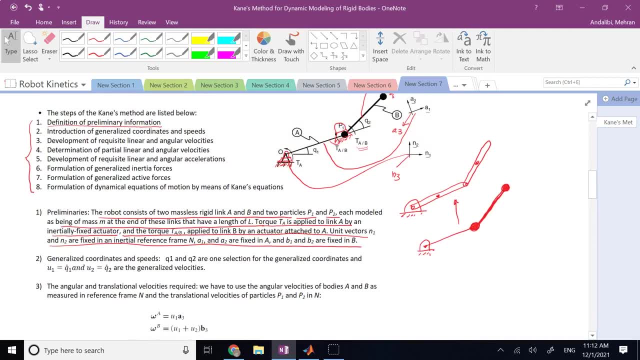 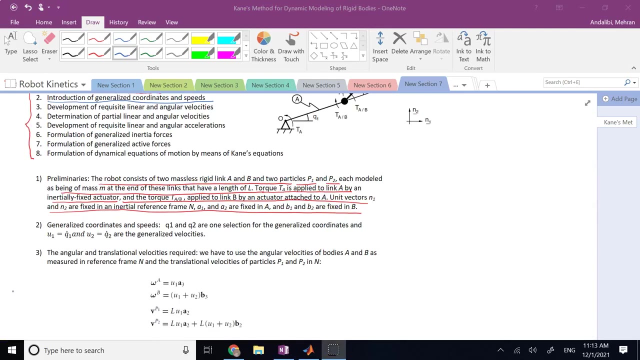 so here we describe the geometry of the system, the coordinate frame that we use, and these are called the preliminaries. that's step number one. step number two is: what generalized coordinates and what generalized speeds are we going to use? so here we distinguish between speed and velocity. okay, here, when we say generalized coordinate and 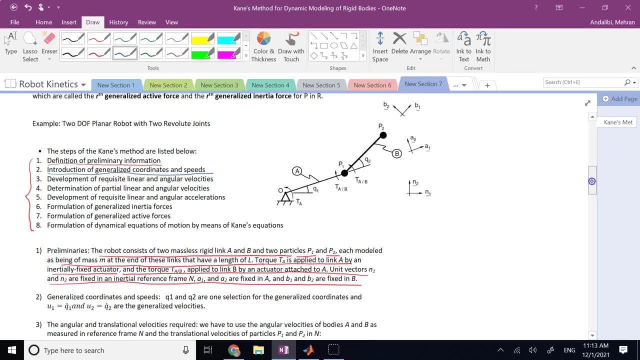 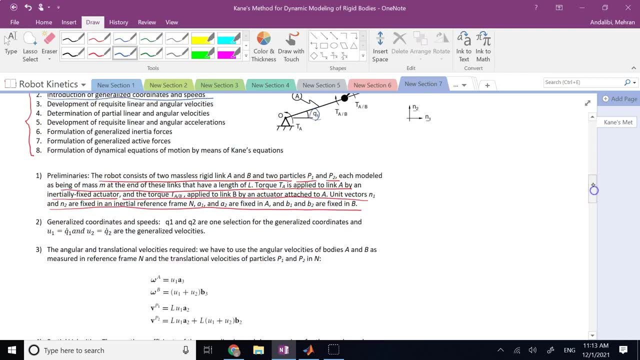 generalize speed. the generalized coordinate, just like lagrangian, that we use are q1 and q2, the two that best describe the degrees of freedom in the system, and generalized speeds are, like the time, derivative of these. so we use q1- dot and q2- dot. 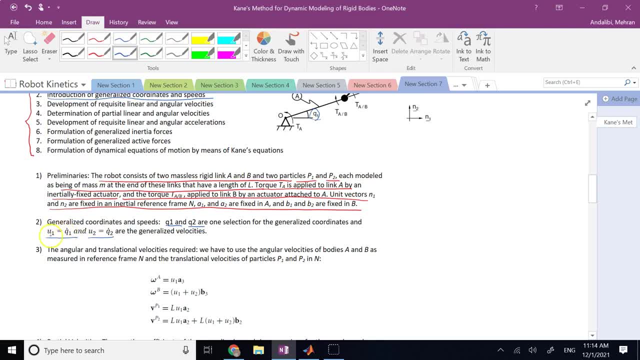 and to avoid showing dot all the time, we basically use a notation: u1 and u2. so the time derivative of this generalized coordinate is what we call generalized speeds, and we call them here u1 and u2, which are the same as q1 and q2 dots. now step number three is: 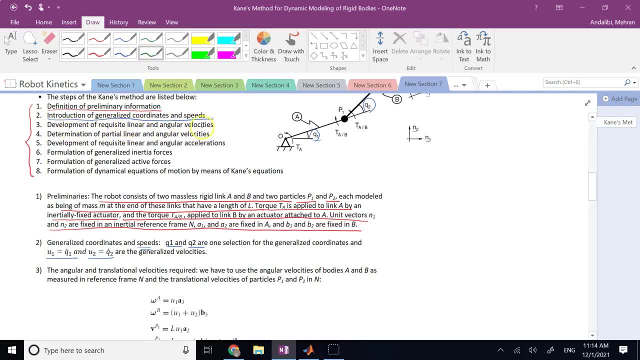 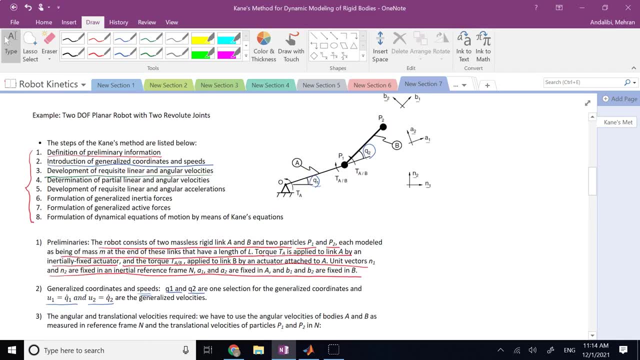 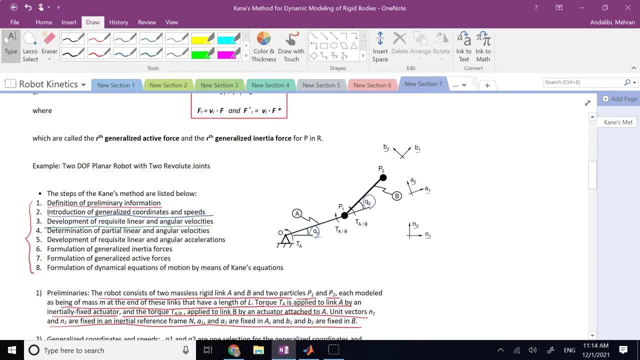 to develop the required or requisite linear and angular velocities. if we want to include the work or the, the power right, as we described it early, by anything in the system, including external forces, external torques and anything for that matter, what kind of linear and angular velocities do we need? 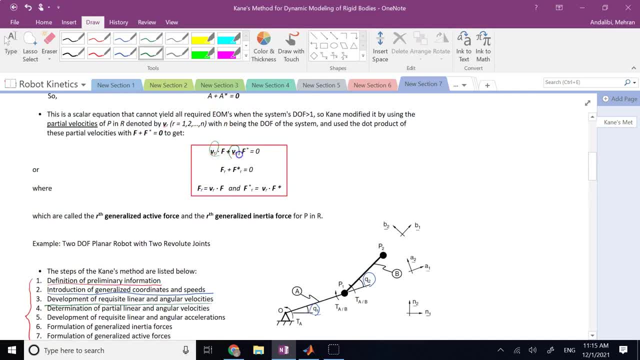 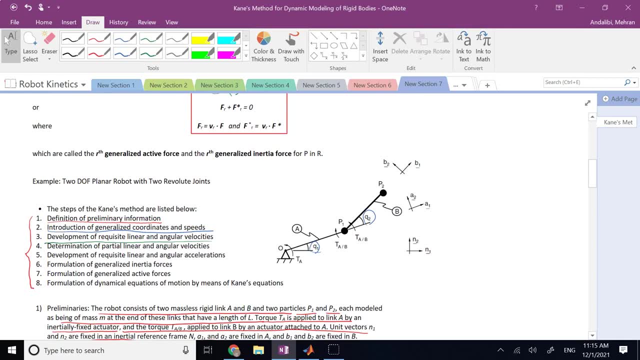 to include for the definitions of this vr. in other words, look at your system and see where is it that any external force or torque is applied and when those forces or torques are applied they are going to be the cause of what kind of motion they are going to be the 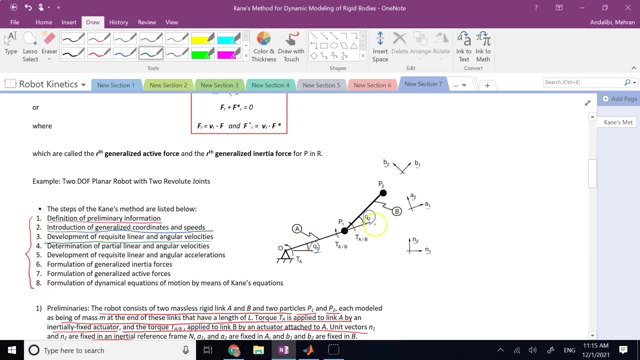 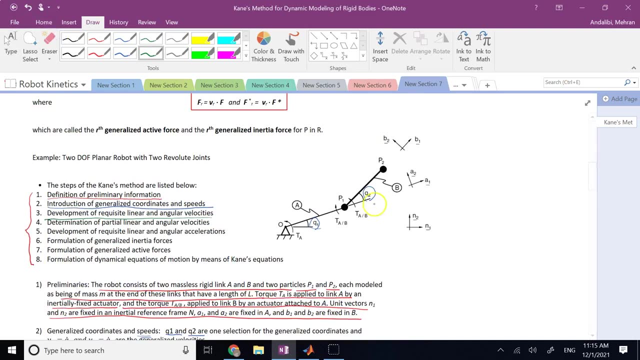 cause of a linear motion or the cause of what an angular motion, and whatever that is the effect of those external forces or torques, whatever the velocity is the direct result of those forces or torques, and so on. so the final thing we need to do is to include them here. so if i look at my system, 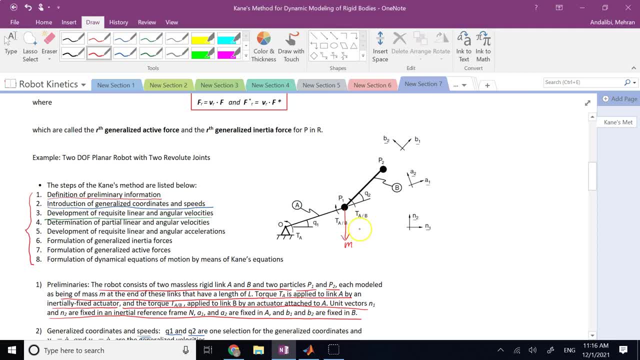 uh, what do i have? i have two gravity forces right, m1g and m2g. by the way, in this system we assume both of the blocks have the same mass, m. so i have mg here and i have mg. there are gravity forces. the end effector here is completely free to move, so there is no force here. 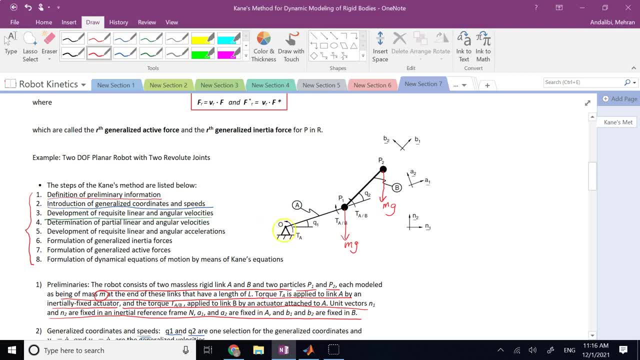 there are reaction forces from outside of the system at point o, so i can call them o y and o x and of course i also have these two torque terms. so there are the six terms if i want to draw the free body diagram of the entire system. 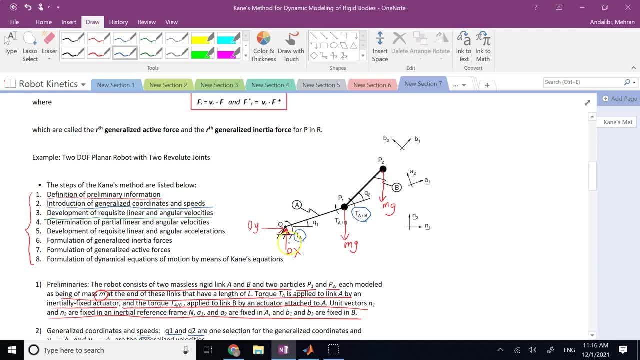 now out of the six, definitely ox and o y do not have the same forces because they are applied to points that do not move. so o x and o y do not cause any motion. so what, i can eliminate them from my list. they don't cause anything. what is the effect of t a? 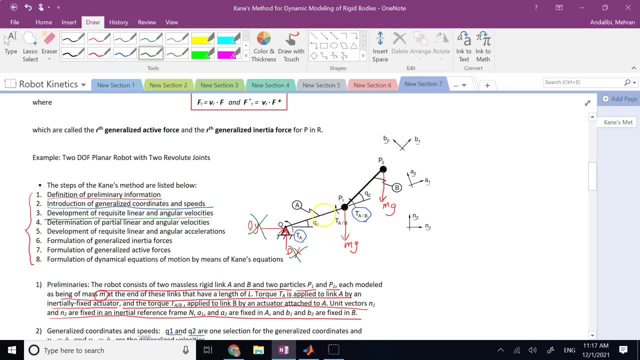 well, t a is to rotate link a. so if this link a is rotating and i call the angular velocity of link a omega a, then definitely i can eliminate them, because they are applied to points that do not move. so o x and o y do not cause any motion. so what? i can eliminate them from my list. they don't cause anything. what is the effect of t a? well, t a is to rotate link a. so if this link a is rotating and i call the angular velocity of link a omega a, then definitely o x and o y do not cause any motion. so what, i can eliminate them from my list. they don't cause anything. what is the effect of t a? well, t a is to rotate link a. so if this link a is rotating and i call the angular velocity of link a omega a, 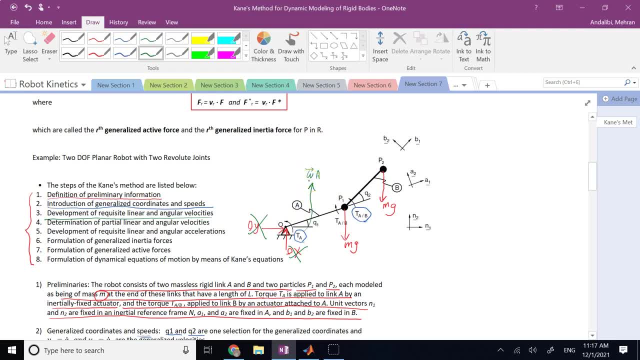 Definitely, omega A is one of the required angular velocities. The same thing for T of A with respect to B. The goal of this guy is to rotate link 2.. So if I call angular velocity of link 2 omega B, then omega B is one of the required things. 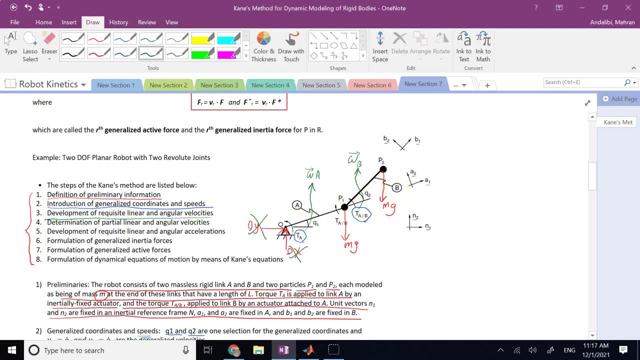 And you see, here I call link 1 and link 2, A and B, What else I have mg forces applied to these mass particles, P1 and P2.. And you know, definitely when you have a force applied to a particle that particle would get acceleration. 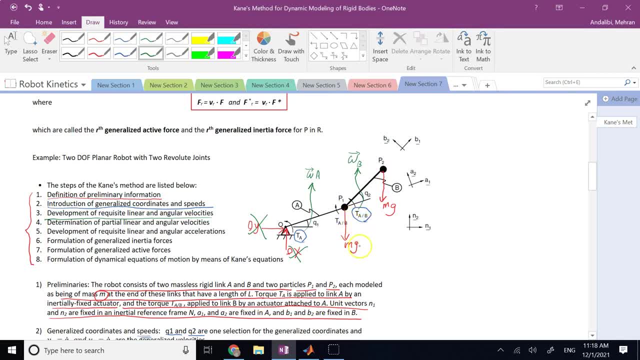 I mean linear acceleration, A, and then A causes some V. So the goal of this mg is to move particle P1.. So velocity of particle P1 is definitely something you want to consider. That's the effect of that mg. The same thing for this mg. 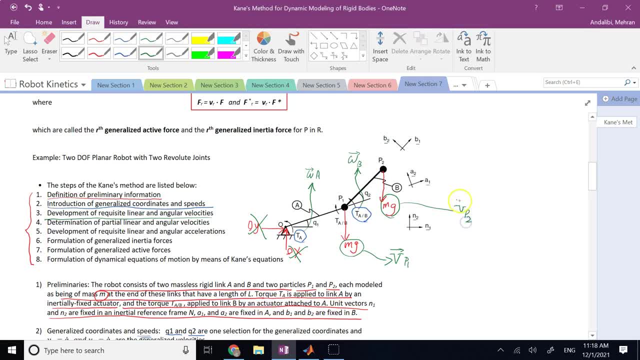 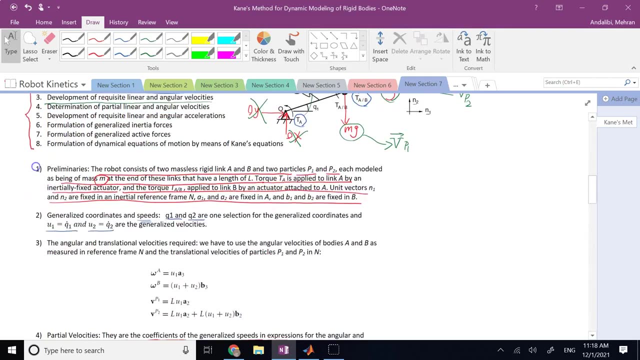 It should create Vp2.. So clearly you see your required linear and angular velocities of omega A, omega B, VpA and VpB, Because that's where those external forces and moments who cause any motion are in effect, And that's exactly what you see in step number 3.. 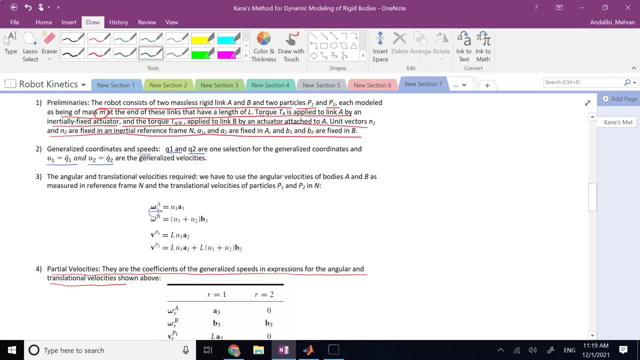 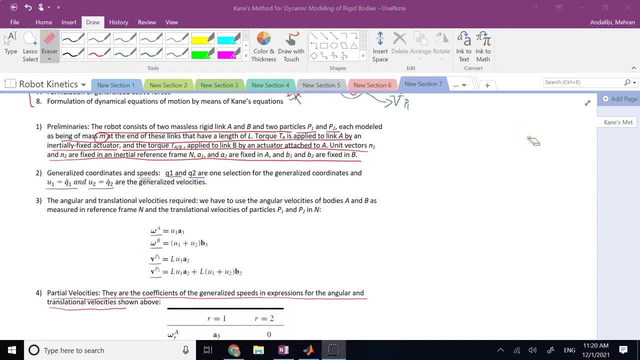 That we have to use omega, Omega of A, omega of B, VpA and Vp, Vp1 and Vp2.. And we also need to determine how much they are. So, since these are velocities, definitely their magnitude depends on what. 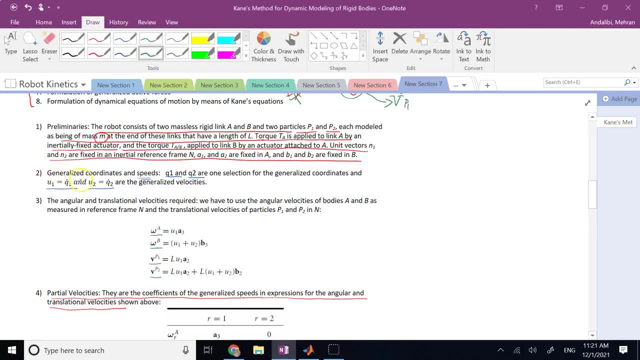 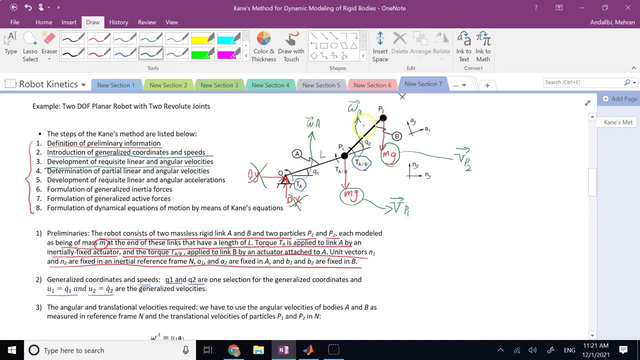 Depends on U1 and U2, the generalized speeds, as well as the geometry, which in this case is L. Remember, the length of each one of these members is L, So they depend on L and U1 and U2. And their direction should be described in one of these three coordinate frames that we have. 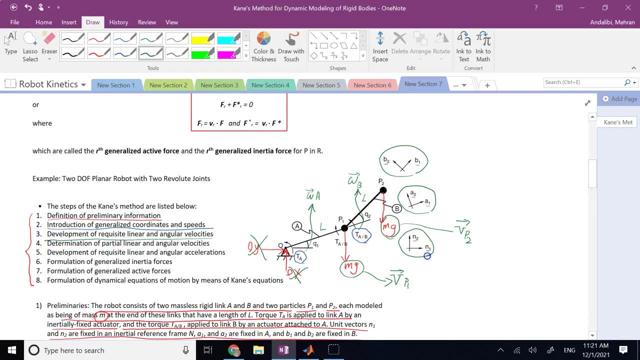 Either A1, A2, A3, B1, B2, B3 or N1, N2, N3.. Okay, So if I can describe them, that's all I need. So how can I do that Here? I can do it based on very simple rigid body kinematics. 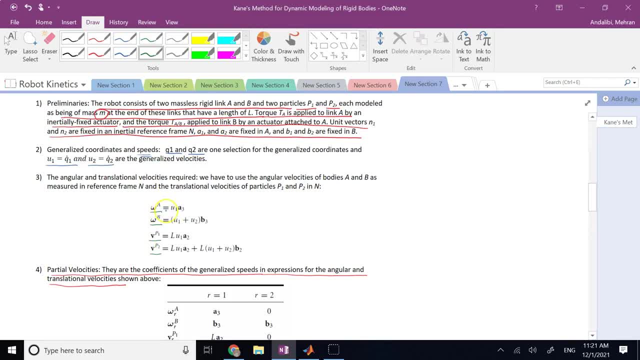 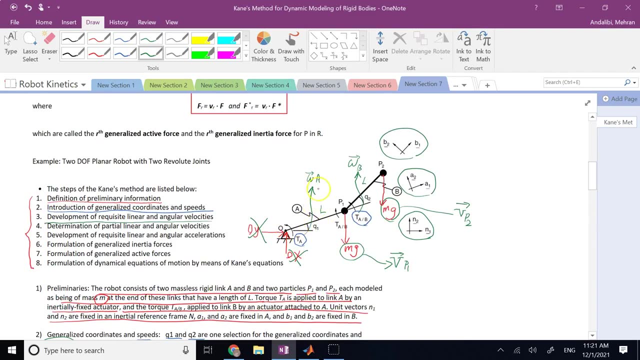 So omega of block A Or link A is definitely U1 times A3. Why Magnitude of it is U1? because definitely block A is rotating with angular velocity. Q1 dot. Correct. So Q1 dot is the same as omega A. 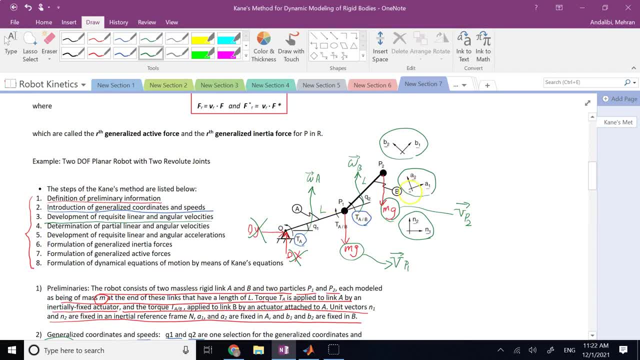 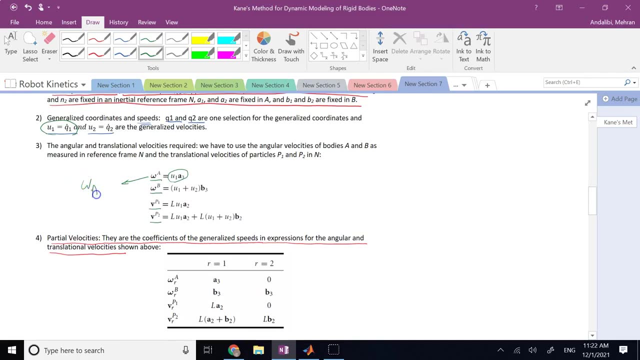 And the direction of it is about what axis? It's about A3.. Right, Because A is what is attached to this rigid body. So basically, what I'm calculating here Is omega of A written in A, Basically The omega of that rigid body measured in its own body attached frame. 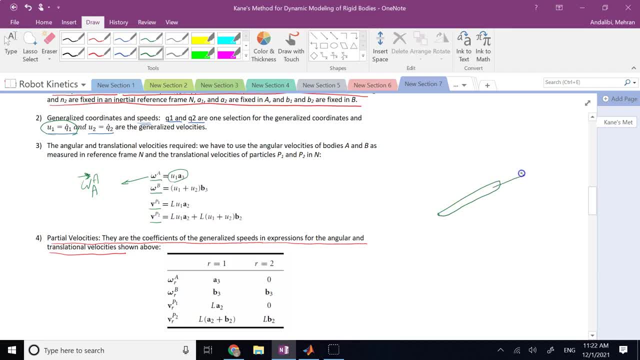 And since this rigid body has A1, A2, and A3 is out of the board And your rotation is about the axis: out of the board, Correct, Correct. So omega is going to be the magnitude of It times the direction of it. 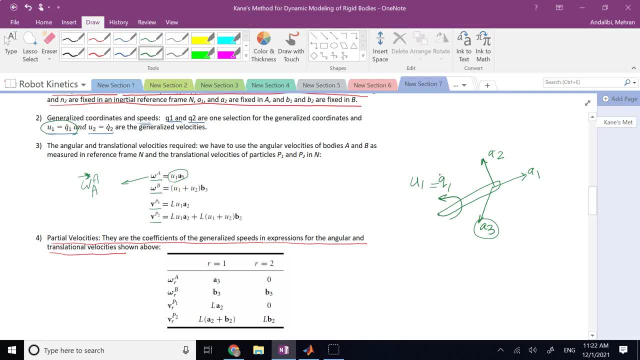 So U1 times A3 is very obvious. The same thing for link 2.. Link 2. The magnitude of the rotational velocity of it is U1 plus U2. Or Q1 dot plus Q2 dot. And again, since frame B is attached to second link, 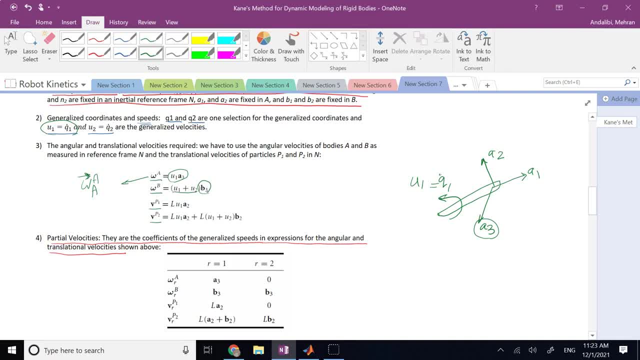 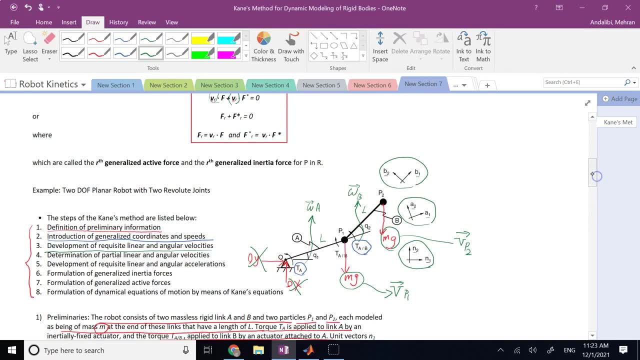 The axis normal to the plane, for it is going to be B3. So U1 plus U2 times B3 is omega B. And why is it that you add these two together? Because the angle Q2 is relative to member 1.. 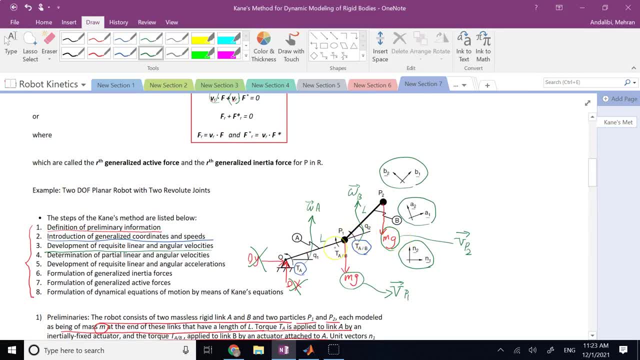 It's not relative to the inertial frame, So I have to add Q1 dots and Q2 dots together, Correct? So this is so far for the omegas, which were quite clear. Now let's talk about velocities of each one of these particles. 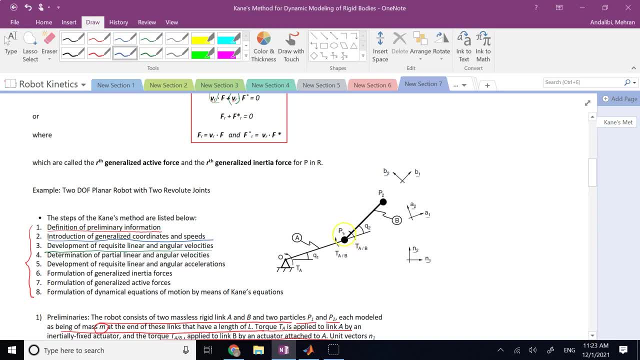 So first we need velocity of this particle, P1.. P1 does rotate about O And, as you can see, As you know, When a point is rotating about a fixed point, Velocity of it. V equals omega cross R, As you know. 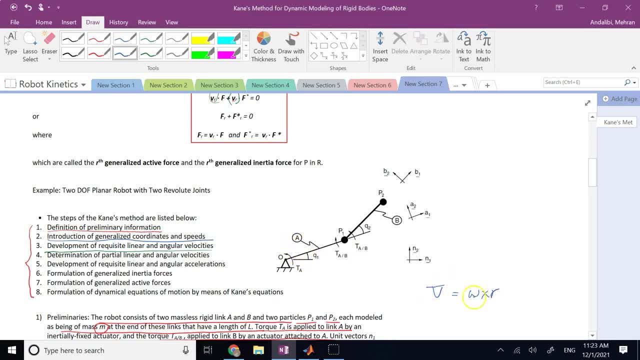 And omega here is U1 in the direction of A3. And R for it, in this case, is this vector. So this is going to be L in the direction of A1. And if you do so, What will you get? Well, you get U1 times L. 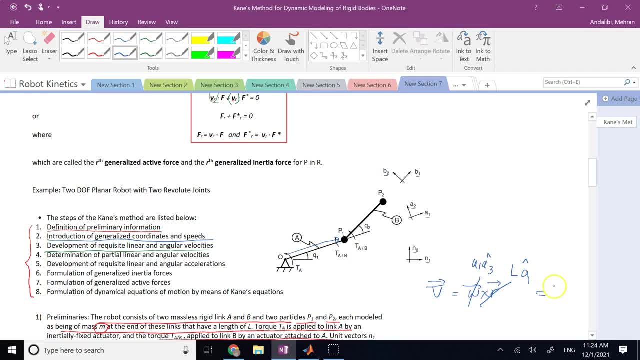 And then A3 cross A1 is going to be A2. So there's going to be LU1 in the direction of A2. Again, A2 comes from A3 cross A1. So LU1. Right, Which is LQ1 dot in the direction of A2.. 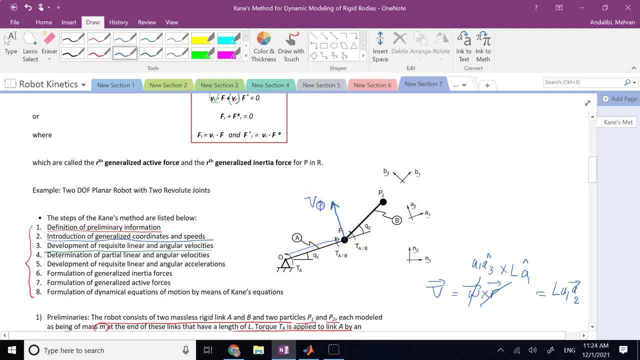 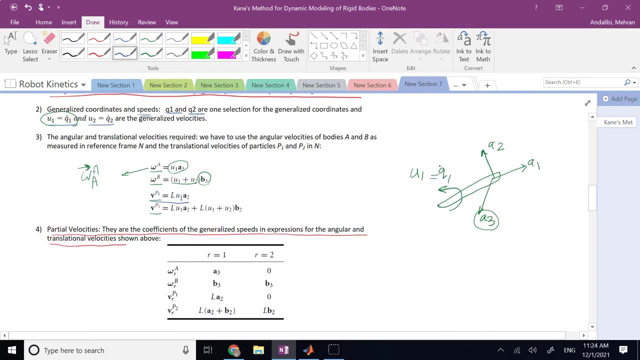 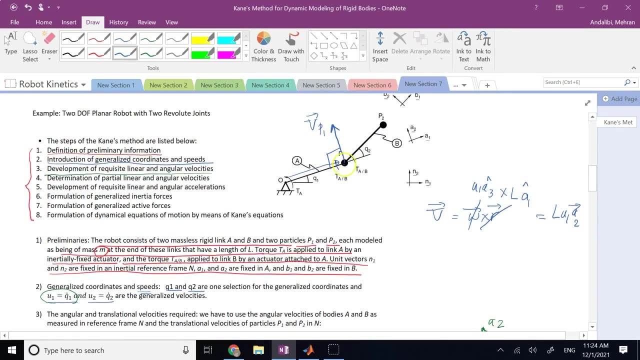 So this direction, This is going to be V of P1. Absolutely it is. You know that from dynamics And that's what you see here. And then we need V of P2.. And for that, Now that we have V of P1.. 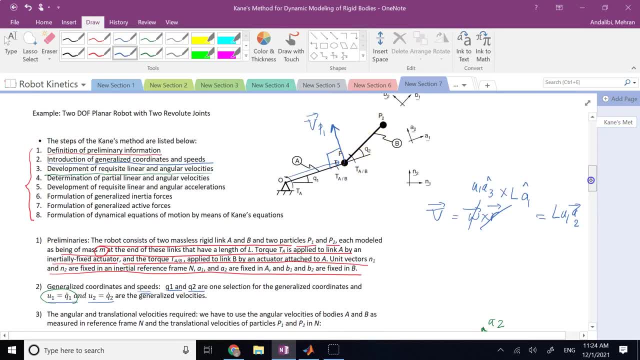 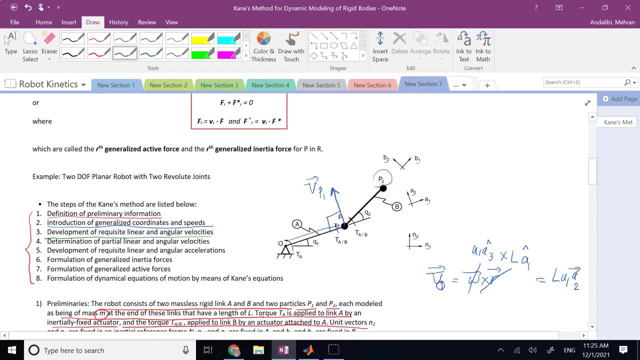 I go to rigid body. B And V of P2 can be found through V of P1 and omega of the rigid body. So V of P2 is going to be what It's going to be: V of P1.. Plus omega of this one. 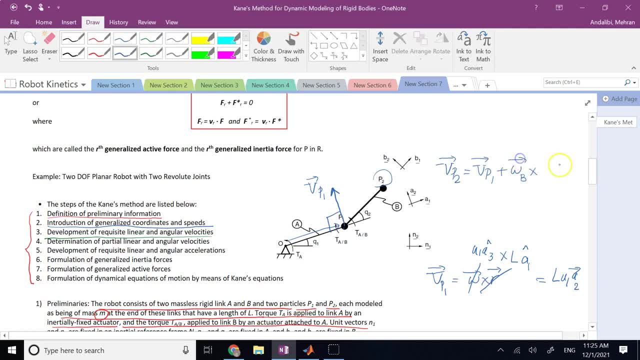 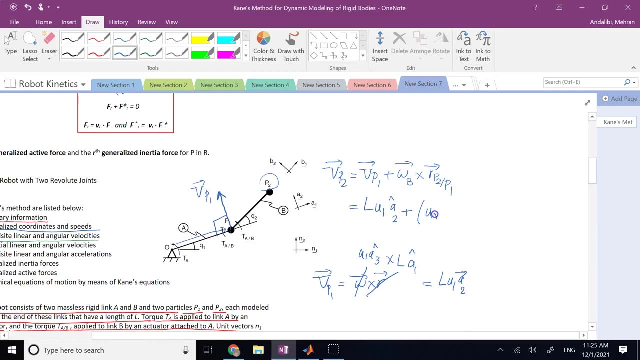 This rigid body Cross, the R between these two points. V of P1 is already LU1A2.. Omega of rigid body B, as we found it, Is U1 plus U2 times B3.. Cross, What is R? The R is this vector. 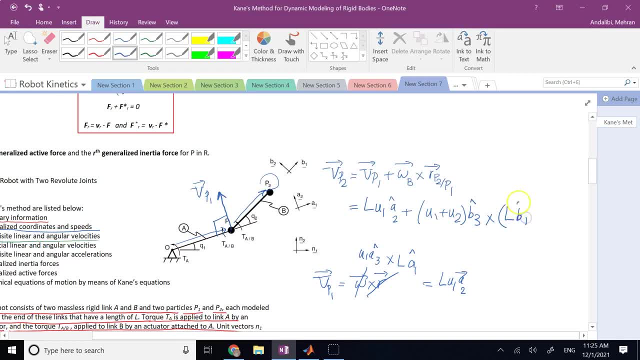 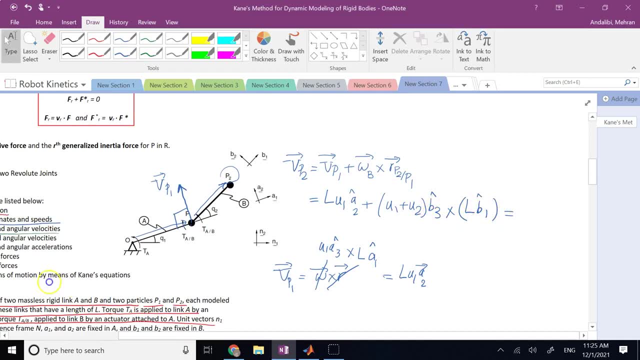 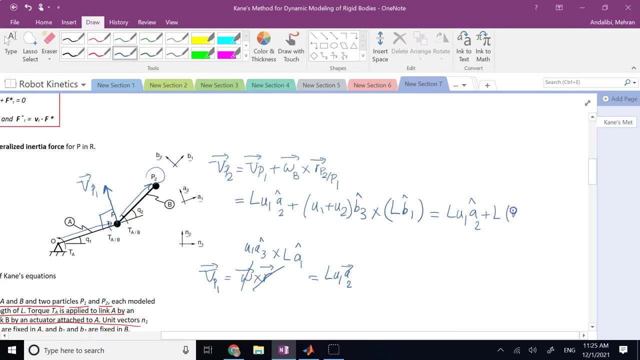 So there's also L in the direction of B1. So if we do that again, we have B3 cross B1. So that's going to be B2. And so you will get LU1A2 plus L times U1 plus U2.. 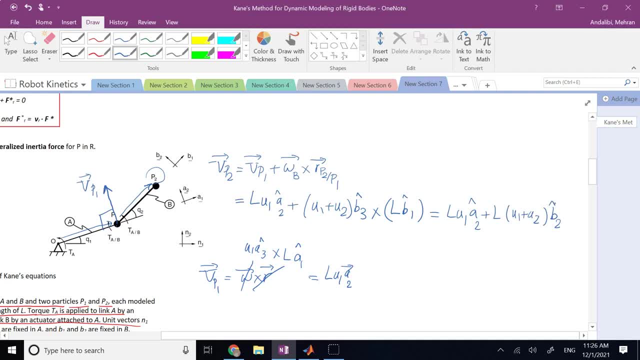 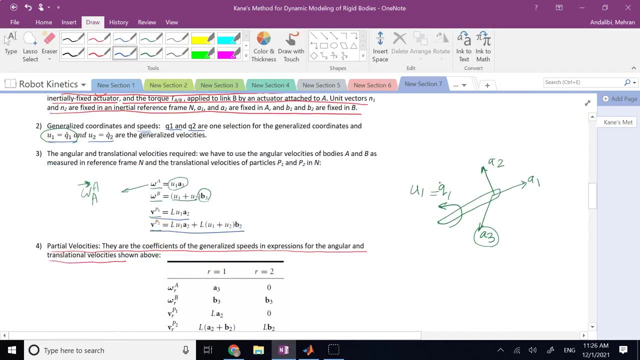 The whole thing times B2.. Right, So this guy is your velocity of a particle B, And exactly you can see. that's what you see here. So now I have determined The required linear and angular velocities of the system, Using these in the next step. 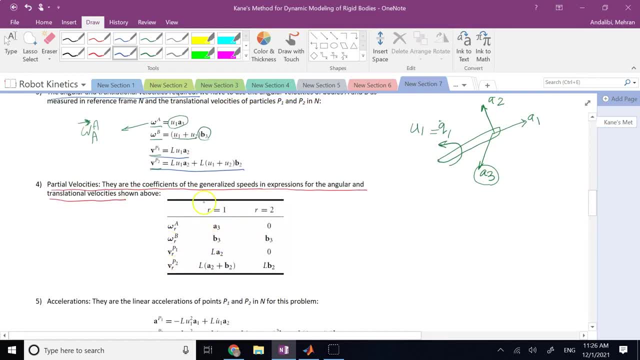 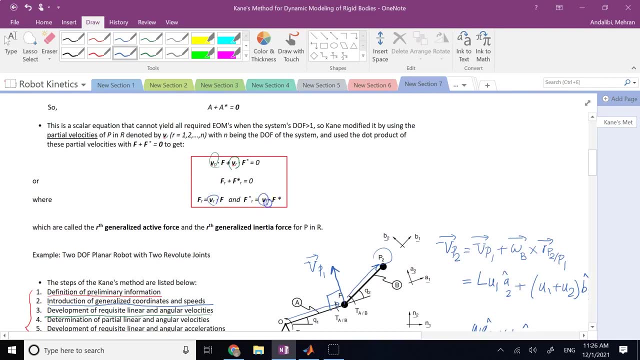 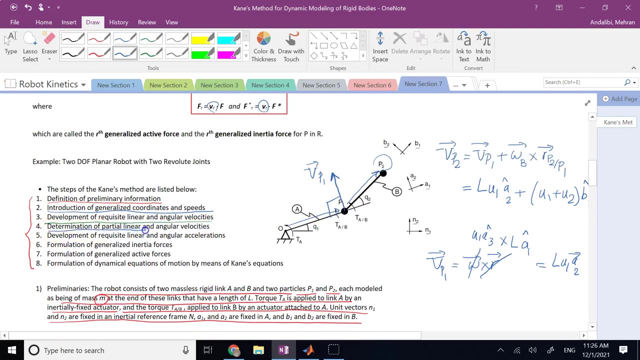 I can determine those partial velocities, Those VRs or omega Rs That I need to use in my formula. Okay, So that's a step number four, now Determining the partial linear and angular velocities, The VR or omega R terms. 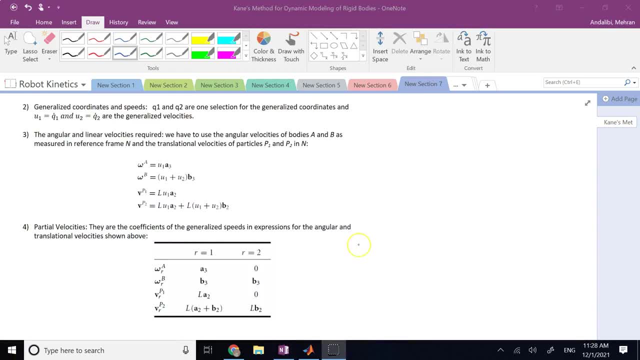 Okay, So let's go ahead and do that. This step is not hard at all. Once step three is done, Step four is no big deal Because These VRs and omega Rs, These guys, Are really the coefficients Of the generalized speeds. 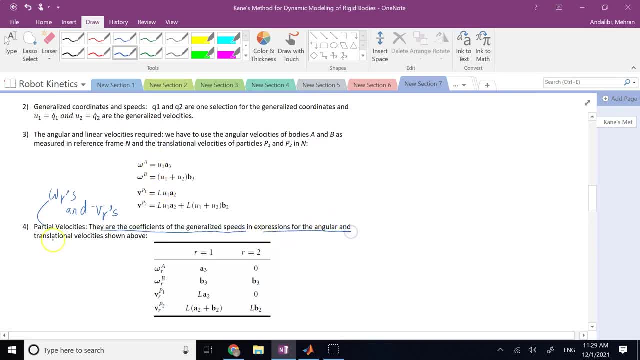 In the expressions for angular and linear velocities. So you form a table like this: On the left column You arrange all of these four terms: Omega A, Omega B, VP A, VP, VP1, VP2.. And you give a subscript R to each one. 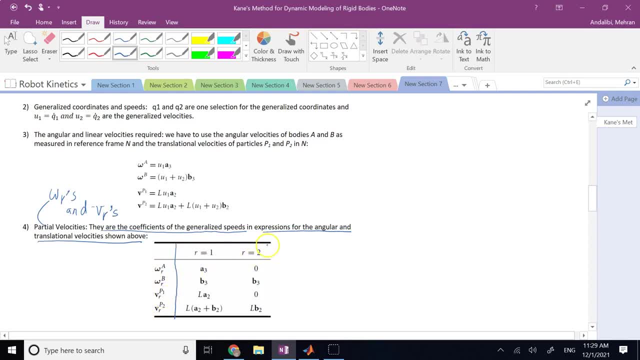 Because here you have two R's. Remember you have two degrees of freedom, So you have two degrees of freedom. R always goes from one to N. N is the degrees of freedom And here N is two. So R only can be one or two. 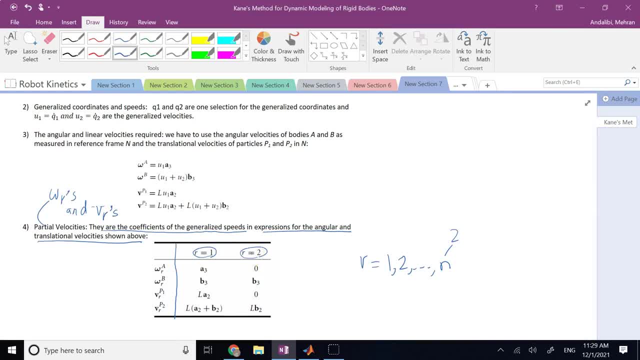 So these VRs or omega Rs, that you have The ideal belonging to R of one, The first degree of freedom, Or R of two, The second degree of freedom. Okay, So now what do you do For omega RA when R is one? 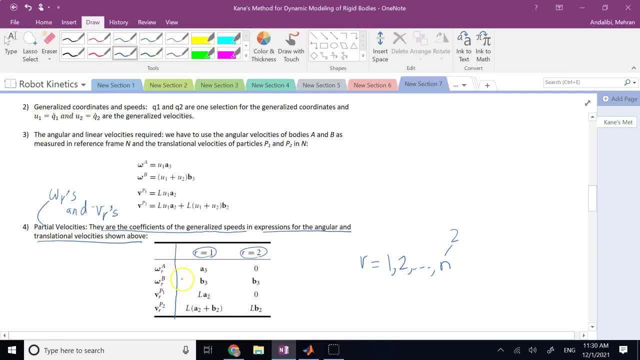 What does it mean? What's the meaning of this? So when I say Omega A, number one, What does it mean? It means the coefficient of Generalized speed, one Which is U1. In omega A, So you can also write it as partial. 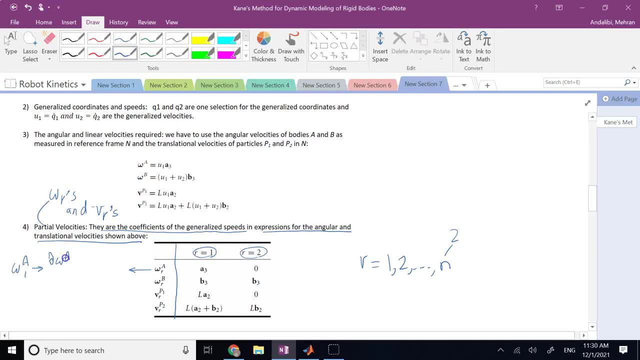 Derivative of omega A With respect to U1. Right And omega A number two Can write it as Partial derivative of omega A With respect to U1.. With respect to U2.. Or the coefficient of it, really, If 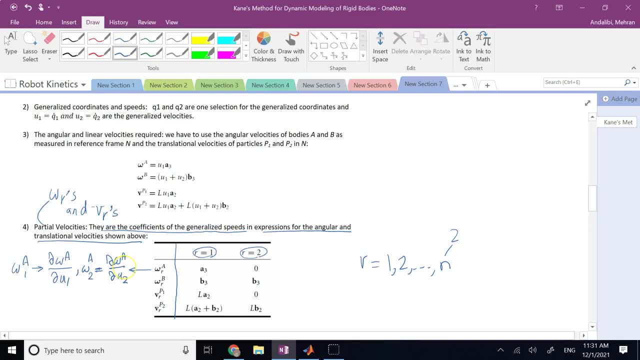 Because they are all linear terms. If they are not linear, You have to use partial derivatives, But they are linear. So what do you get? How many coefficients of U1. Do I have in omega A? I have A3. That's the coefficient. 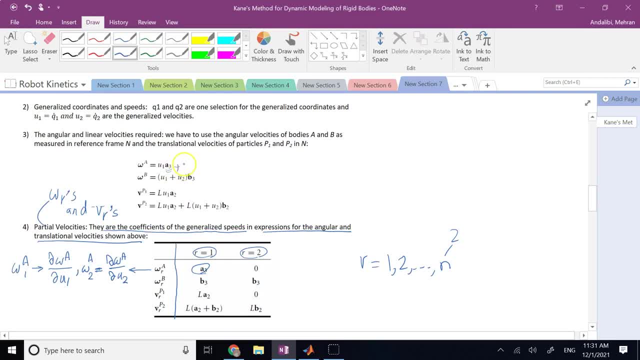 So it goes here. Do I have any coefficients For U2 in omega A? No, It's like U2 times zero. So the coefficient of U2. Is going to be what? Zero? Similarly for omega B. What's the coefficient of U1?? 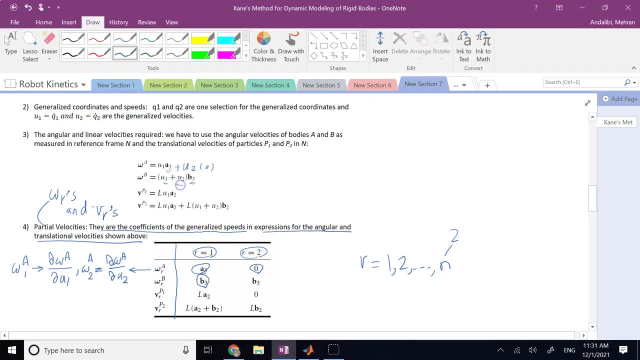 That's B3.. So it goes here. What's the coefficient of U2?? Again, that's also B3.. So it goes there When we go to V of P1.. What's the coefficient of U1?? That's LA2.. 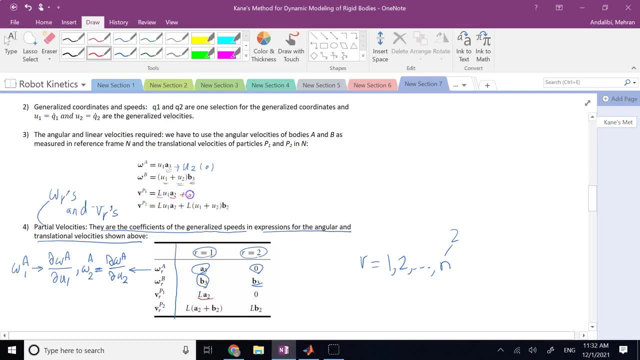 Do you have any coefficients? No, Do you have any U2 terms? No, So you can write it as zero times U2.. And so that zero goes here. And finally, What's the coefficient of U1 in VP2?? Well, I have one place: LA2.. 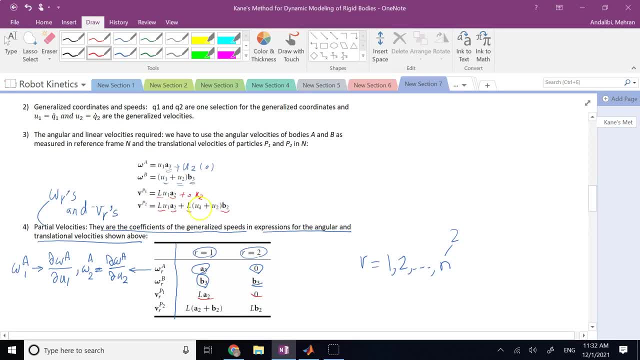 The other place I have LB2.. They are both multiplied by U1. So it's going to be LA2 plus LB2.. Or you factor out L. What do you have for U2?? You have LB2 multiplied by U2.. 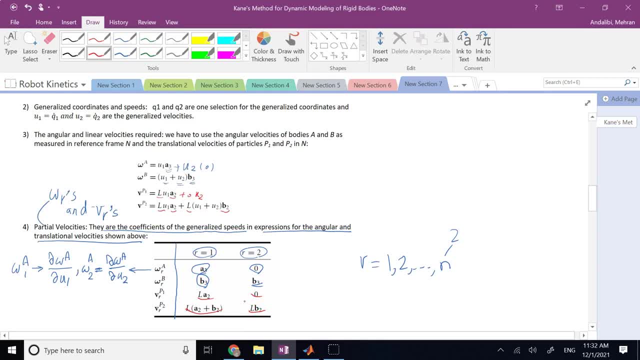 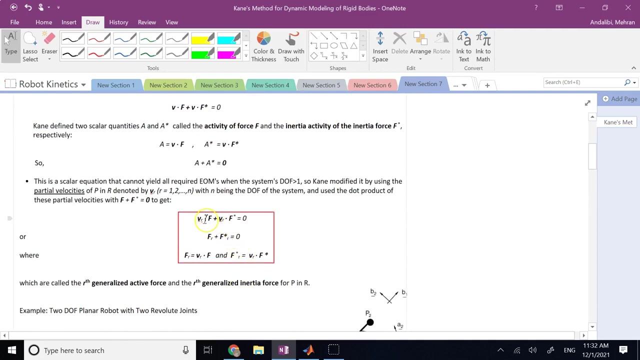 So you get it here Right. So just that simple partial derivative or the coefficient will definitely get you what you wanted. So now that my table is good, I got all of these VR terms and omega R terms- I'm ready to use them into my cane method formula. 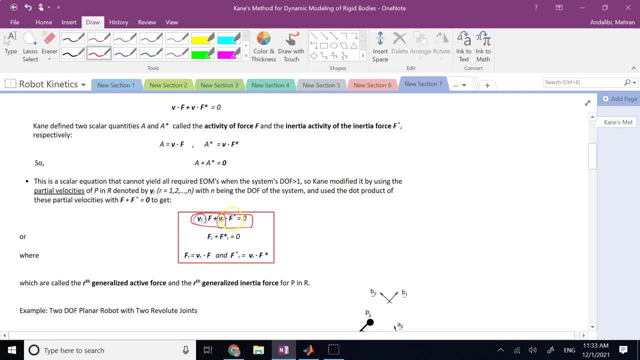 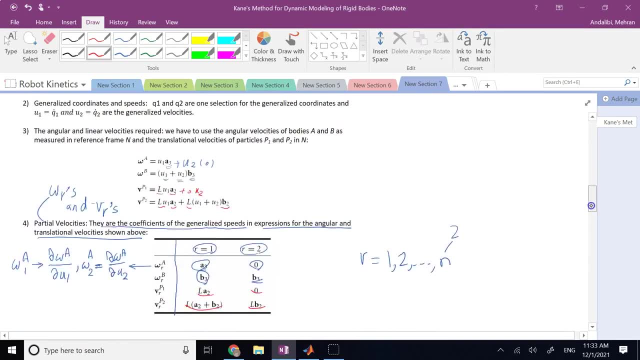 So I've got these parts covered, Except for F's, now The F and the F star. you have to take care of them too. So that's why, in the next step, We have to calculate the accelerations. And you might say: 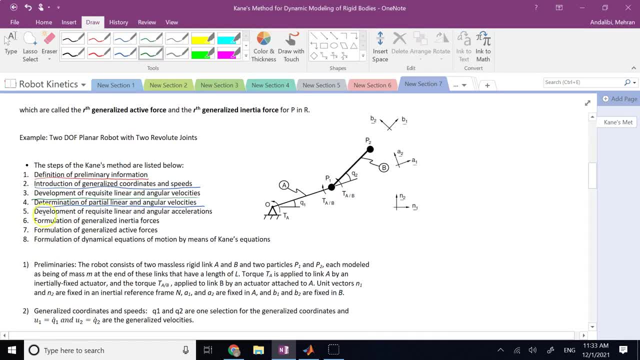 Well, you just said forces. What happened to accelerations? We need the accelerations Why? Because these inertial forces, F R, star, If you remember, They are the masses times the accelerations, Correct? Let's go back here. 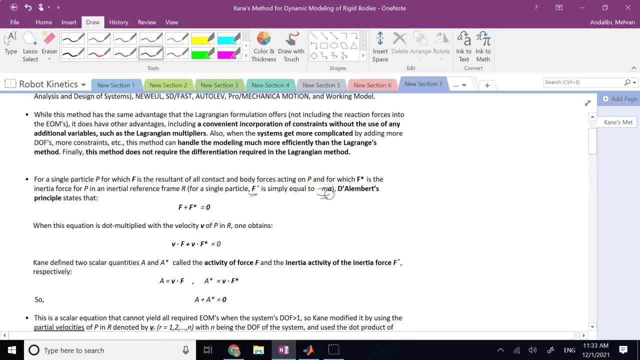 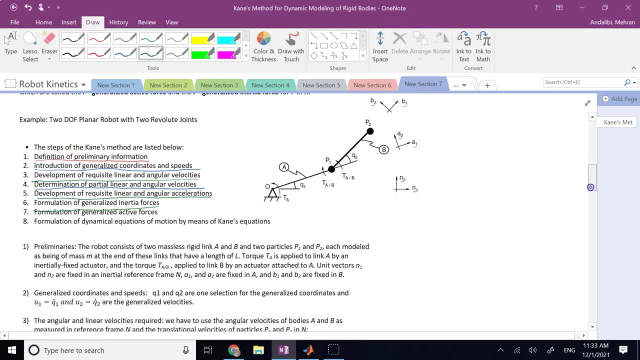 For a single object. This F star is negative M times A. So I need to know A in order to determine F star. So I need to know here the acceleration of The system, linear or angular. that I need in order to go to step number six. 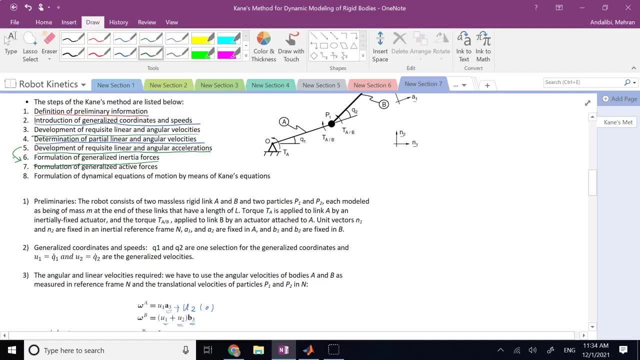 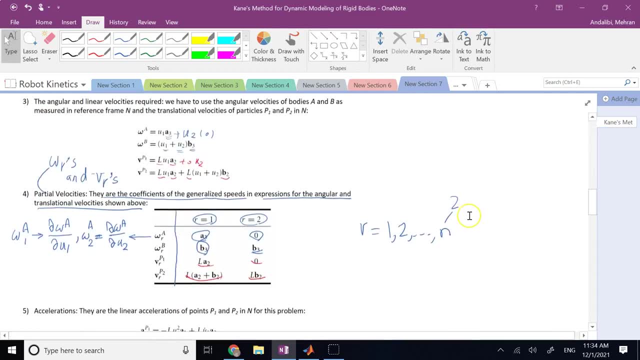 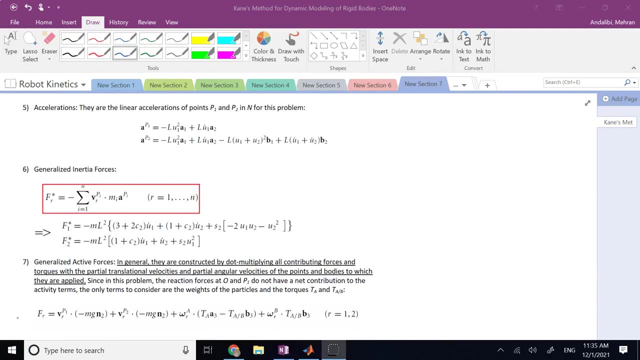 So if I don't know step number five, I cannot go to step number Six. So let's go ahead and determine the Accelerations that I need for step number five, Again for acceleration of the two particles P1 and P2.. 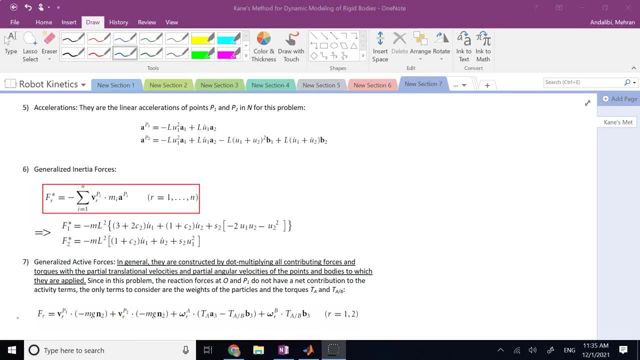 I use the rigid body kinematics. Now, pay attention in this case, Because all I have, all the mass of the system, is concentrated Into the two particles P1 and P2.. All I need to find is the linear accelerations AP1 and AP2.. 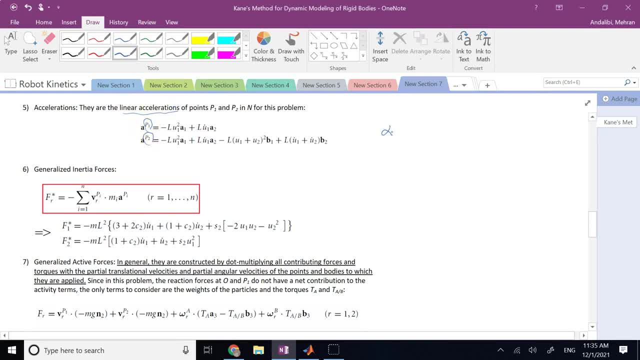 I do not need an alpha, Because alpha is important when you have inertia matrix I To multiply by that and it gives you a torque Right. But in this system these blocks do not have In inertia Because the rigid bodies are No, have no masses. 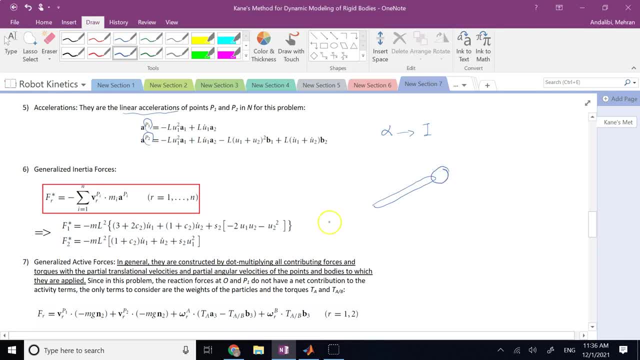 All the mass is concentrated at the particle. Okay, So the rigid bodies themselves are massless, So they don't have I, So I do not need alpha. Just keep that in mind. Okay, So now how do I find them again? 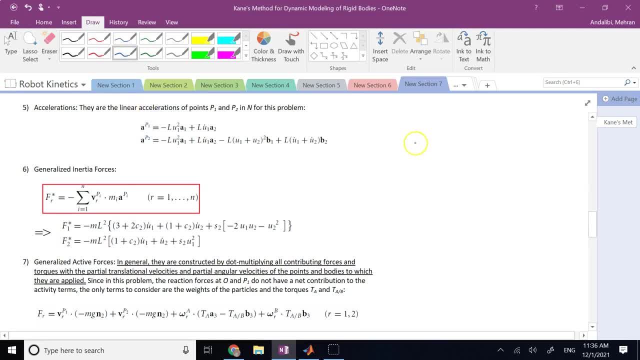 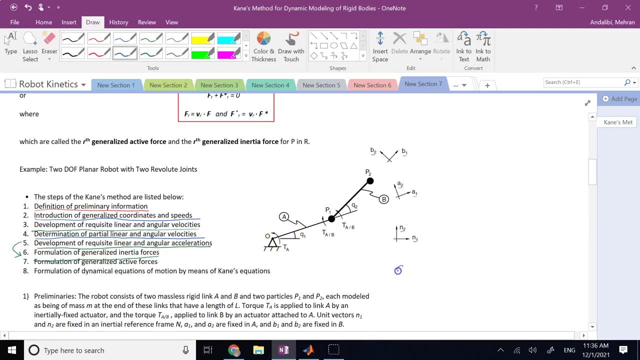 As I said, basic rigid body Kinematics. So what is A of P1? P1 is rotating about the fixed point, So A of P1 is going to be what Is going to be A of point O Right, Which we know is zero plus alpha of member A. 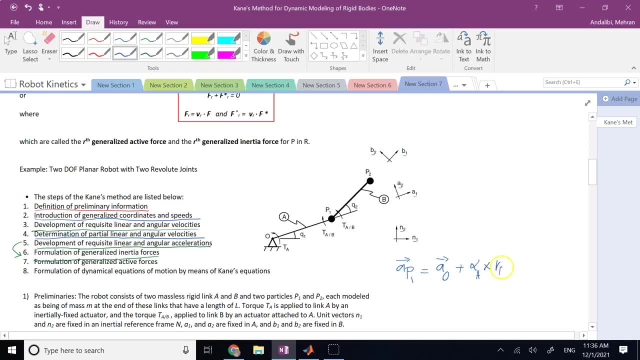 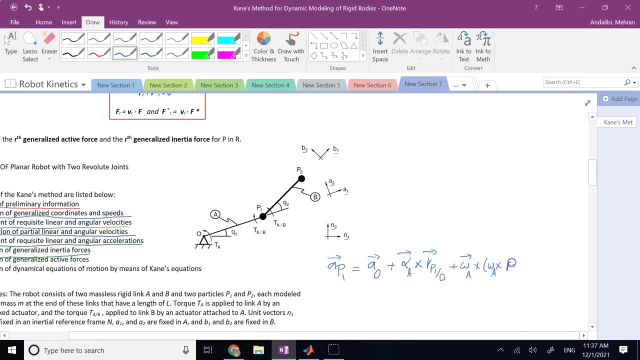 Cross R of P1 with respect to O, And then plus omega of member A, cross Omega of member A, cross R of P1 with respect to O. As I said, we know this guy is zero Alpha of A. Remember, omega of A was what? 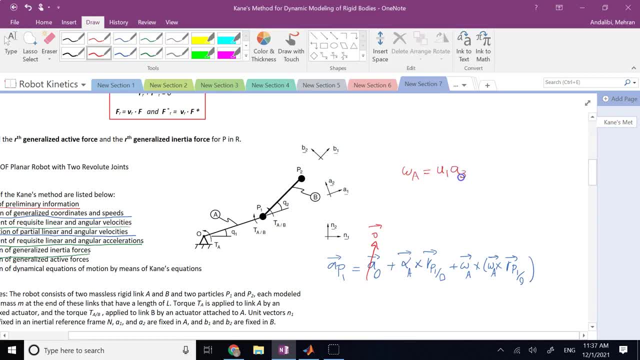 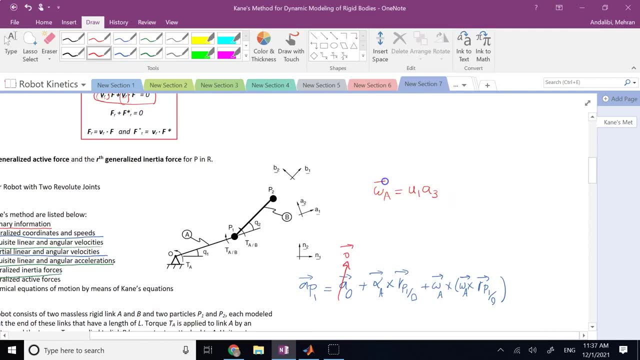 Was U1 in the direction of A3.. Correct, That's what we had right down here. So what is alpha of this member? Alpha of A is definitely what U1 dot in the direction of A3.. Correct, This is all plan or motion. 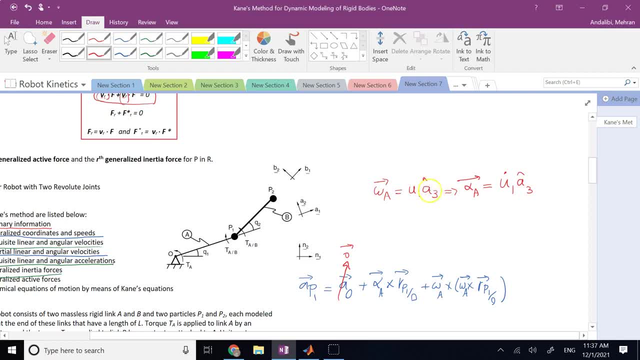 You might say: well, when you take time derivative, A3 does have derivative, Doesn't it? No, Not in this case, Because A3 is always perpendicular to the board, out of the board, So A3 does not change its direction, So it doesn't have time derivative. 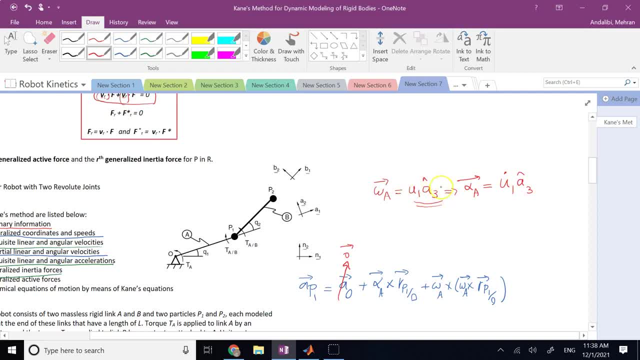 So in this product the only term that has a time derivative is the first one, That's alpha of A. So let's write it down: That's U1, dot A3.. This R vector, as we saw it last time, It is L times A1.. 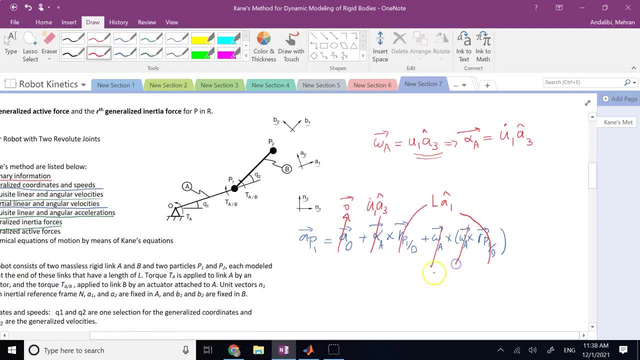 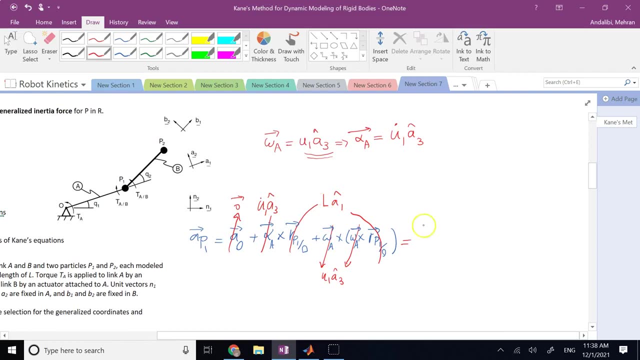 And omega. we just said it, Omega is U1, A3.. And if you simplify this, Here you have A3 cross A1, which is going to be A2. So it is going to be LU1 dot A2.. And the next term is going to be negative. 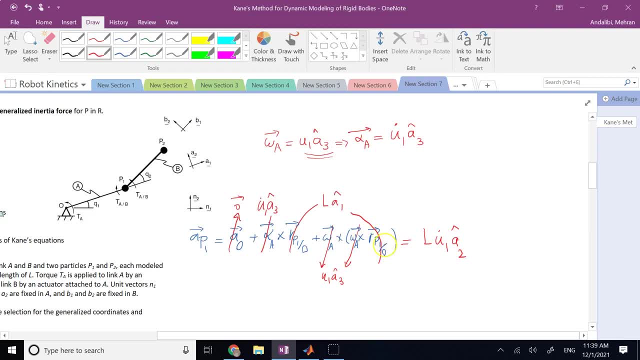 Negative magnitude: omega squared times R. So it is going to be negative. L Magnitude of it is U1, dot Square it in the direction of A1.. So this is acceleration of particle. P. It has two terms. We have this tangential acceleration. 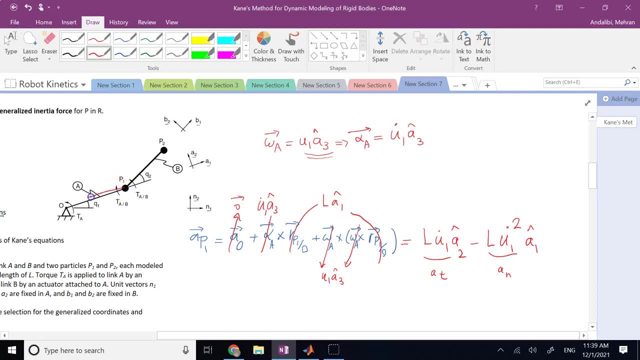 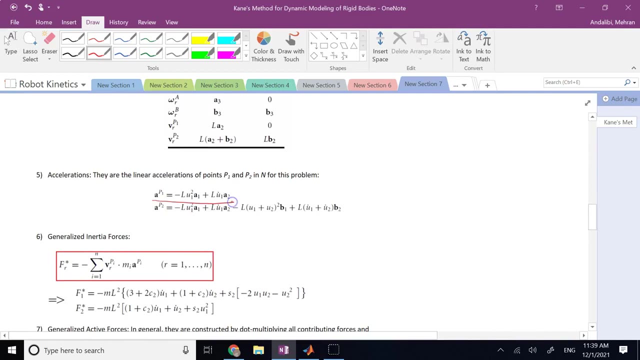 And we have the centripetal acceleration Right. So we have one term here toward the center And we have one term here Right, And we know all of this from dynamics, Right, And that's what you can see here And then for A of P2.. 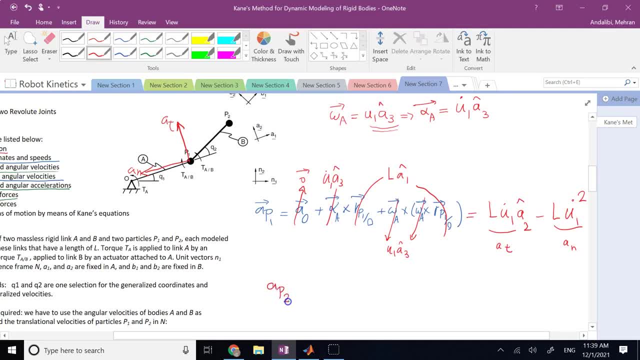 We repeat the exact same thing: Right A of P2 is equal to A of P1.. Plus alpha of member B cross R of P2 with respect to P1.. And then plus omega of member B cross omega of member B cross R of P2 with respect to P1. 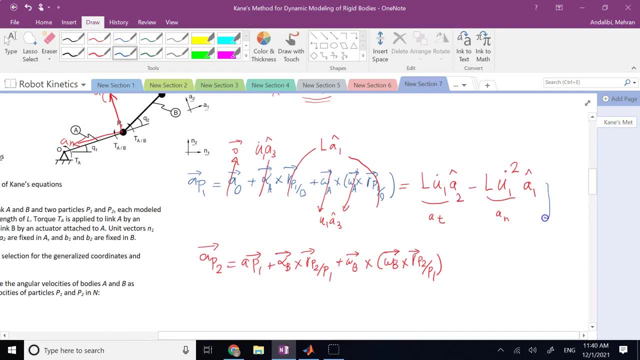 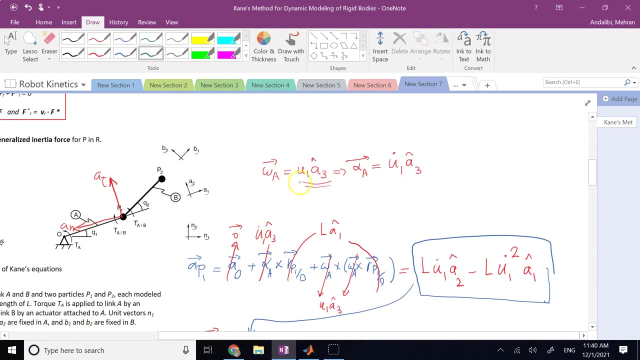 And again A of P1. you directly have it So you can just go ahead and bring this guy down. Right, That's directly given to me. Alpha of member B- Remember, omega of member B was what Was U1 plus U2 in the B3 direction. 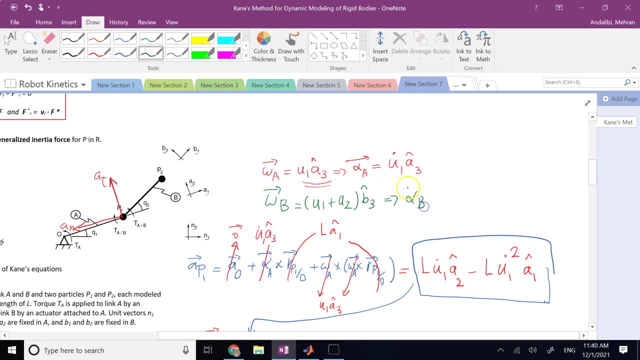 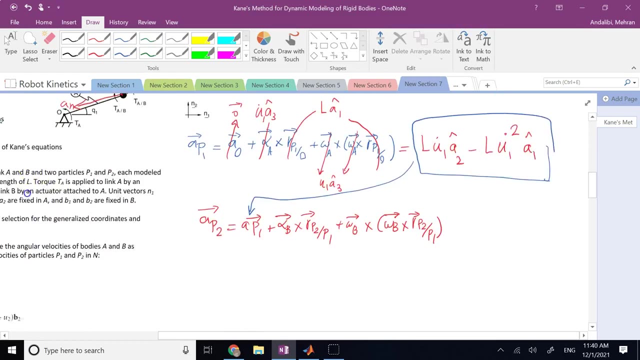 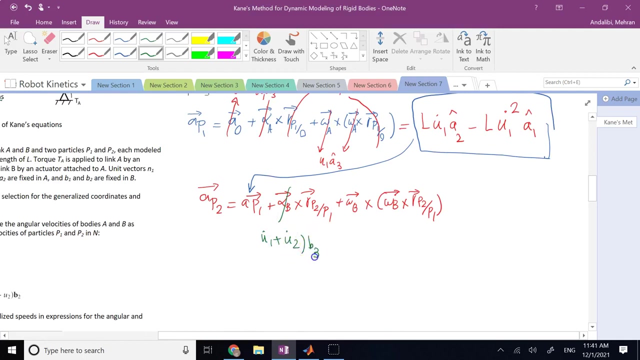 So alpha of member B. Again, since B3 is always perpendicular to the board, outward Has magnitude 1. Has no time derivative, So it's going to be simply U1 dot plus U2 dot in the direction of B3. So you can write it down here: 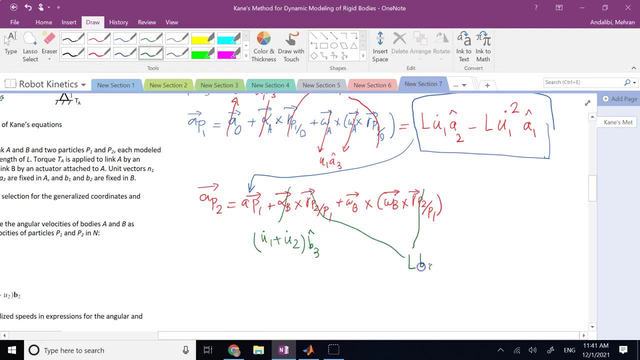 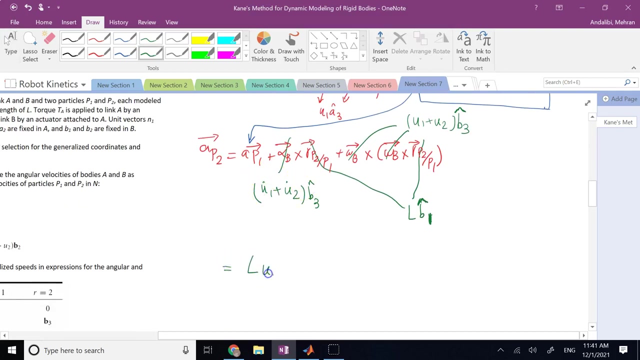 This unit vector is L times B1, as we saw last time, And this omega, as we saw it, was what Was U1 plus U2 times B3. And if we carry this out, you will get whatever A hat, Which was L U1 dot A2, minus L U1 squared A1.. 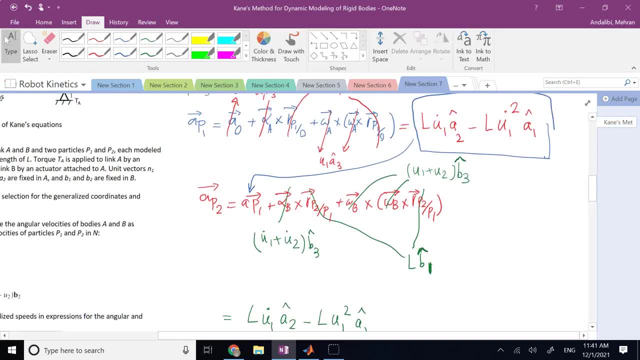 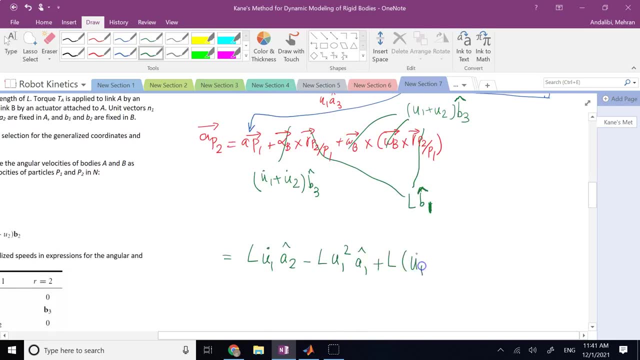 And then plus the relative term, Because here you have B3 cross B1. So it's going to be B2. It's going to be plus L times: U1 dot plus U2 dot, B2.. Then minus L times, as you can see here. 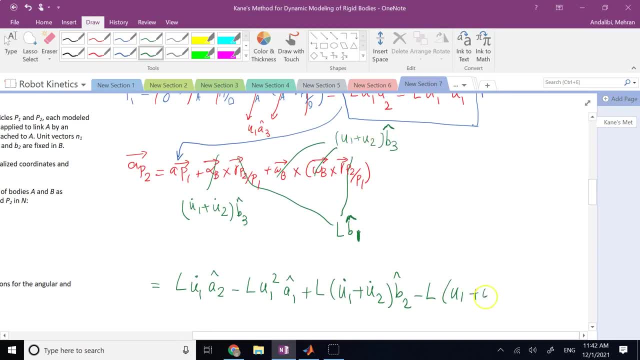 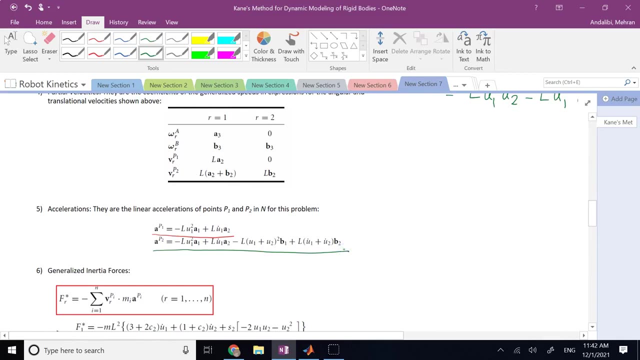 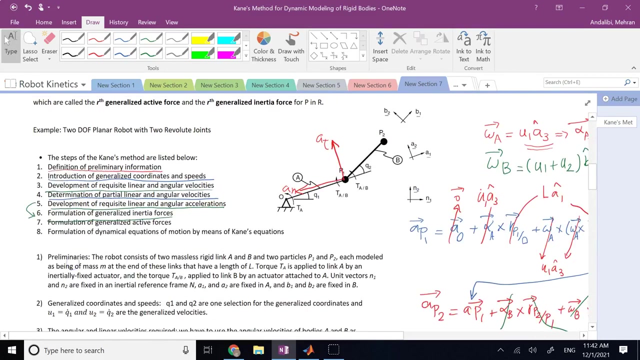 U1 plus U2. The whole thing squared in the direction of B1. And that's acceleration of P2. And again you can clearly see that here. So now I found the linear accelerations I want in the system And I can determine those F star R terms. 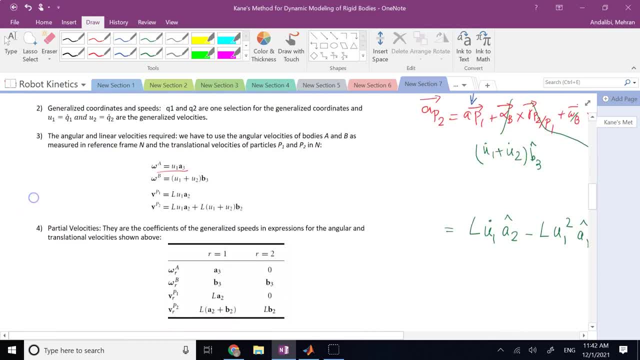 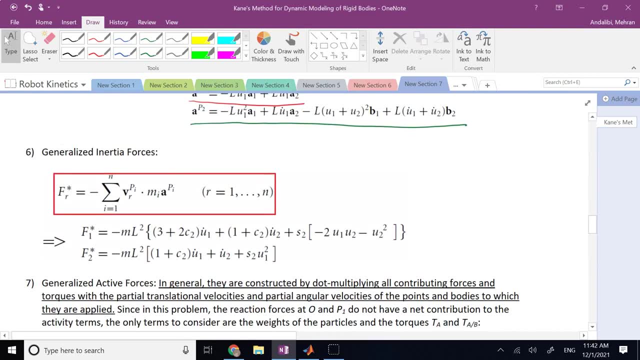 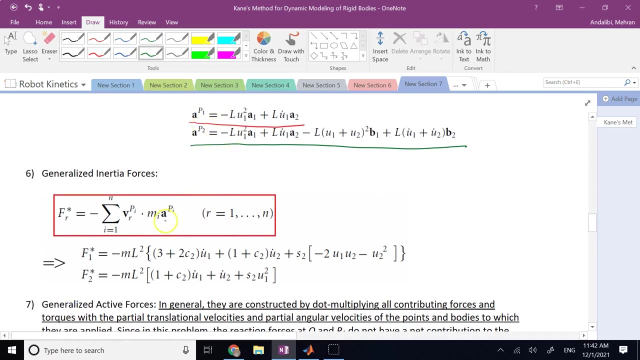 The generalized inertial forces F, star, R. How do I find them now? Well, in order to find those, We multiply each one of these accelerations of these particles by the corresponding mass, And then dot product it With V? R of that particle. 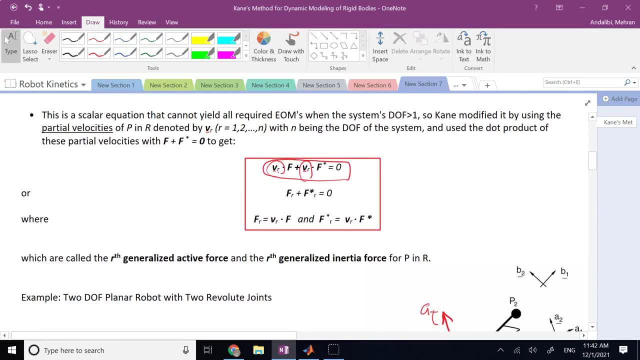 Right, Because, remember, here We define F? R star as V R dot F star, But now you have more than one V, You have several V? R's. Since you have several V R's, Each one of those terms that you dot product. 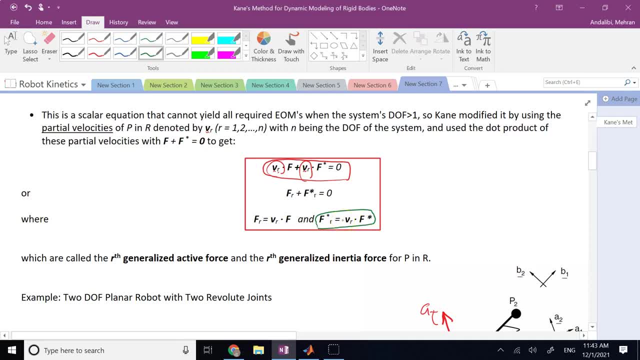 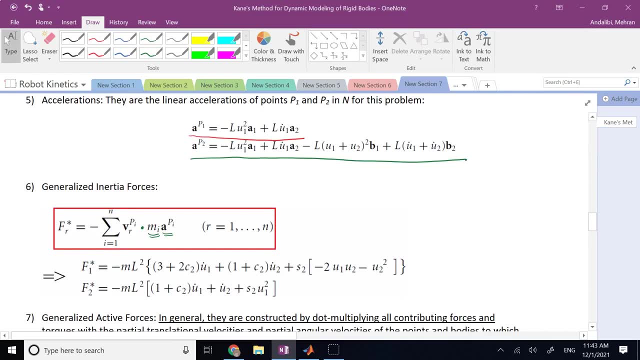 Now you have to add them together to get what? To get the Total F star R, And that's what you see here: This negative M, I, A, P, I. That whole thing is your F star of I, The inertial force of particle, I. 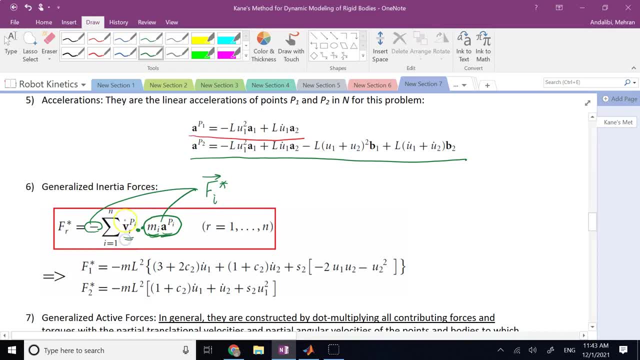 You dot, product that With the velocity of that particle And sum them all over, all particles, And that give you F star R. And there are two of these F star R's, One for R of one, One for R of two. 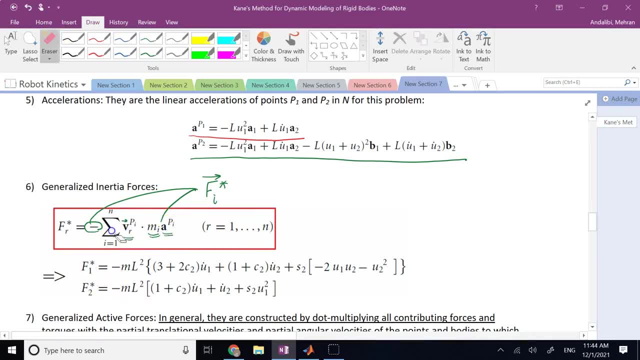 And if you expand it, You should get these two terms for F star one And F star two. Let me show you one of them, at least, Right, So you know how these terms are calculated. So let's say F star two. 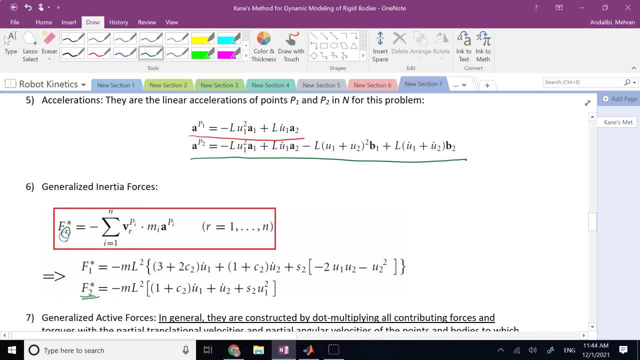 How do I calculate F star two? F star two means R should be equal to two. So what do you get? F star two Equals what, Based on this formula, is negative of R is always two, But I can go from one to two. 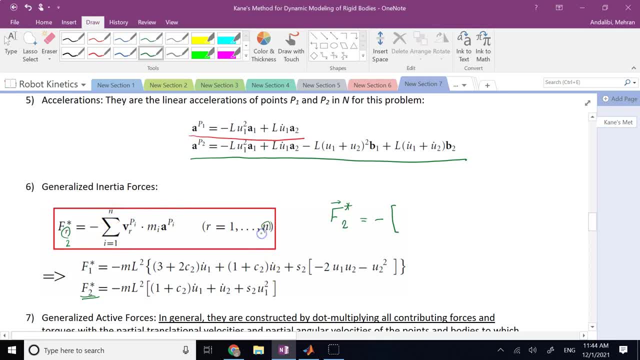 Because N is also two. Right, N is the same N that you have here. So I goes from one to two And R one time goes one, One time goes two. So let's plug in. I have one here, You will get V one. 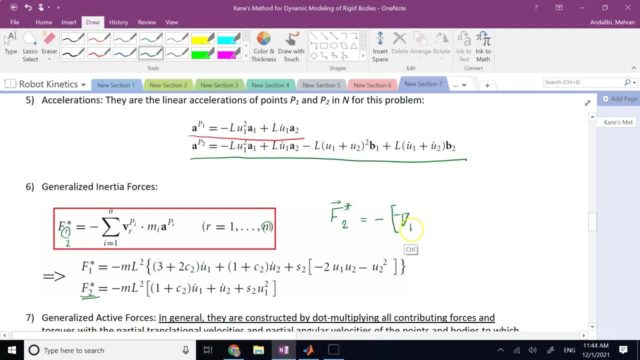 Remember R is Sorry, R is two, So V two, Because R is two. Right Of P one, First I goes one Dot M, one A of P one, Then plus P two, P two Or V of P two. 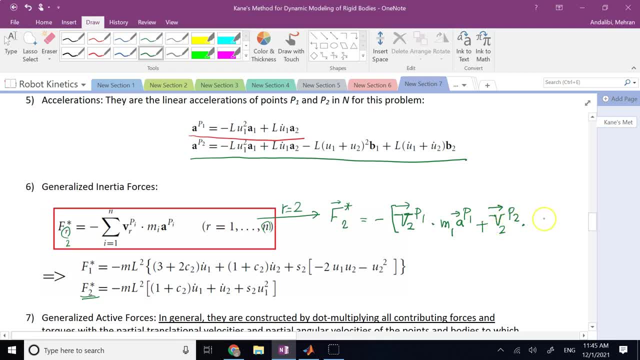 The two components of it. The second component of it, Dot M, two. A of P, two. So this is how we expand it. Now, What do we get? Well, let's go ahead and find these partial velocity terms: V of P one, two. 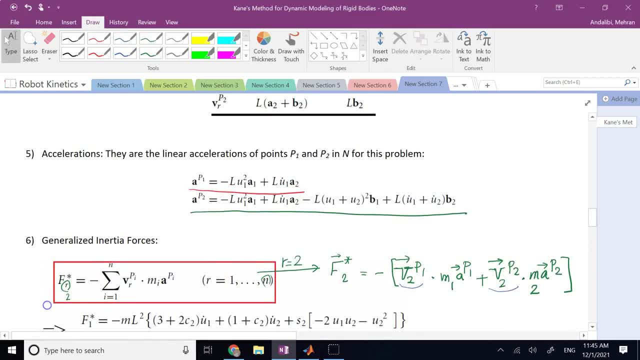 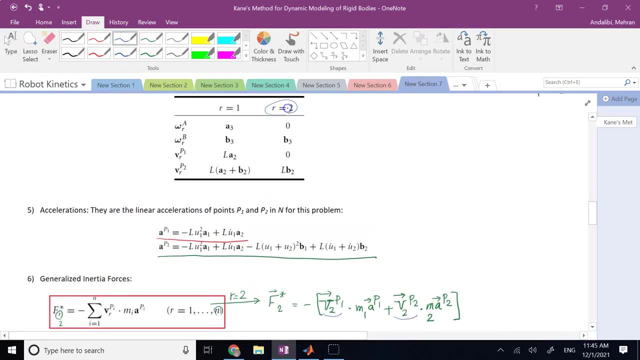 And V of P two. two, Correct, We can find them from my table. Correct, So V two. So I have to go under R of two And one of them is V of P one. One of them is V of P two. 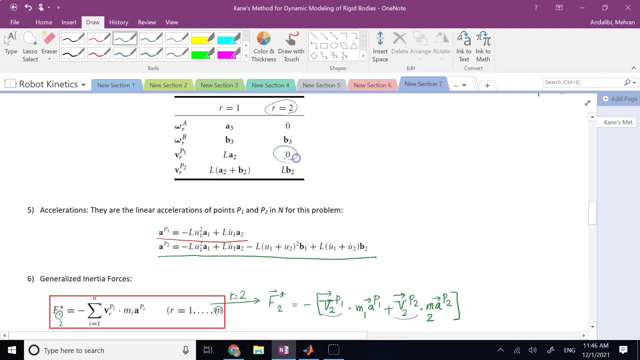 So V of P one for two is this guy. V of P two for R of two is this one. So the first one is what Zero. The second one is L B two, M one and M two. in this case, they are both equal to M. 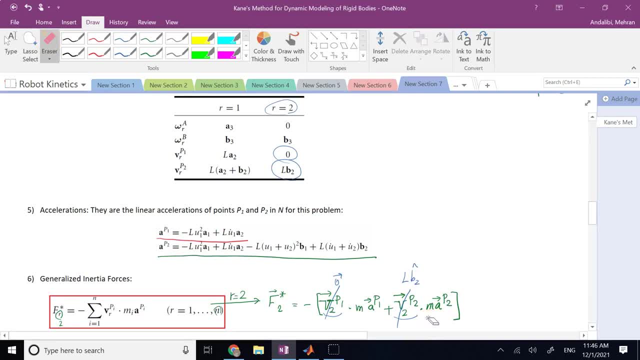 So I can get rid of this subscript. What is A P one? What is A T two? I have them both here, Right? So, first of all, I don't need to write A P one, because it will be multiplied by a zero. 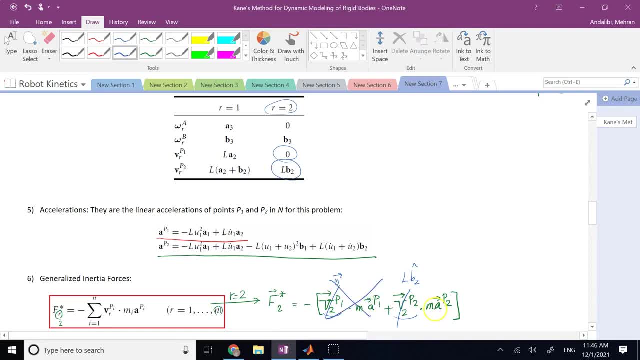 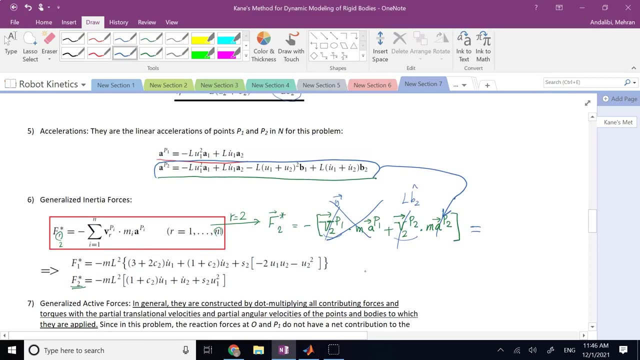 So this term I can completely neglect. All I need is this: A, P, two, which I already have down there. Right, I will bring that whole thing and plug it here, and what will you get when you expand? so all I need really is to dot product this term with that term over. 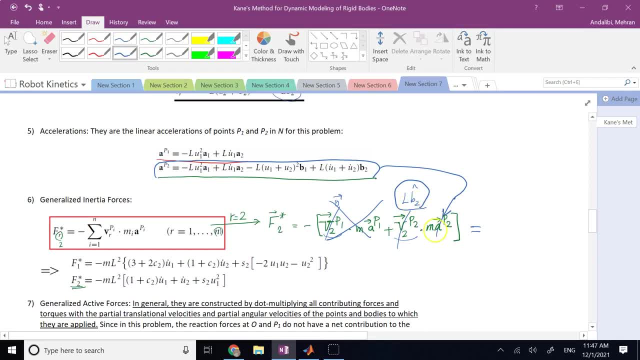 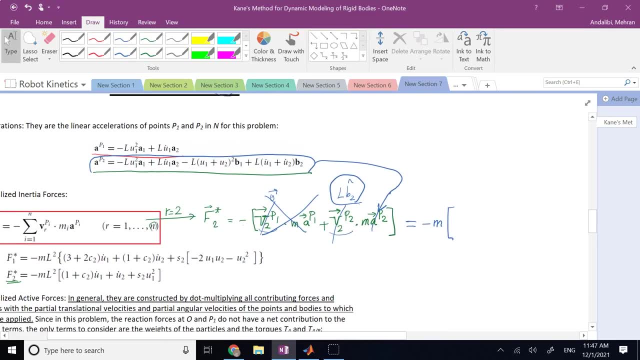 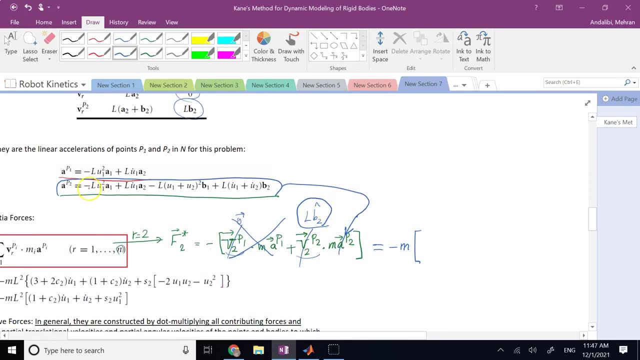 there and there is negative and there is M. so I bring M out. with the negative, it becomes negative M. and then what? now it's going to be lb2 dot. what negative l? u1 squared a1. so if you want, I can write it for you: lb2 dot- negative l u1. 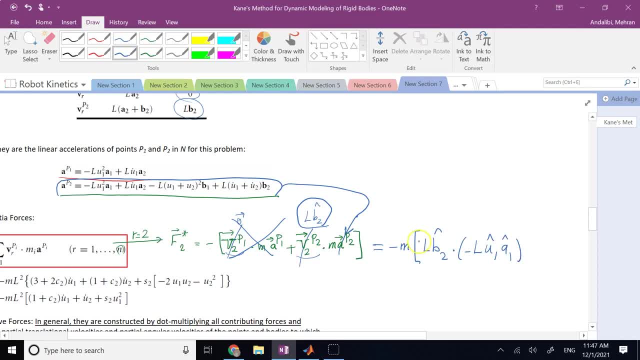 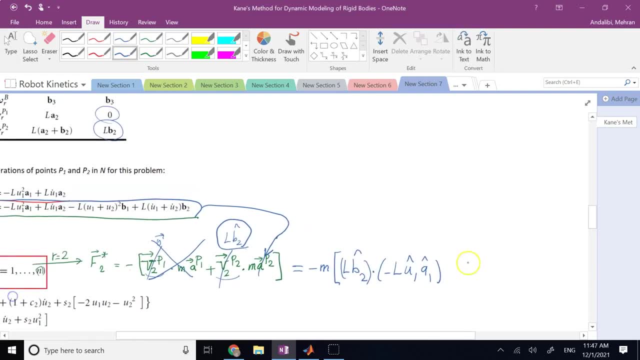 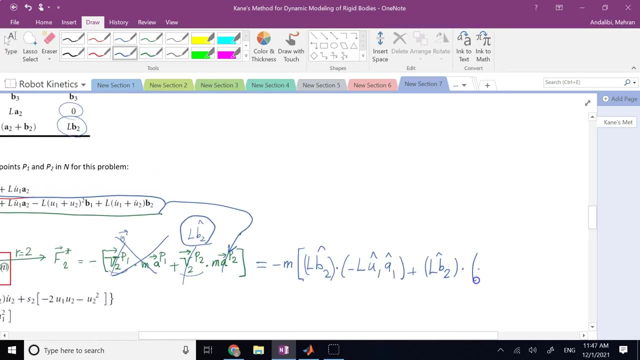 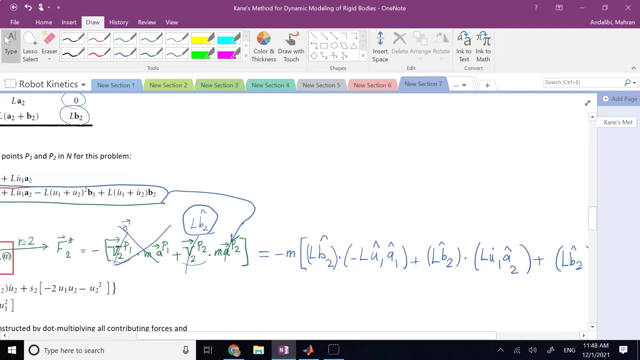 squared a1. this is the first term. and then what again? lb2 dot. now you have the second term: l? u1 dots a2. again lb2 times or dot product. the next term is negative: l? u1 squared a1. so if you want, I can write it for you: lb2 dot negative l? u1 squared a1. 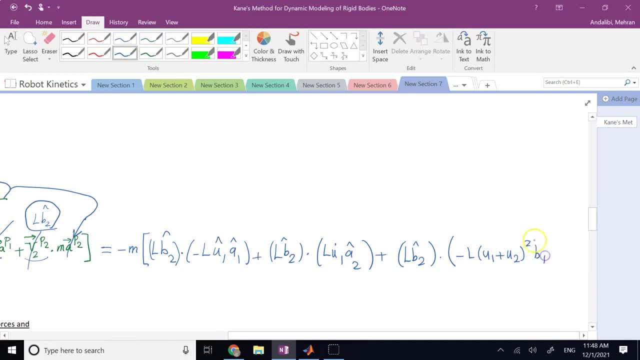 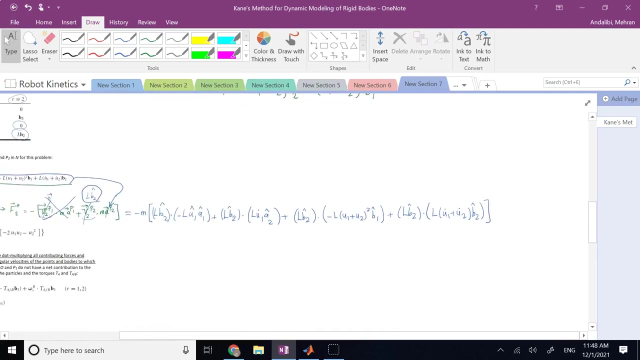 plus u2, the whole thing squared b1 and finally plus lb2, dot, and you have what l, u1, dot, u2, dot, b2. okay, so this is the expansion, now a1 plus the positive derivative, so I can write it for you. so here is the result I'm going to bring it to you. I'm going to use is saves: I'm. 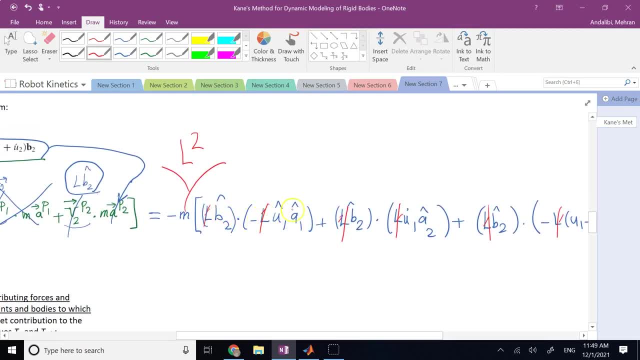 going to double bottom this premise. so I get minus double times l because the portfolio part it equals quit a tangent when I subtract all the extra points said plus b18.5 into L squared, which is than 0.5.. negative here. so what's the result? it's negative of b2 and a1. so what is b2 and a1 dot product? 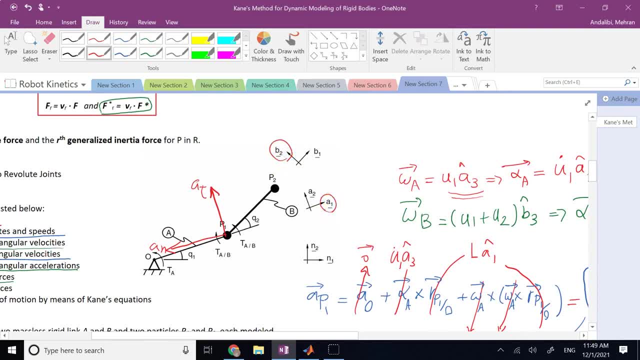 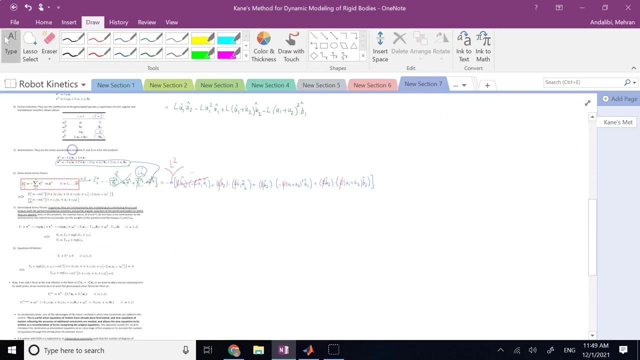 this is b2, this is a1. clearly, you see, the angle between them is 90 degrees plus q2, because this angle, if you draw a1 here, this angle here is q2, so the angle between b2 and q1 is 90 plus q2. so when you do dot product, 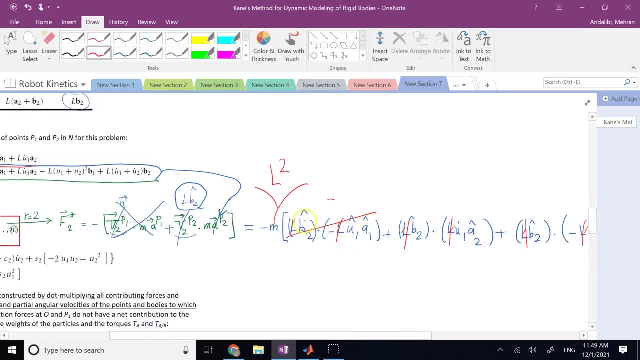 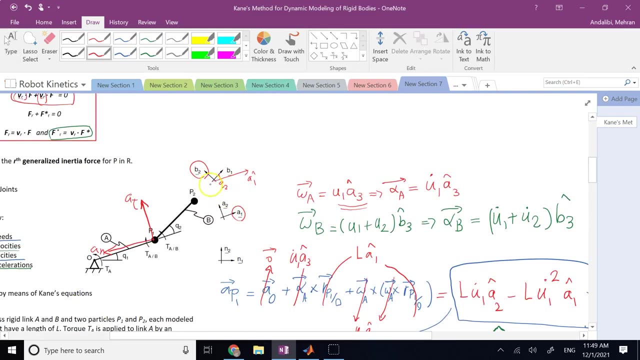 dot product of two unit vectors is magnitude first one, magnitude second one, which is one and one, so it's going to be cosine of 90 degrees plus q2. here you have b2, here you have a2 and a2. clearly, b2 and a2, the angle between them is the same as a1 and b1, and 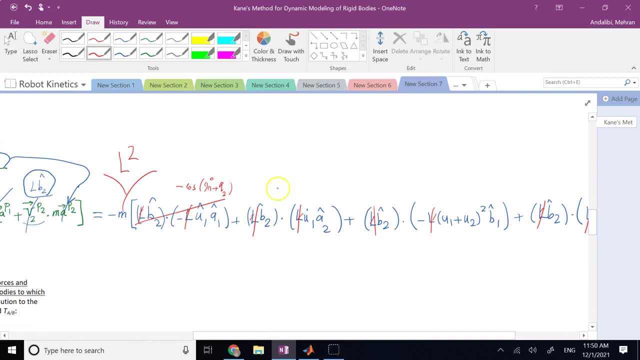 that is q2. so definitely here you will get um. one more thing here: this u1 will come out as well, and it doesn't have a hat because it's just a speed. so this one is going to be. It's going to be U1, dot and then B2A2,, as I said, is cosine of Q2, correct? 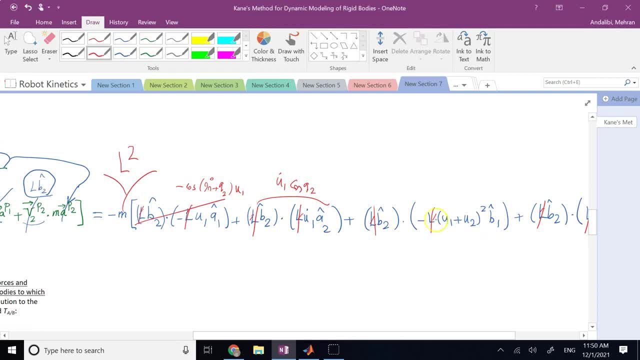 What about here? B2 dot B1. We know B1 and B2, they are perpendicular to each other, so the whole dot product is going to be 0. And here you have B2 dot B2, which is 1, so all you will get is really U1 dot plus U2. 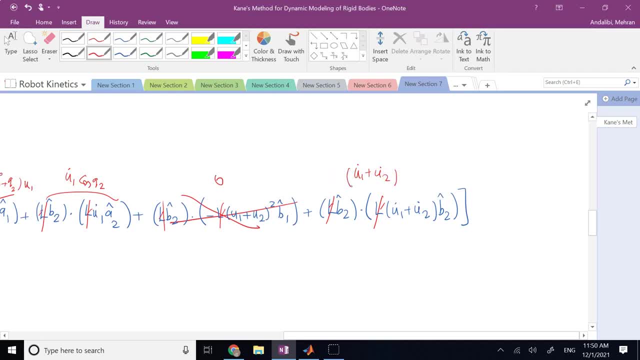 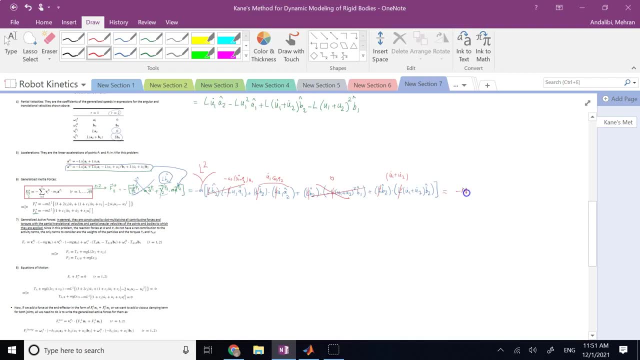 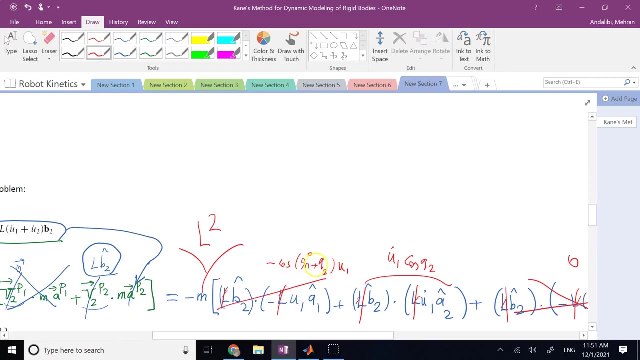 dot times, cosine of 0, which is 1.. So if I want to simplify, you will get what Negative ML squared times what From geometry you know. cosine of 90 plus an angle is negative sine. With that negative sine it becomes positive sine. 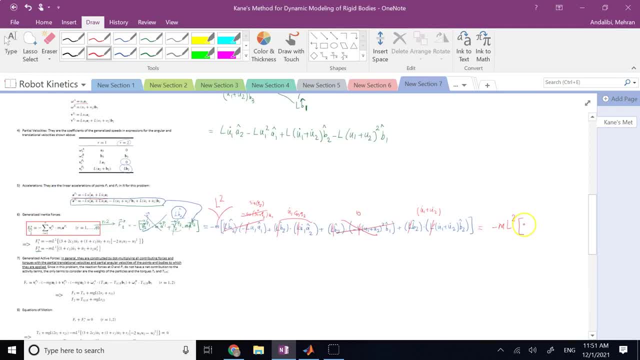 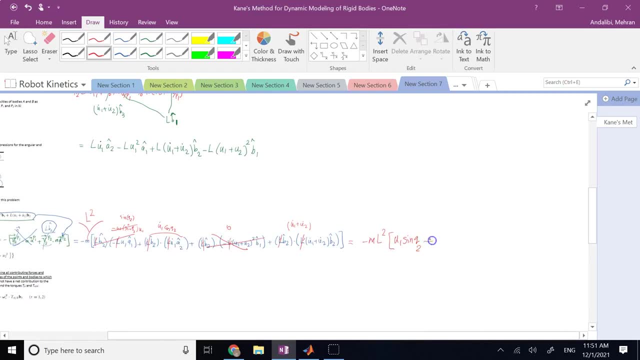 So it becomes U1 sine Q2.. Plus U1 dot cosine Q2.. And then plus U1 dot plus U2 dot. Or you can factor these two out to say U1 dot times 1 plus cosine of Q2.. So it's U1 dot times 1 plus cosine Q2, plus U2 dot plus U1 sine of Q2.. 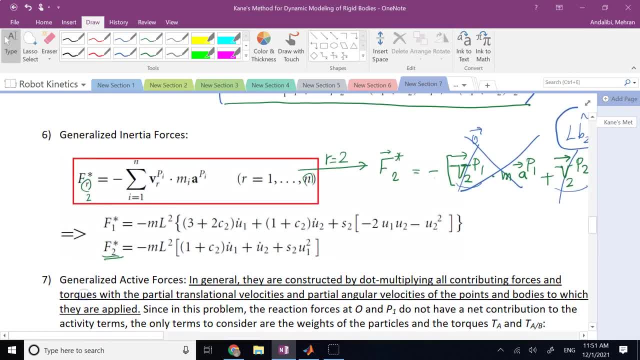 The whole thing Times negative ML squared. That's exactly what you see here. C2 here means cosine of Q2.. And if you do this time expand it for R equal 1, you will see that F1 star is going to be. 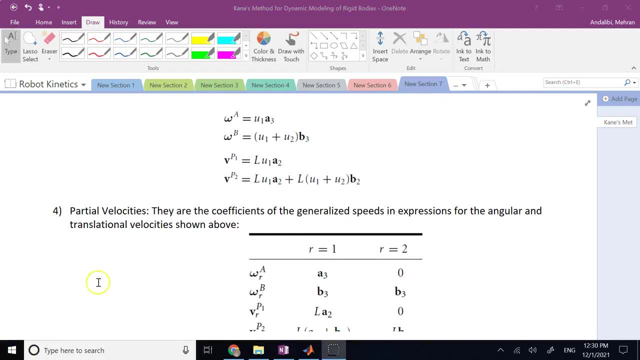 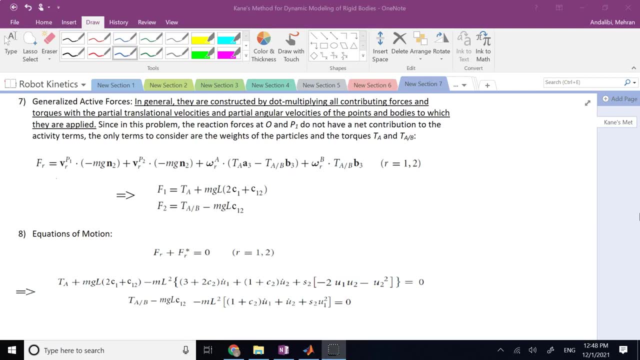 that whole big thing. Okay, So now we have to calculate the generalized active forces and equations of motion. So for generalized active forces, what we need to do is to dot product dot, multiply any active force or torque by the velocities of the points or the bodies to which they are applied and add them together. 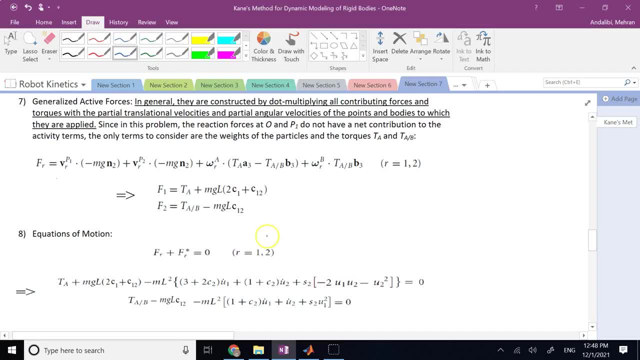 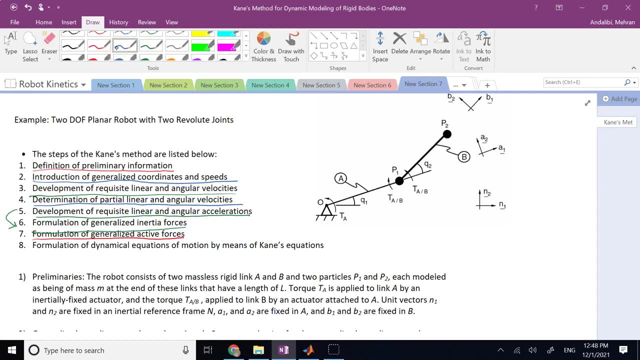 So, if you remember, we look at the free body diagram or the robot here We had TA and TAB right As well. we had these MGs. We learned that there are two forces. If I look at the free body diagram of the entire robot, there are two forces at O as well: OX and OY. 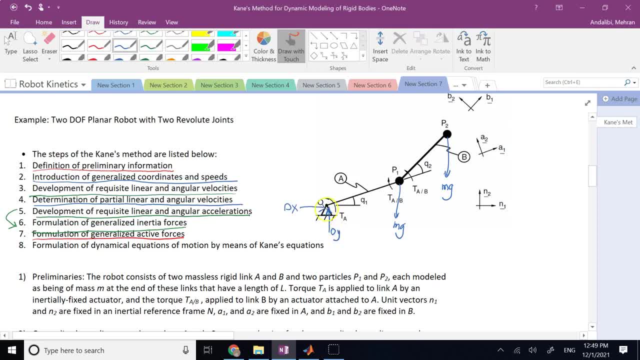 But they are not active forces. They are applied to stationary points. That point does not have a velocity. So So those two we can exclude from our calculations and formulations. These two MGs, if I want to write them in terms of the unit vectors, they are definitely negative MG times, N2 direction, correct. 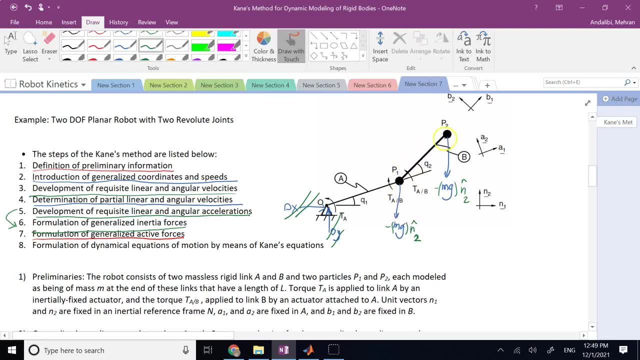 And so now, since these two forces are applied to P1 and P2, and there are particles, so for each one we need the velocity of the corresponding particles. So I need velocity of P1 and dot product the other one by velocity of P2.. 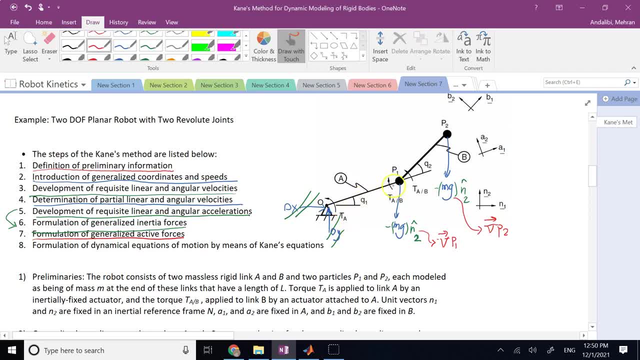 And then the torque TA that is applied to rigid body, A that should be dot producted by omega A because that causes a rotary motion, And similarly, T of AB that is applied to block B that should be dot producted by omega B because that's the cause of the motion. 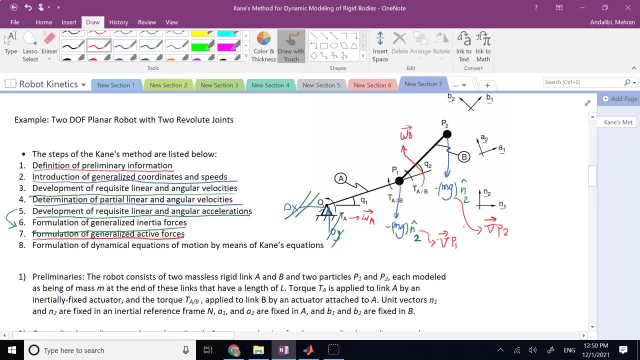 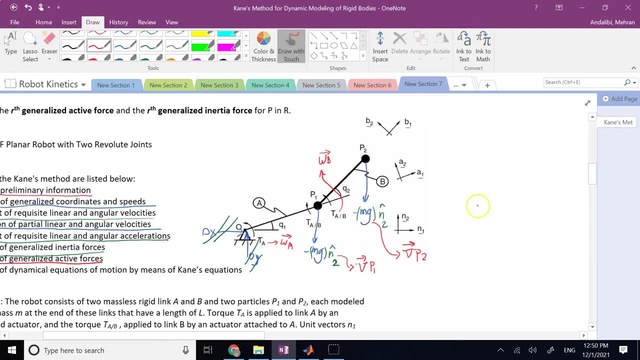 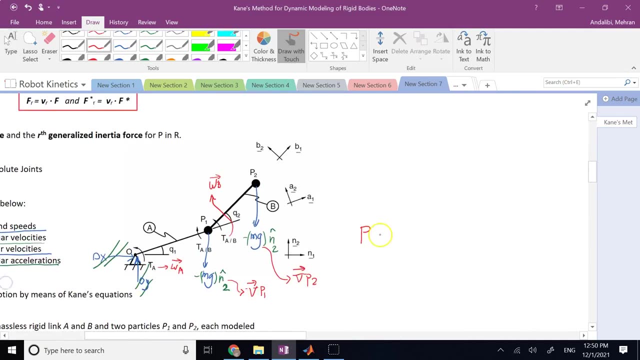 So when we do the dot product of these four terms and add them together, that is the total active forces that you have. And remember that the definition of power that I initially described for you- power if the system is a linear system, it is going to be V dot P, V dot F. I'm sorry. 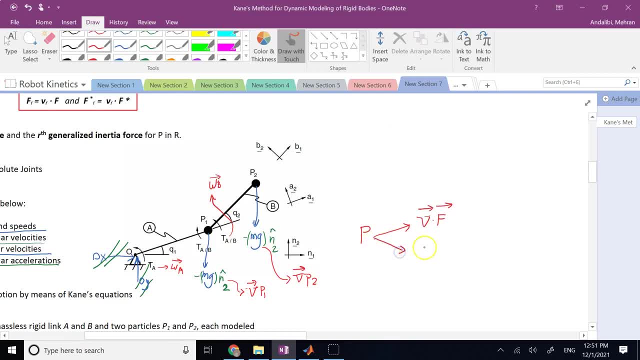 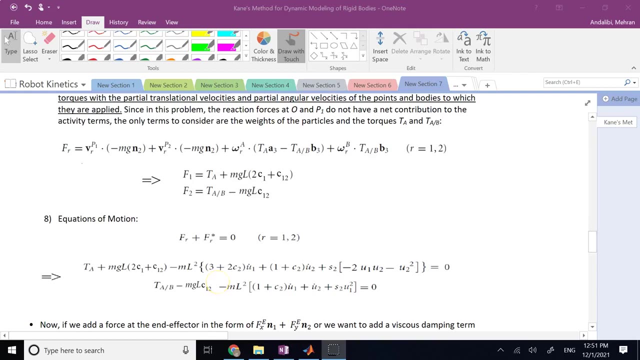 If the system is a rotary system, it is going to be omega, dot T, okay, So that's what you see down here. So if we go down here, we can see these four terms right: This one, This one, This one. 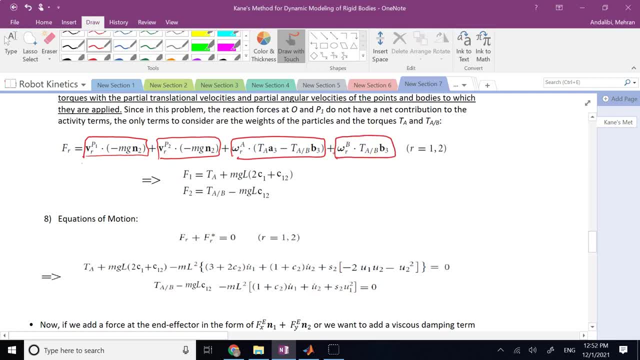 And this one. So they're all clear. The only thing I might need to explain is here: why is it that omega A dot producted with TA minus TAB, not just with TA? The reason is, when you have this rigid body A, it has this. 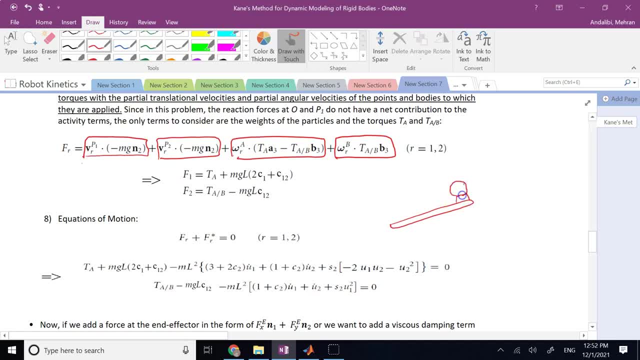 It has this motor on it and this motor is turning rigid body B. so the torque that you are applying to block B, object B, you call it TAB- the reaction of that is applied back to the motor and motor is rigidly attached to block A. 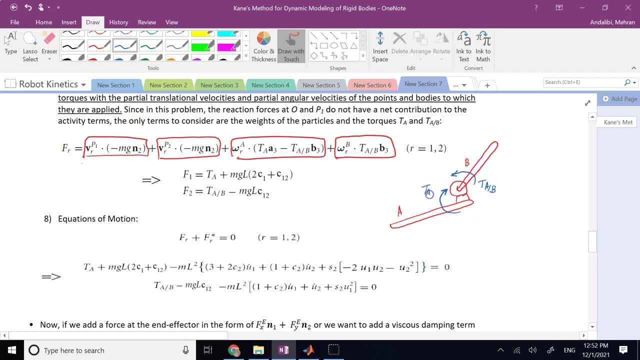 so you have a reaction TAB, So you have TAB backwards on block A and you also have this T of A. So this TA was in the direction of A3,, if you remember, and that TAB is in the direction of B3. 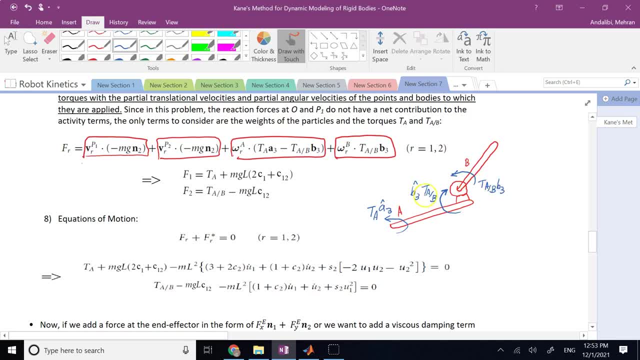 Okay, And because this is a reaction, use the negative sign. So here I have to add those two together, which is the net torque on block A. So here I have to add those two together, which is the net torque on block B. So here I have to add those two together, which is the net torque on block A. So here I have to add those two together, which is the net torque on block B And that TAB also on block A. so this can't be applied back to B3, and it's the reaction of that TAB on block A. 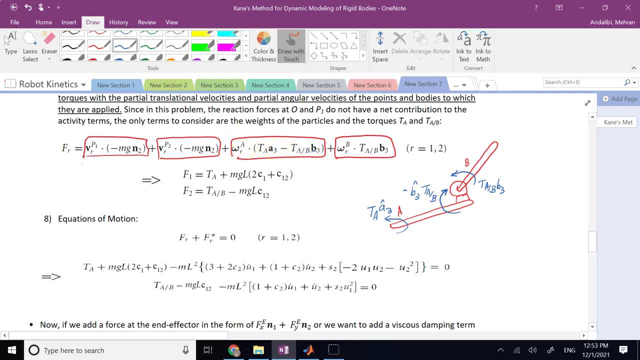 And that TAB also on block B. All right, let's solve it by perhaps applying two A fans to this f of A, And let's donc for this and put it in the buzzing area. So this is fixed. We have two winds of A. the first is the wind flow. 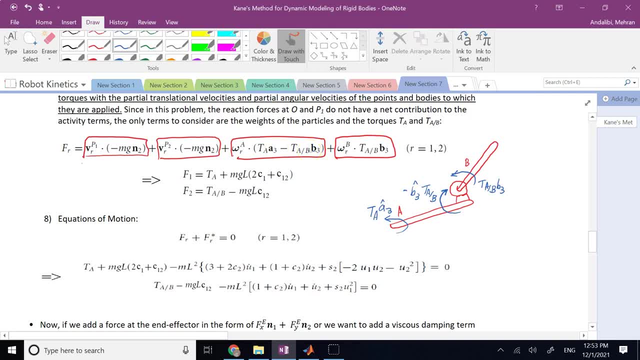 The second gets the called mistaken fenomene. The third is the force of R. So the difference is the strength of the beam from the voltage gainNA2, the maximum force on the d-axis arc is the force on theonian wave. 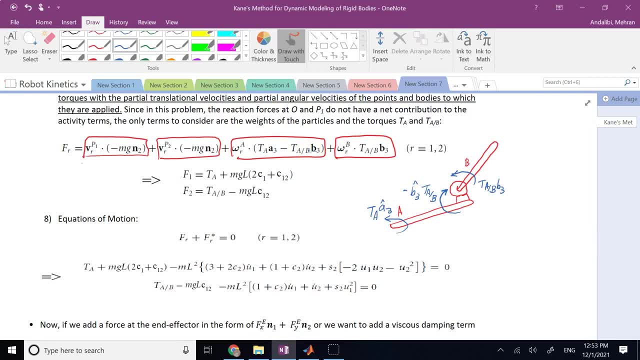 So once again. so here we have a method to apply corner participle H fim, and that is r. now, r can be one or two. so if i apply r of one one time, i get f1. if i apply r of two, i get f of. 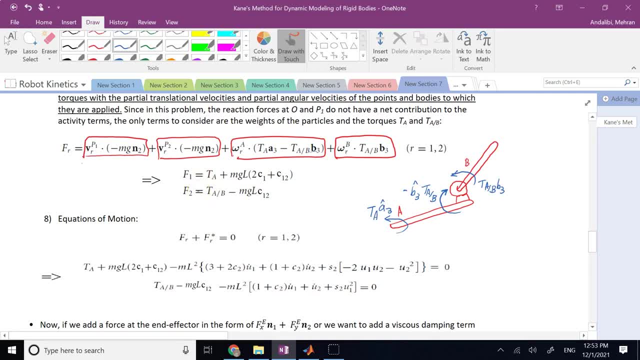 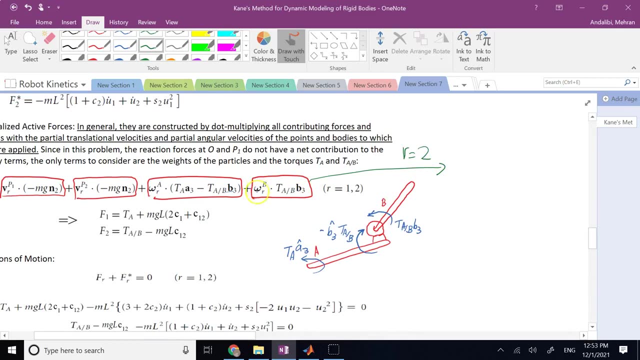 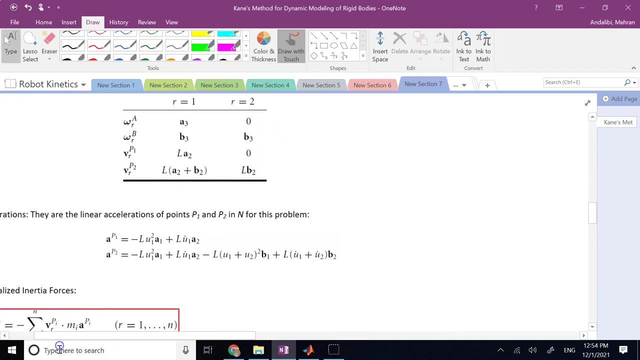 two and then i get both of my basically generalized active forces. so let me show you one of them. for example here: if i apply r equal two, here what's gonna happen? so when r is two, i need omega b of two, omega a of two, vp and v? p one and vp two of two. so basically i need to go to that table. 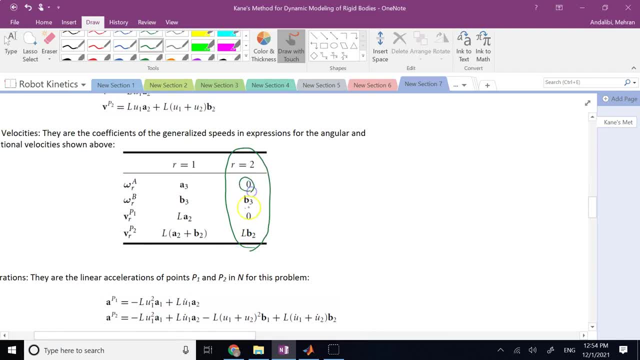 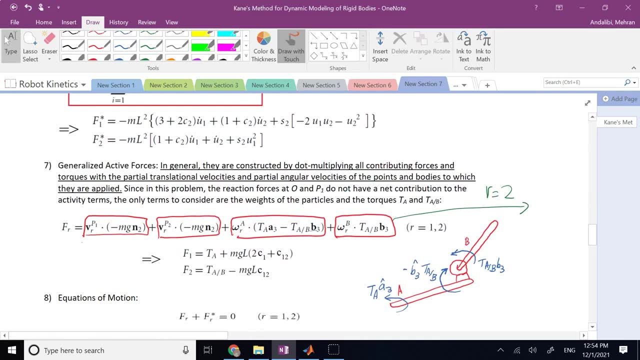 and i need to look at the second column. so these are the terms i need: zero b, three, zero lb2, and if i go down here and basically consider them, this one was zero and, uh, this one is l b 2, this one is b 3 and this one is zero. 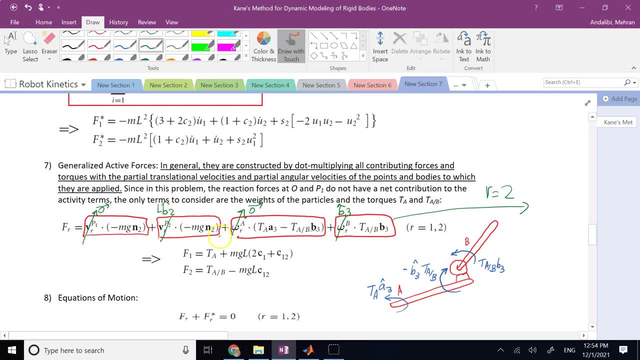 so if you expand it is going to be lb2, dot, mg, n2 and then b3.tabb3. so this last one is very easy, because b3.b3 is one, so you're just going to get tab. that one is going to be negative mg times l. 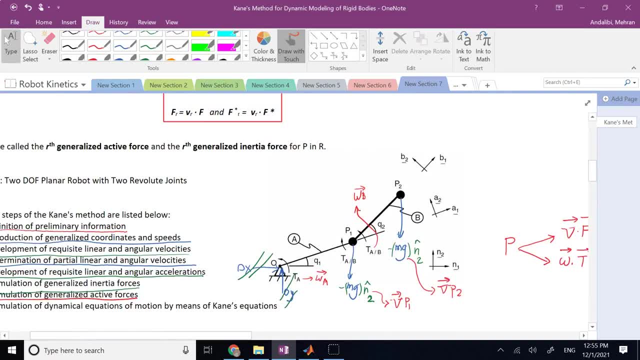 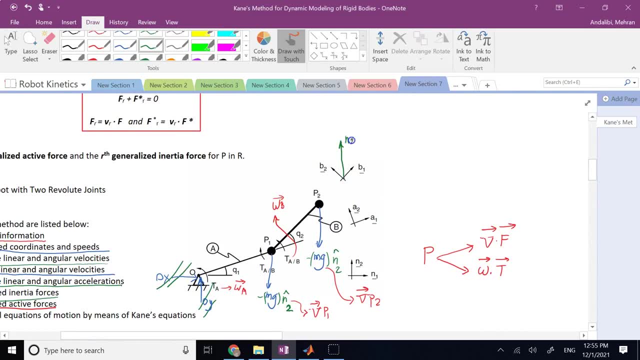 times b, b2.n2, and for that i can go up here that is b2, n2 is upward and the angle between b2 and n2, this angle is clearly q1 plus q2, so it's going to be cosine of q1 plus q2 here. 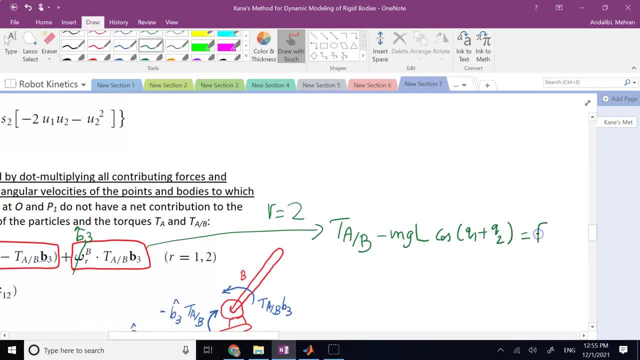 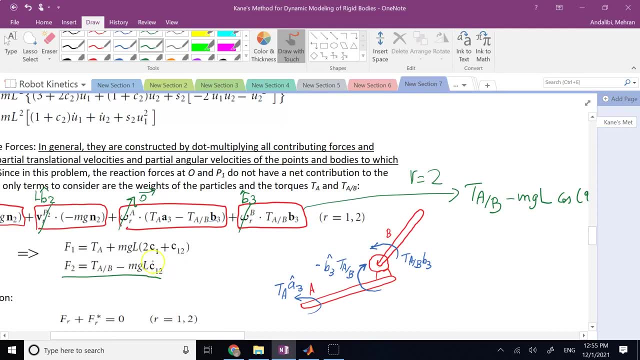 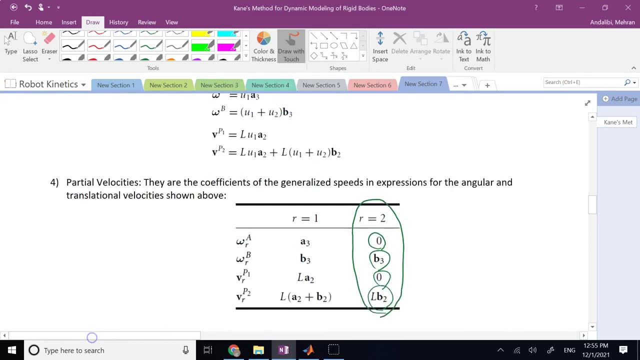 so this should be equal to f of two, and if i go down here you can see that's exactly the case. instead of cosine of q1 plus q2, i will use this short form, notation c1, 2.. and definitely if you apply r of 1 here, that you need to go and choose the first column. 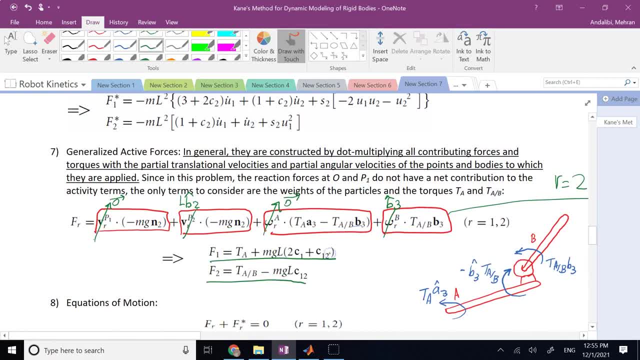 variables, then if you plug in you will get this f1, and now, since you have f1, f2 and f1 star and f2 star for each r, you add them together. so if there are rows which include x1, F2- and i care about them, drawing the html columns in the lower left corner, then you can do this by putting a cell in here and you're done. 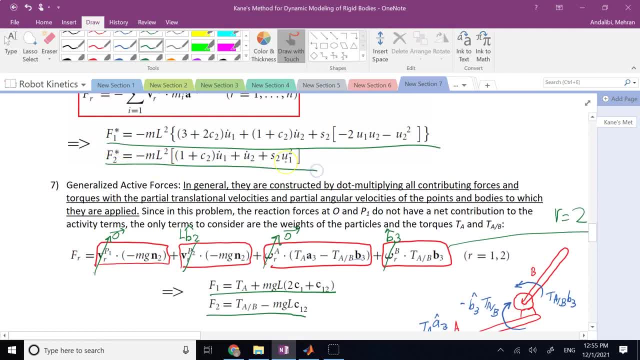 f1 and f2 and f1 star and f2 star for each R, you add them together. so instead of applying the column, you just plug in and turn. and f2 star for each r, you add them together. so first you get f1 plus f1 star equals zero. 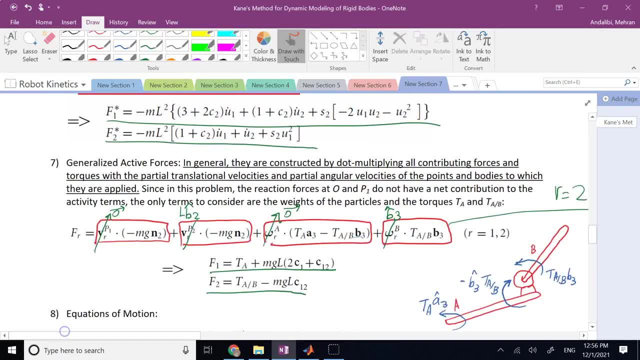 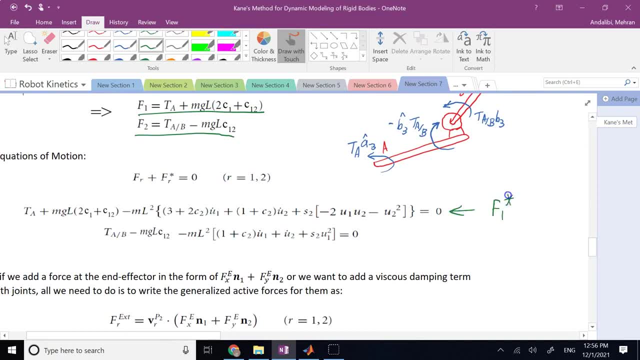 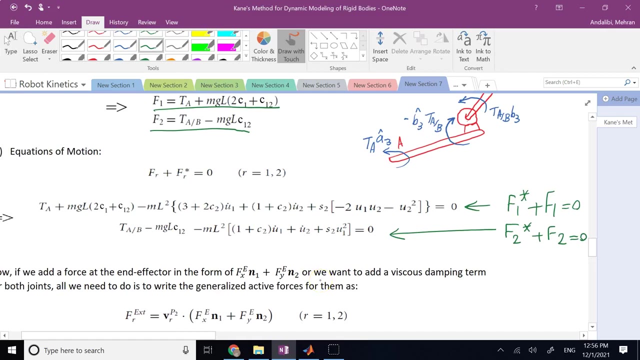 that gives you this equation. then you say: f2 plus f2 star equals zero. that gets you the second equation correct. so these are your two equations of motion derived by the cane method, and that's it now, as i said, they might not look so easy here, but, as i said, when the degrees of freedom go, 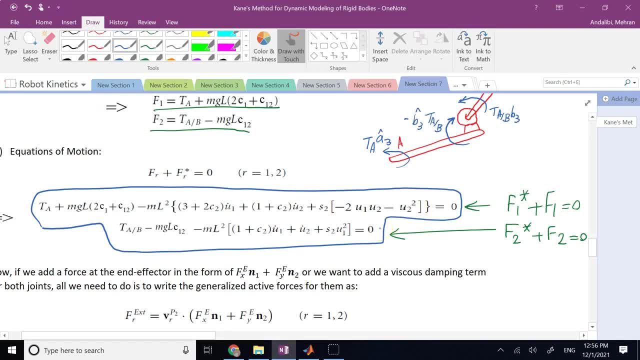 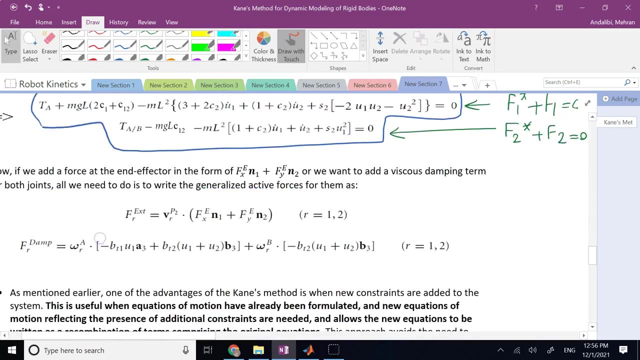 further and further up. this method is quite systematic and it is much easier to go, even compared to the lagrangian method. so it really shows its advantage, its advantages when the degrees of freedom go up or, as i said, when you have some constraints or external forces or some addition to the 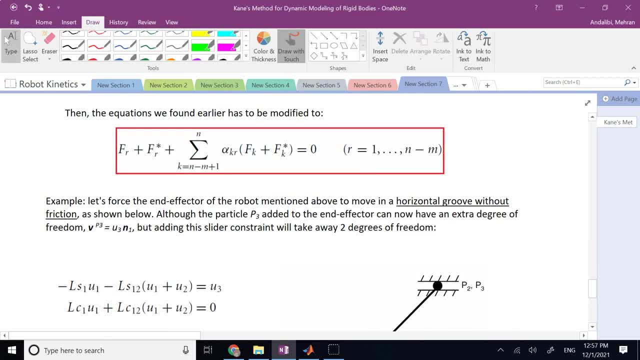 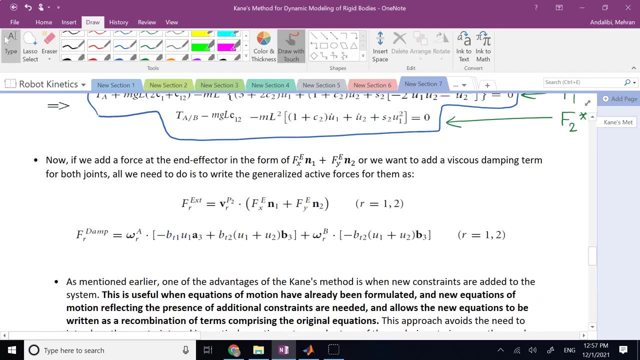 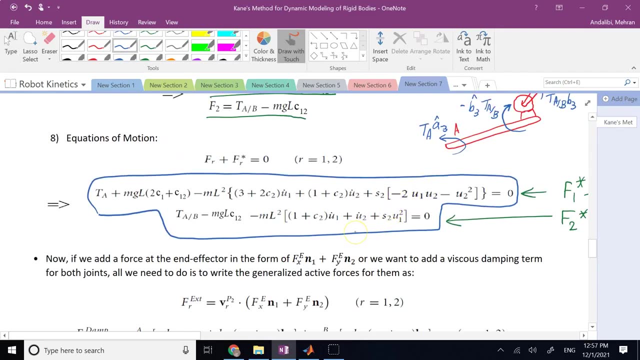 system and you do not want to start from scratch and re-derive everything. i'll show you in a minute. that's the case with this method: adding some stuff to the system- external extra forces, extra constraints and so on. we can still use whatever equation that we have, and 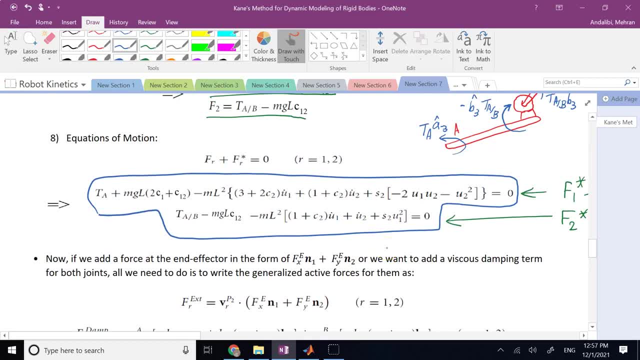 um, um, um, um, um. modify them a little bit and get the equations of motion for the new system, while with other methods it's not that easy. for many of them you have to redo a bunch of things or all from scratch. okay, so when it comes to complicated system, this: 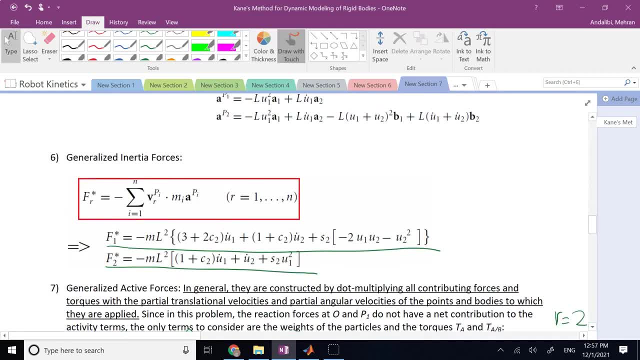 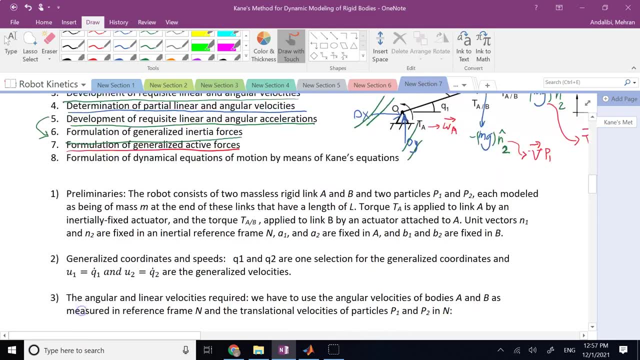 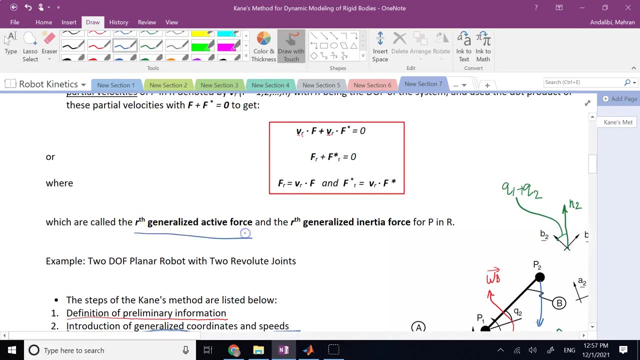 method can be the method of choice. the last thing, before i go to those, uh, extra advantages, is, if you remember, i told you that we call these frs, or fr stars, generalized active forces, and i said that these vr's or these omega rs, they don't have the 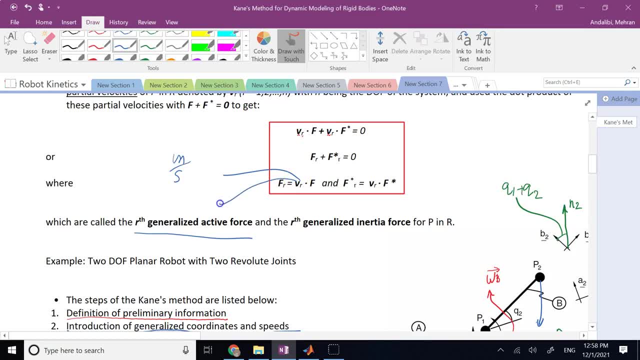 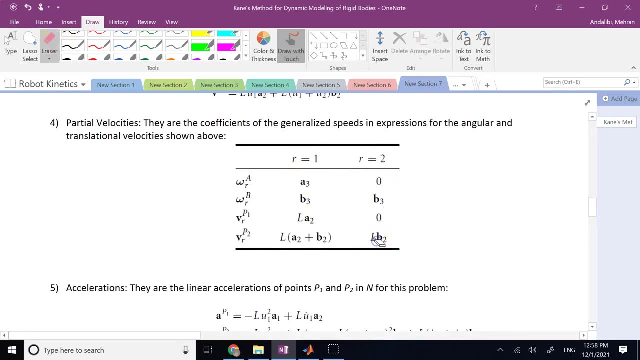 units of, let's say, meters per second, they have the unit of one. okay, that's why we call them generalized forces. we don't call them powers or activities anymore. why is that? you can see here from the table if you look at, uh, the units here. uh, for omegas, they are the units that we call the. 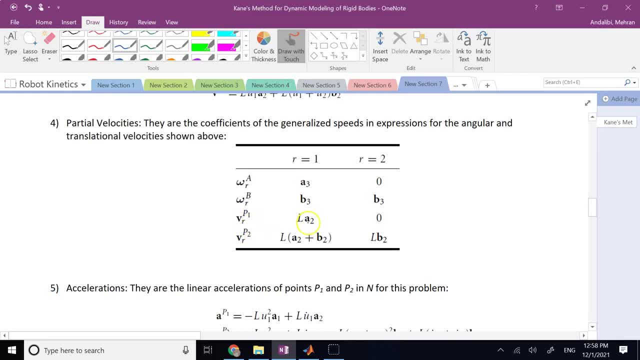 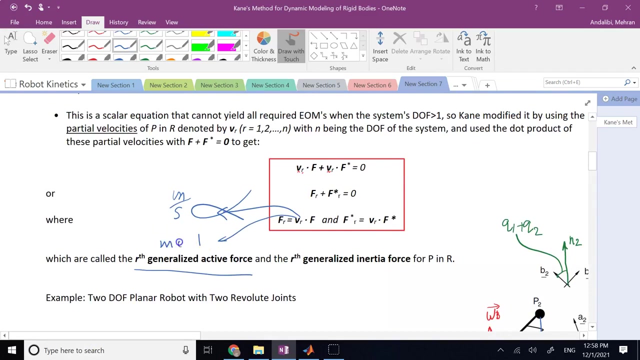 unit vectors, because the unit is one for v's, the unit is meters. right, because look here, it's just a unit vector. right for omegas and for um v's it is the unit of length. so you don't see the unit of time anywhere, anything divided by unit of time. so if i want to say more accurate, it's either meter. 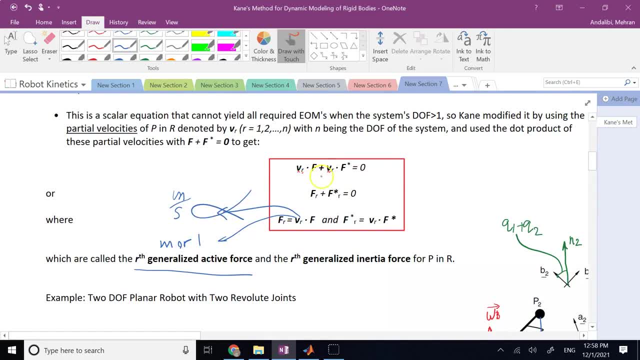 or like one okay. so you're not really multiplying meters per second to get a power or something. it's just like you are literally multiplying a force by a meter or you are multiplying a torque by a one. so the unit is going to be like newton meter, which is kind of like a um, a work really, or jewels, so we can say that really the 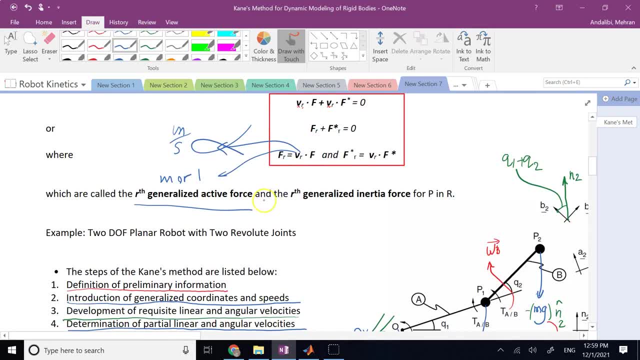 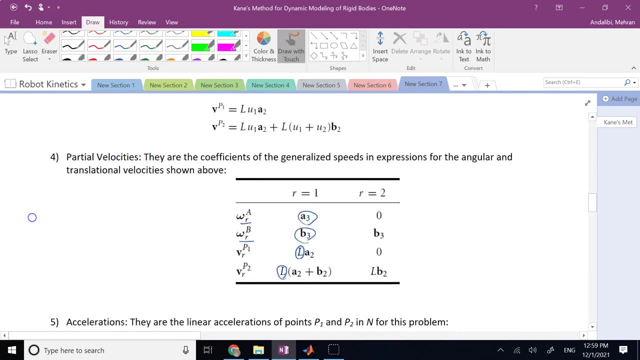 unit of these generalized forces is not even force and it's not power. it's kind of like jewels. the unit of them is the unit of work, really. that's why we call them active force or the force in action. right, the effect of force in action. so just keep that in. 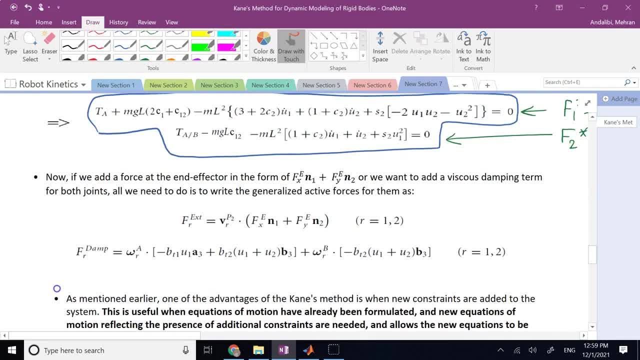 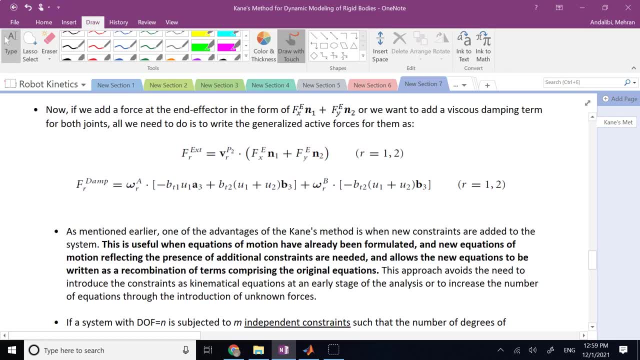 mind good. so now let's go ahead and talk about modifications. if you want to add something to the system, uh, what should you do to the equations you have already derived? so now let's consider that we have added a force at the end effector. what should we change? 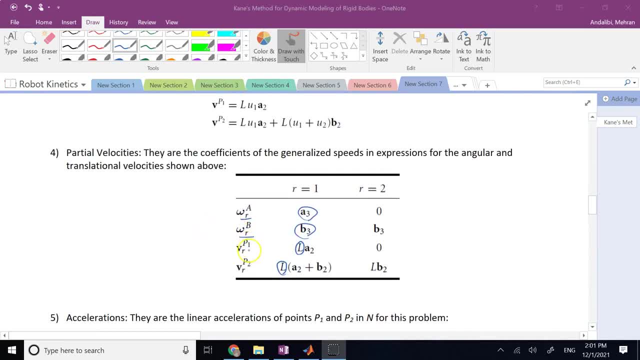 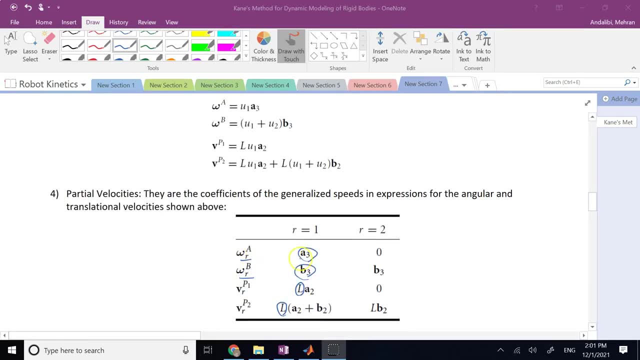 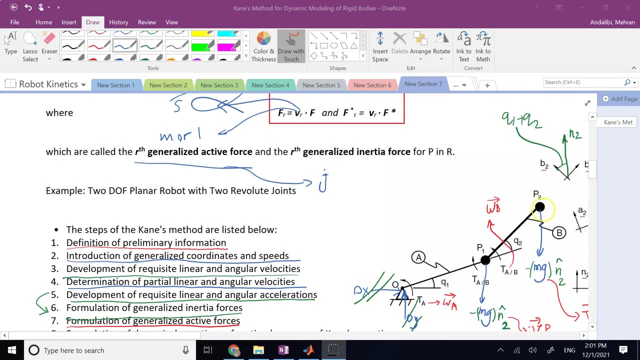 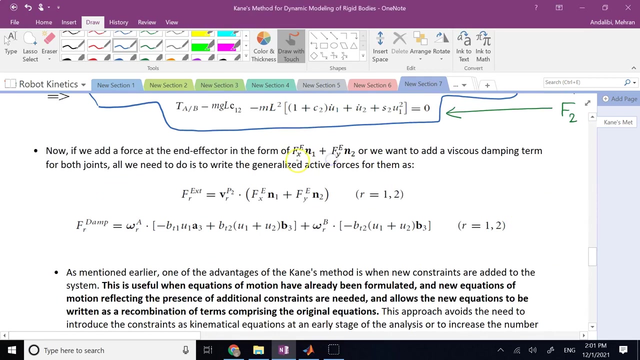 do we change any of our vr or omega r terms? absolutely not, especially because here the particle p2 is already at the end effector and i do not need to add any extra uh motion or velocity where that new force that i mentioned applying at the end effector, is happening. 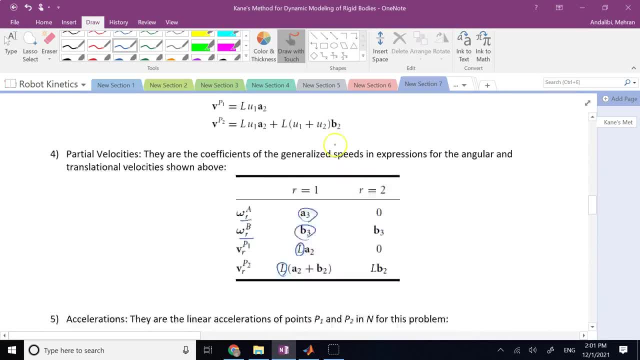 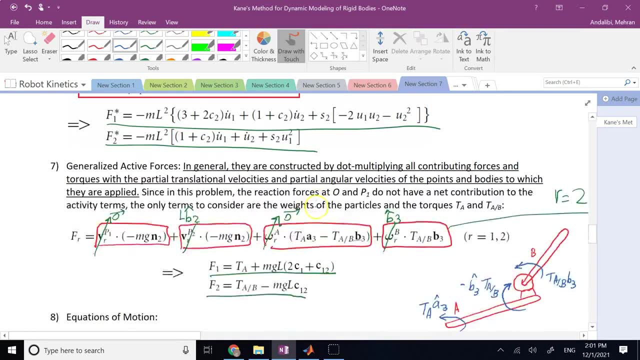 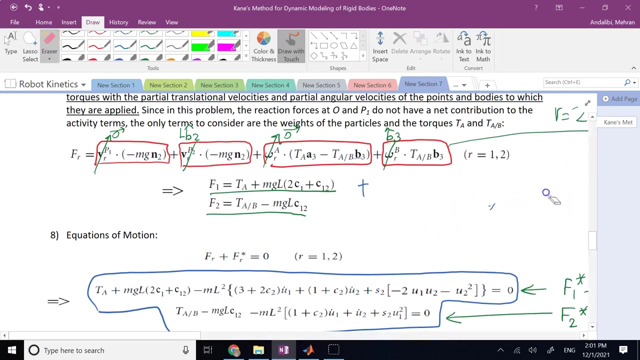 that area. the velocity of it is already considered in my vr and omega r terms, so i'm good. what about the inertial forces? no change. the only thing you need to change is the active forces, because now you have some extra term that you should add to your um active forces. now you have this new force right: fx n1 and fy n2. 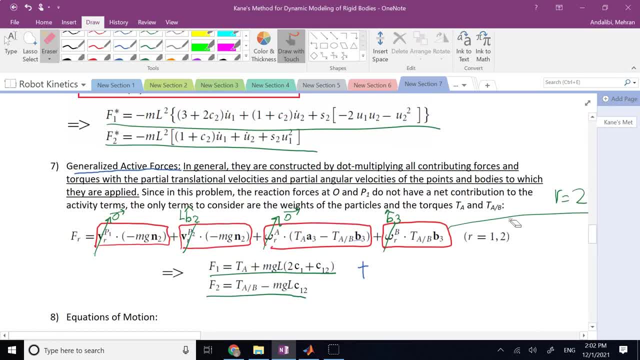 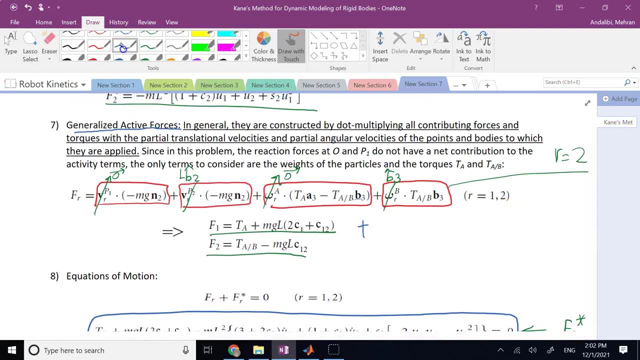 and that is applied to a place for which the motion is called vp2. so now you have to add what to it? you have to add, basically, this new force and dot producted by vr, p2, dot producted by this new force, fx, and one plus f y n. 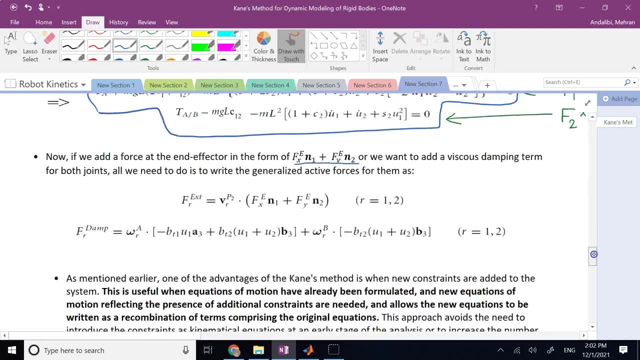 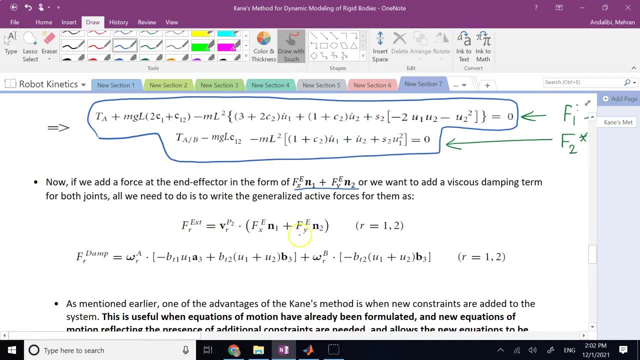 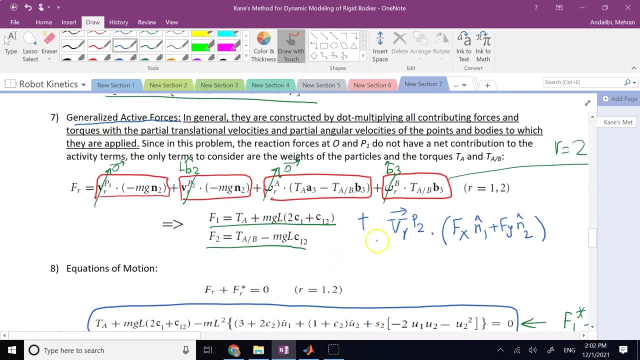 two. that's all you need to add and it's clearly mentioned here for you. so you plug r1, it gives you one term to be adding to the active force f1. so you're going to have some extra term added here. and uh, if you put r of 2, it gives you one term to add to what to r of 2, and that's all. it is everything. 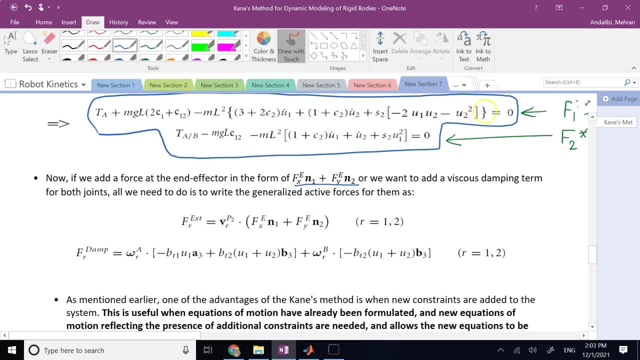 else is the same. you will get the same equation of motion plus some extra terms. you might say: what about if i have some viscous damping at the joints? can i add that? sure? what do i need to do again? those are active forces or torques, so we have to just modify. 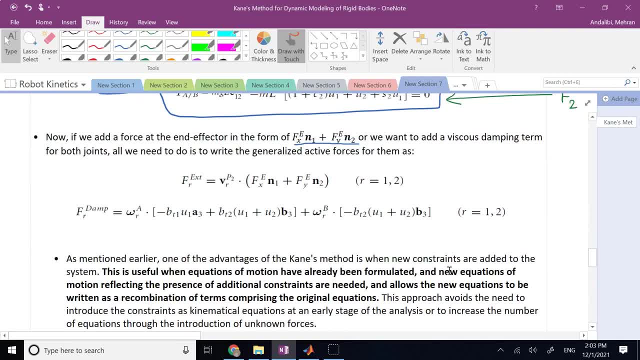 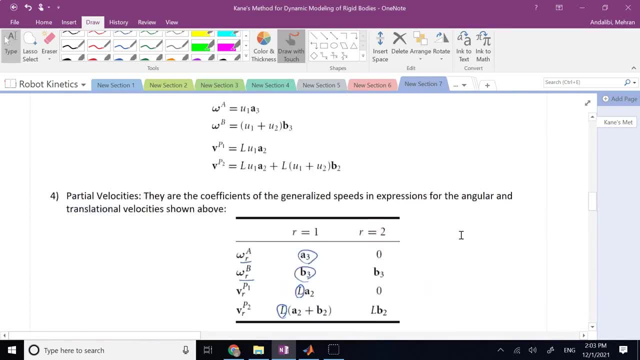 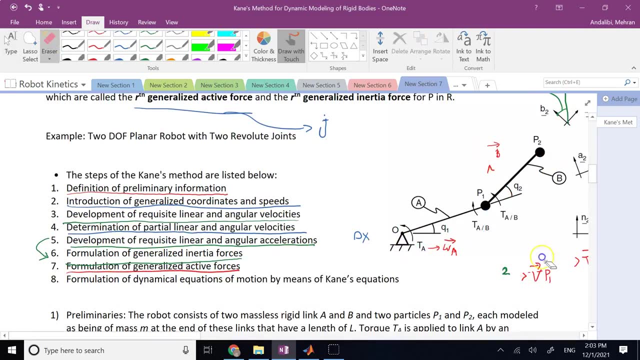 where those are happening. and guess what? one of them is like ta: it is affecting the first joint. one of them is like tab: it is affecting the second joint, correct? so if i want to show them here for you, the first viscous friction is happening here. the second one is happening here: 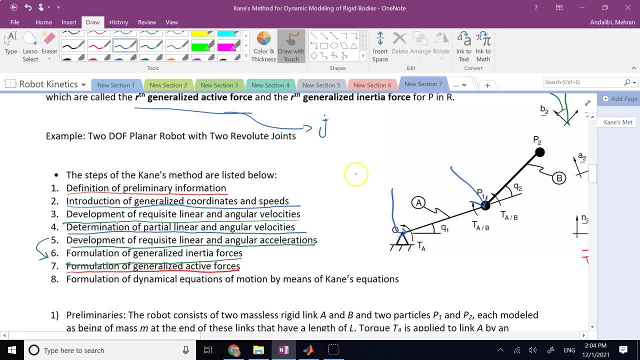 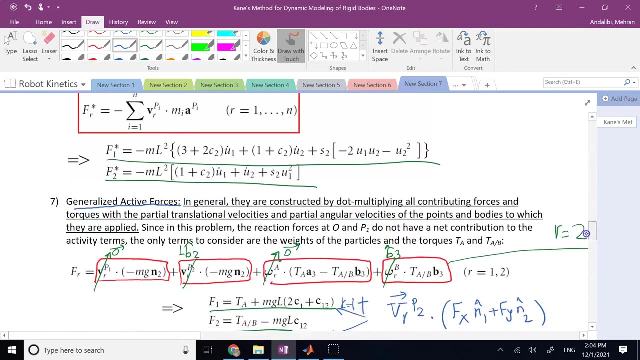 so the first one should be dot multiplied by omega r of a, whatever it is, and this one should be dot multiplied by omega r of b, because that's similar to the torque tab is going to rotate member b, that's all it is. and here we go and take a look at these terms. 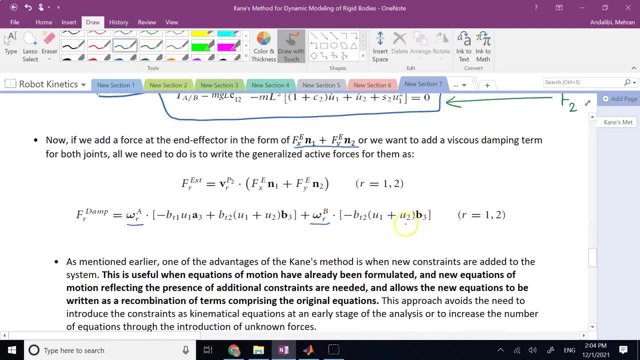 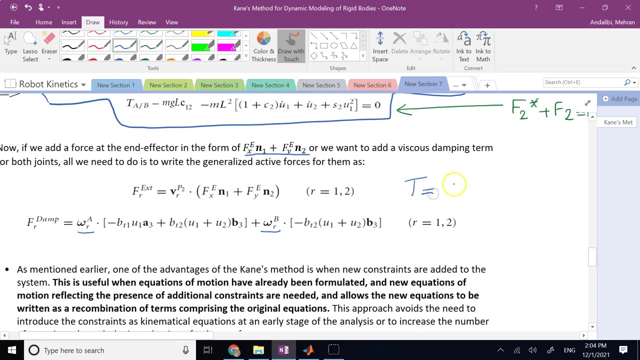 you clearly see what i said. now, what are they? let's say the um. what is the second viscous friction at the joint? well, if you remember, viscous friction is what the viscous friction at the joint is formulated by. t equals some coefficient b times the angular velocity at that joint, q dot. so this is the formula for. 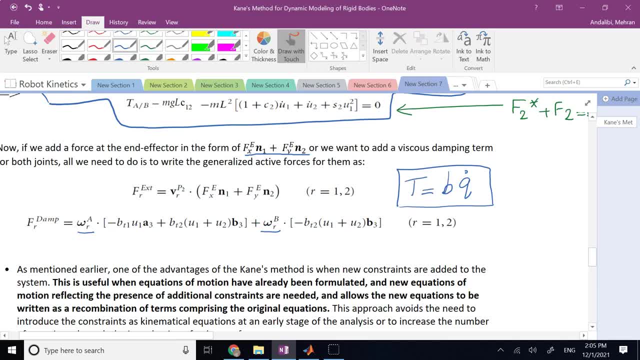 a viscous friction at a joint, a rotary joint. now, the second joint that i have, we know this- is its angular velocity: u1 plus u2, or q1 dot plus q2 dot times b3, correct, that's the uh q dot for the number two, and here you call the coefficient of viscous friction for it, you call it bt2. 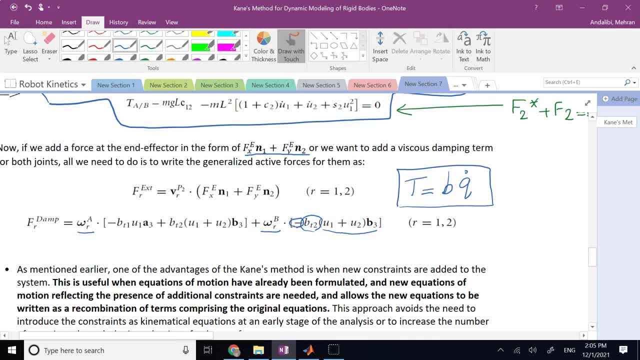 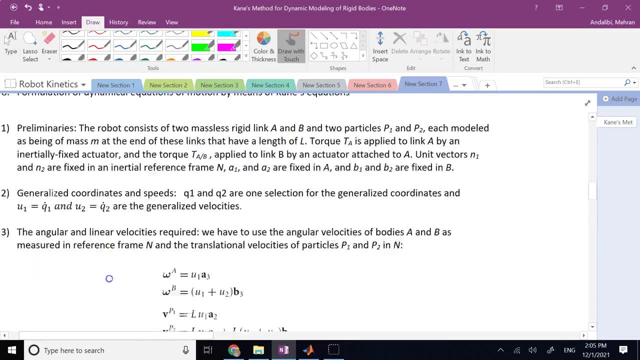 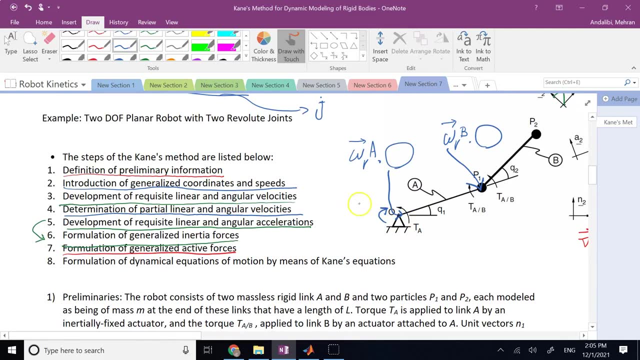 and it is a negative term. why negative? because it is opposing the direction of motion, right, or the way that the motion is happening. so if this is going this way, that damping viscous friction is like this: this is: you might call it t of b right, t of b1, and this guy you might call it t of b2. so, because they are opposing the 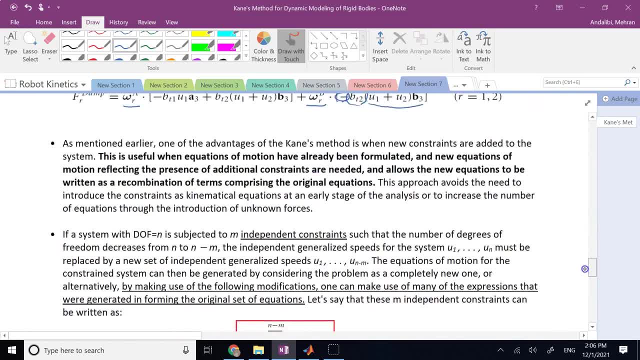 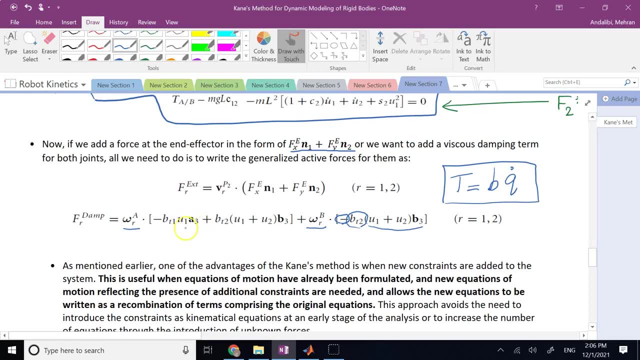 motion. you definitely want a negative sign, and that's again what you can see here. what about the first joint? well, the first joint, the angular velocities of it, is u1, a3, u1 is q1, dot the coefficient: at that point you call it BT, one with a. 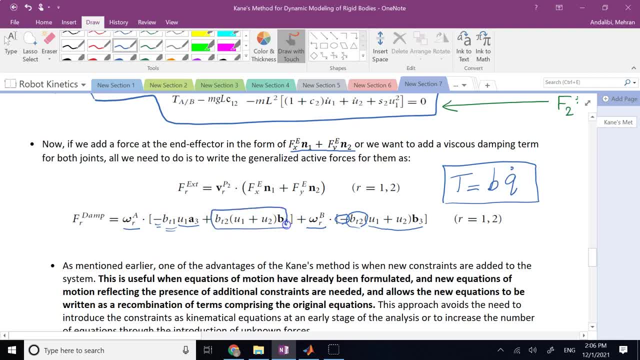 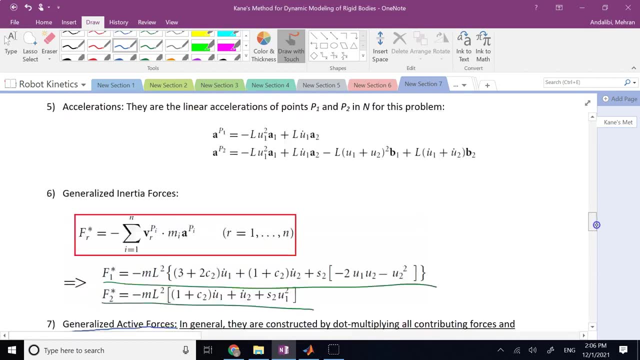 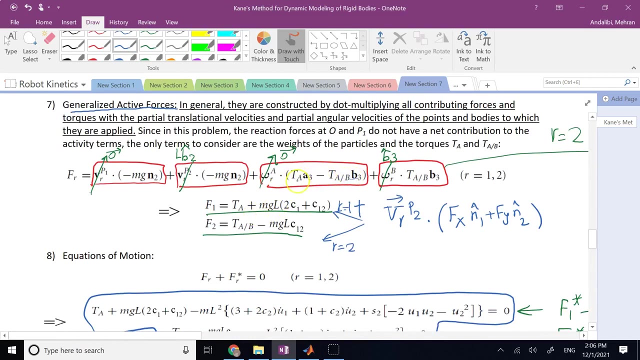 negative sign and you might say: what is this guy? and this guy is the same as this one on the right. but instead of negative it's positive. what is it? it's again action and reaction. if you remember here that we in a n negative TAB for the first member. why? because we said the motor is attached to. 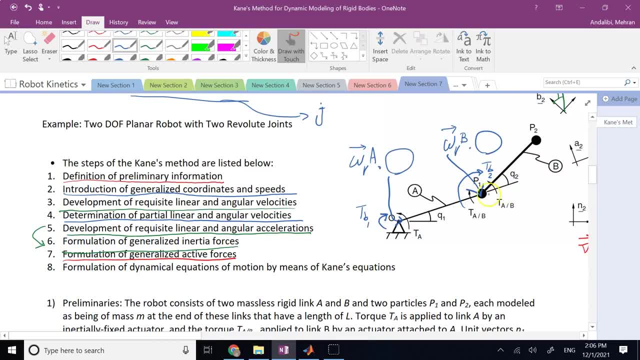 member one. so if you apply a TAB by motor to member B, reaction of that is applied back to what to member a. the same thing happens about this viscous friction. if this TB2 is applied on the shaft of motor or link of member B, then the reaction of that which is this way is going to be applied back to the motor. 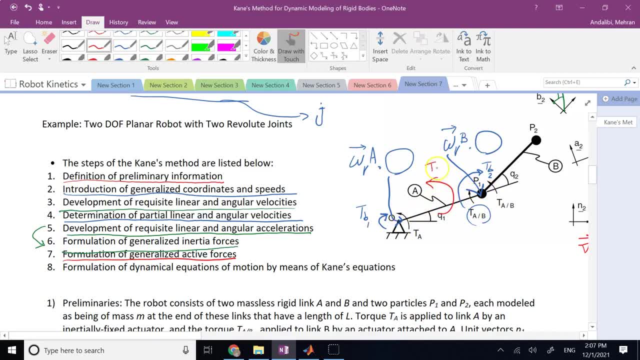 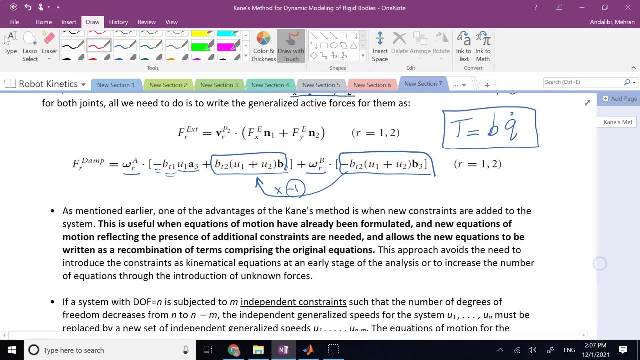 and motor is attached to member a, so it is going to be applied to member a, so it is going to be this minus that, okay, the total negative or the total momentum due to viscous friction, and that's what you can see here. so it is quite clear that if I want to, 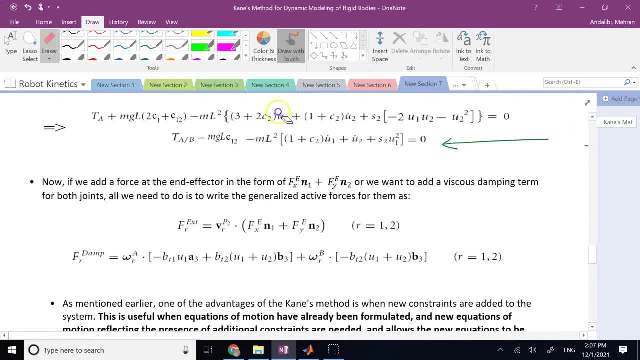 add a viscous damping, or if I want to add, let's say, a force at the end effector, or so on, all I need to do is to add one or several terms to what? to my active forces? because my inertial forces are the same, and in this case, 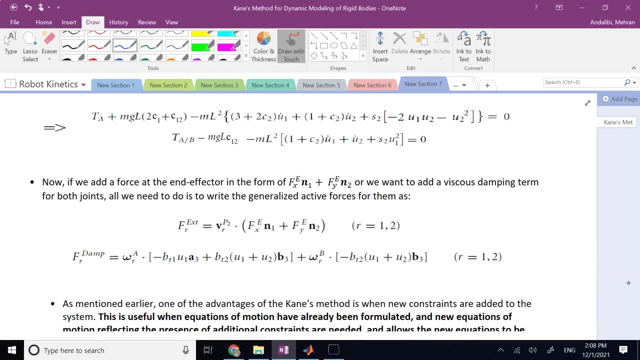 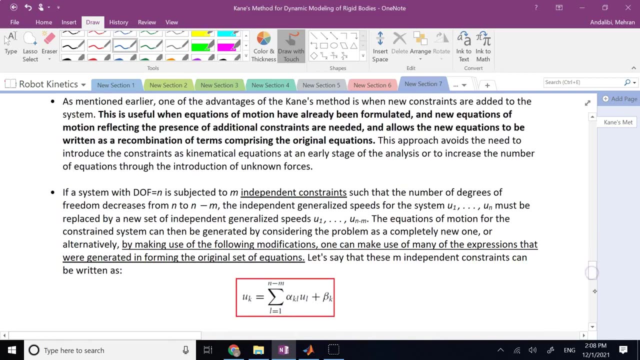 as long as I'm not adding a degree of freedom or anything, or applying force or torques to a new location, I do not need to add anything to my partial velocities. that's all it is now. sometimes you do have to add something to your degrees of. 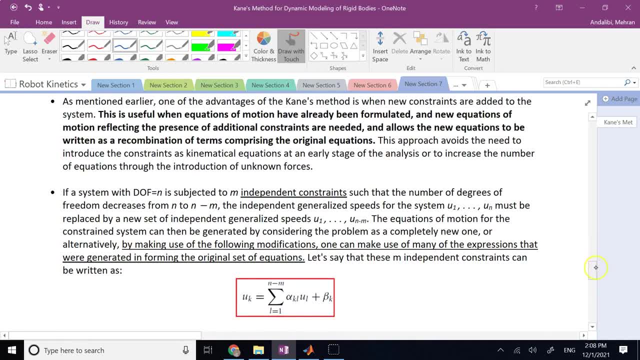 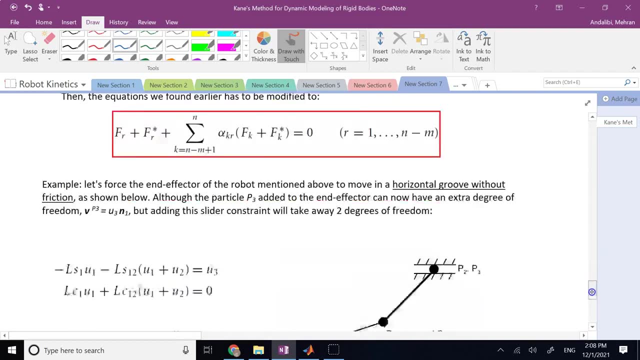 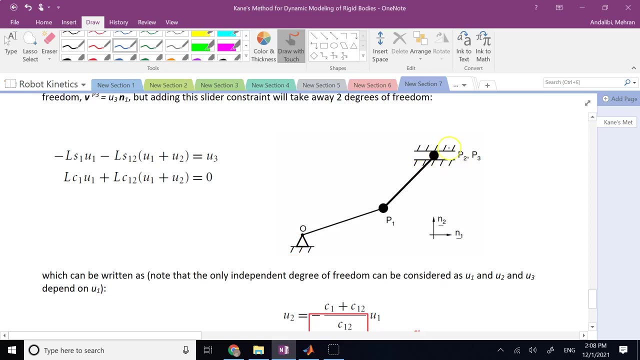 freedom or to your partial velocities. sometimes your degrees of freedom are changed because you are applying a constraint. okay, and again, I'm not going to have to add any more things to my partial velocities. okay, now we are at a time when you have the same gained arms, and this method is well capable of. 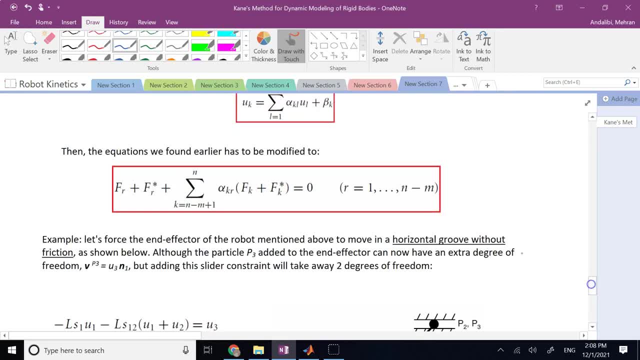 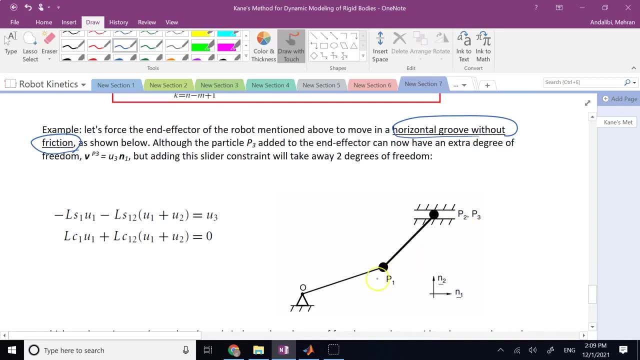 handling this? let's say, for example, here you have the same two degree of freedom planner arm that we talked about, but now you limit the end effector, or point P, to to move inside a horizontal groove, and this horizontal groove has no friction here. just to make it a little bit easier, how do you change your equations of motion? or a general? 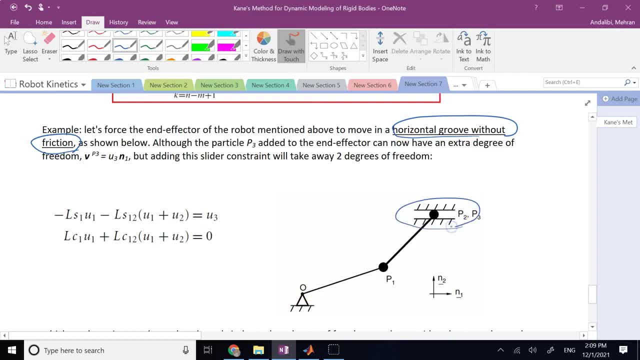 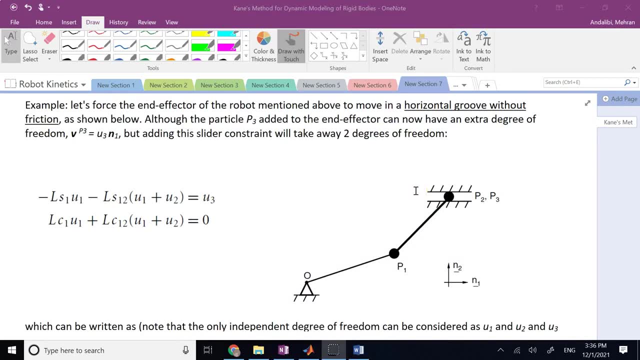 or adjust your equations of motion to accommodate for this extra constraint that you have right. So what you can do here is to add an extra particle- P3, right where P2 is okay, Because P3 is also the end effector. 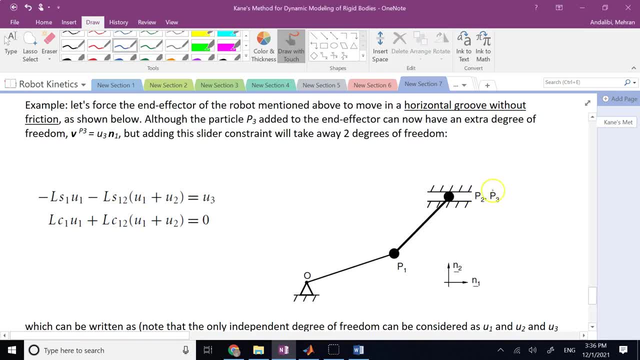 So there is an overlap right, There are coincidences between P2 and P3.. Okay, and P3, adding P3, will add one extra degree of freedom to the system, So P3, with respect to P2, can move horizontally this way, okay. 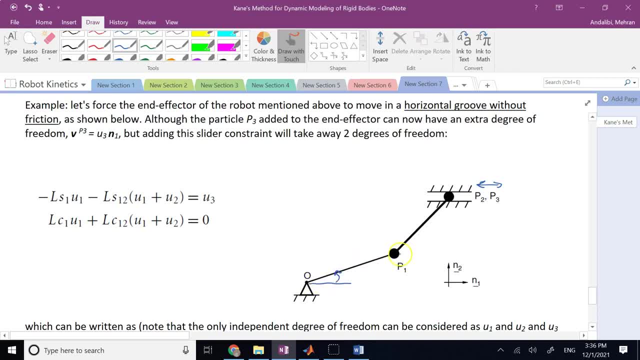 So now you have this degree of freedom. you have this degree of freedom and you have that degree of freedom Q1,, Q2, and that's whatever you want to call it- D3 maybe- But now you have two constraints. 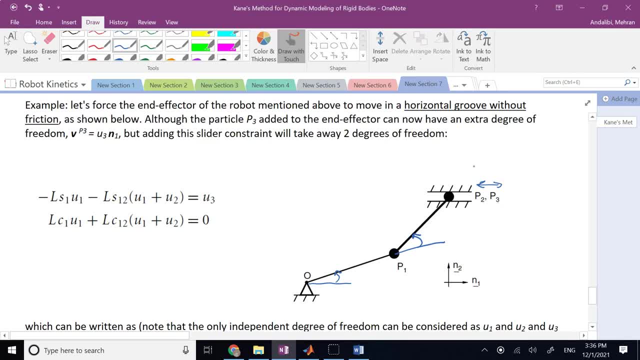 Two constraints added to your system. What are they? Well, here, the velocity of this point, P3, can only be in the horizontal direction, as we said, It cannot have a vertical velocity. What is velocity of P3?? Velocity of P3 is the same as velocity of P2.. 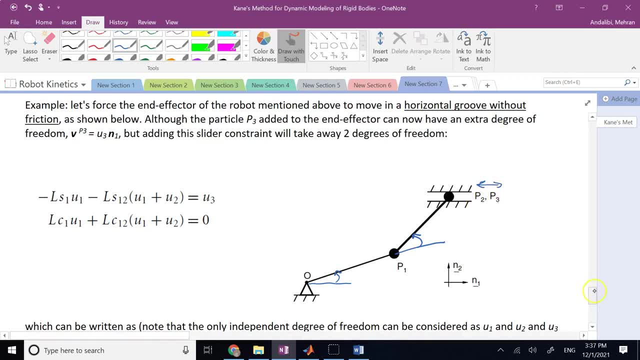 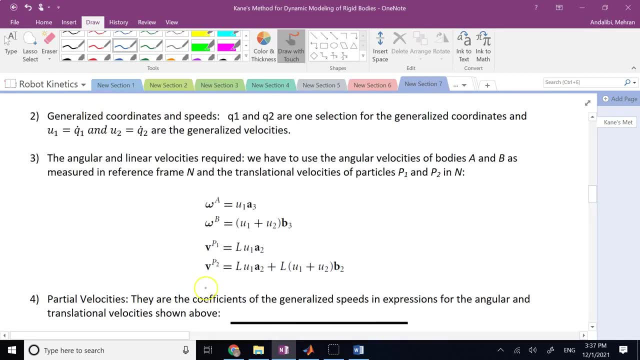 And what is velocity of P2?? So we had the velocity of P2 earlier, right, I assume we calculated that somewhere here. But now we have to dot product this: align X and Y directions or N1 and N2, to get the horizontal and vertical components. 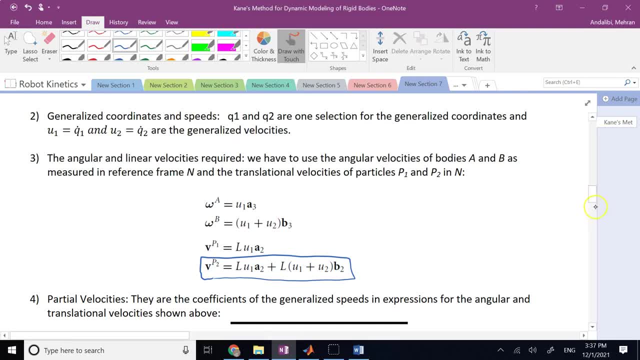 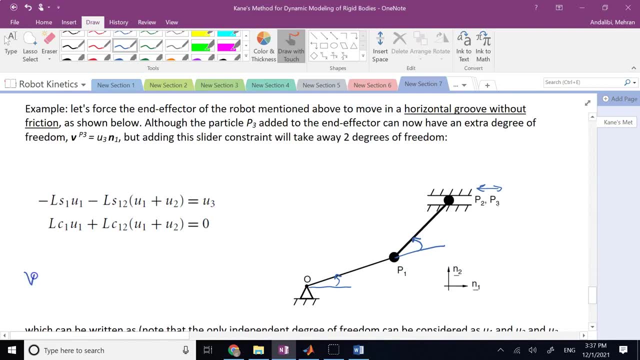 Because the constraints I have applied are, with respect to the inertial frame, okay, About N1 and N2.. Okay, So what I really need is V of P2 dot N2, vertical direction, the vertical component of velocity of P2, which is going to be exactly this guy: L1, C1, U1, plus L1, C1,, 2, U1, plus U2.. 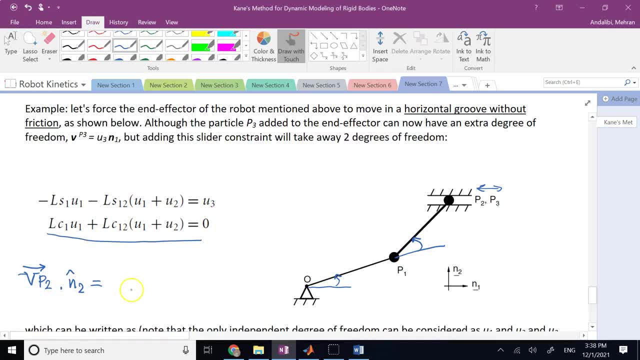 That has to be zero And that is not very hard to see, because Your V of P2,, if you remember it was L, U1, A2, and then plus L times U1, plus U2, B2. So you dot product it with N2.. 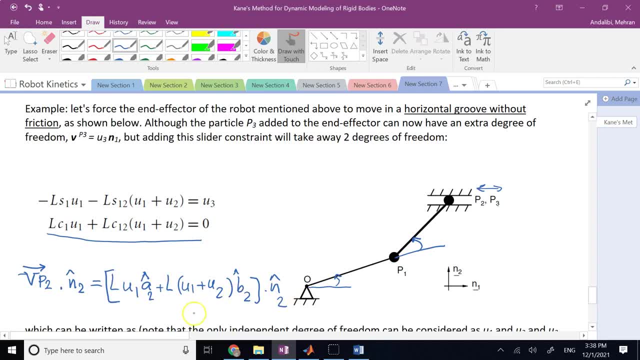 And so here you have A2 dot product with N2 and B2 dot product with N2.. And remember: A2 is this direction and N2 is this direction. So the angle between them is this: Q1.. So correct. 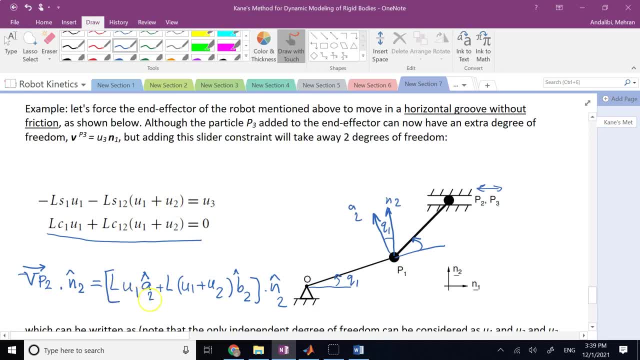 So you should be getting L? U1, and then A2, dot N2,, as I said, is cosine of theta 1 or cosine of Q1, which we show by C1.. So that's this term, And the next term is L, U1 plus U2.. 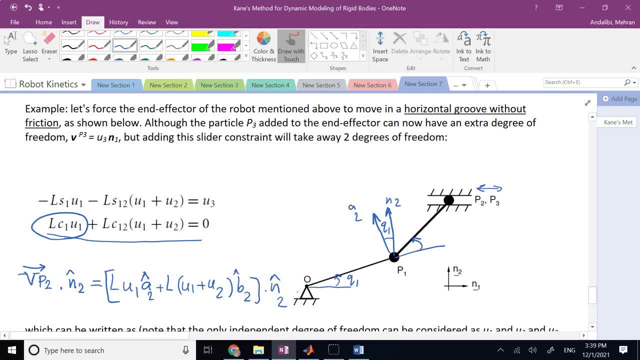 L2 times B2, dot N2.. B2- here is this vector which is perpendicular to member number 2. And this angle is Q2.. So the angle between B2 and N2 is Q1 plus Q2.. So that dot product is going to become cosine of Q1 plus Q2.. 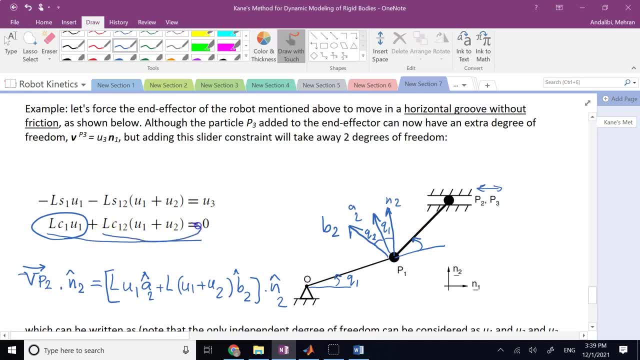 Or C12, which you can see here. So this is your second term. So adding these together should be 0.. And that gives you the bottom equation, the first constraint that you have. The other constraint is now, if you call the generalized speed associated with this horizontal motion, U3. 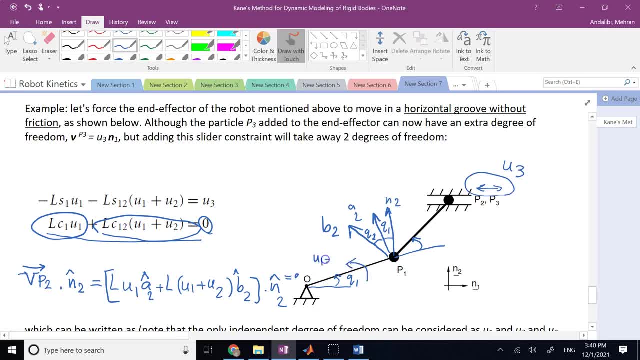 Remember you had U1, which was Q1 dot. You had U2, which was Q2 dot, And now if you call this maybe Q3,, this horizontal motion, then U3 is going to be Q3 dot. So it says the horizontal component of VP2 should be equal to U3.. 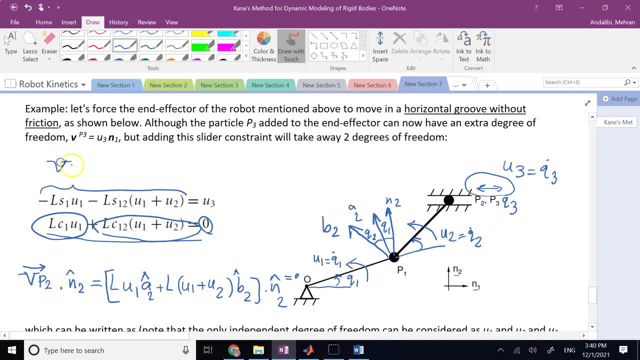 And this is exactly that. This is V of P2.. This is V of P2, dot N1.. This thing should be equal to U3.. So you see, I added one extra degree of freedom to the system. Q3 now. 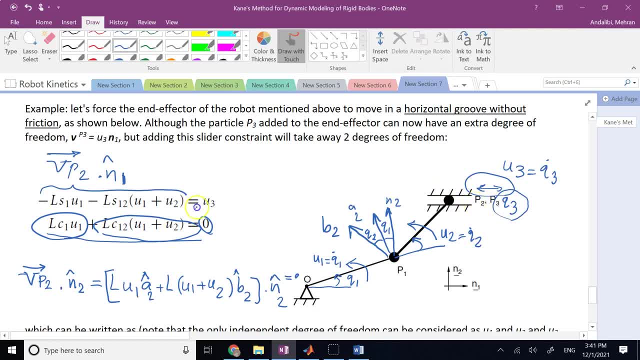 This is the horizontal motion between 2 and 3.. But it came with two extra constraints, So my degree of freedom of the system that was 2 originally. I added 1 to it And then I subtracted two constraints, So now I really only have one degree of freedom left. 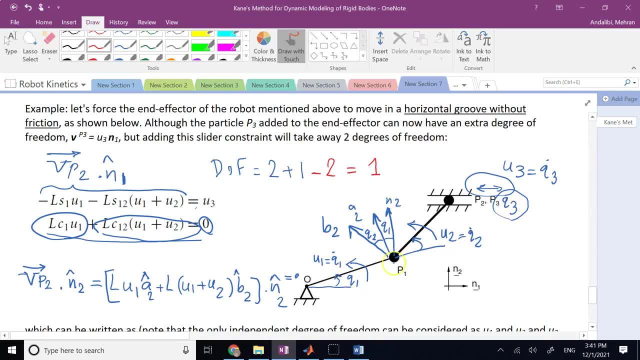 I have three generalized coordinates, but one of them is really independent. The two other depend on this degree of freedom And the question is: how Can I relate, let's say, two of these degrees of freedom, let's say Q2 and Q3 to Q1, or their velocities together? 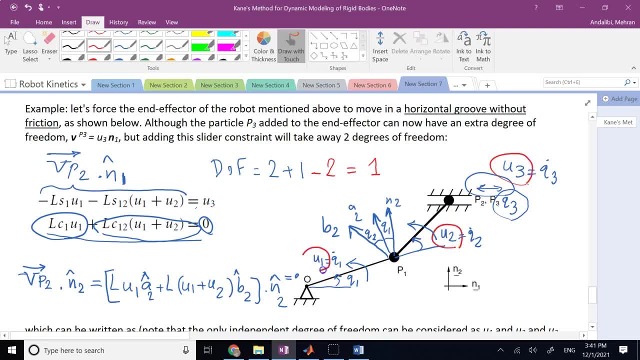 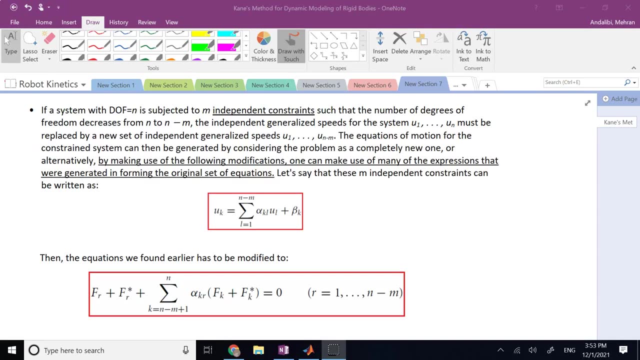 For example, can I relate U3 and U2 somehow to U1?? If I can do that, then incorporating these constraints into my equations of motion is not going to be necessarily a hard thing. So here we answer the question in general, that if you have N degrees of freedom and you add M constraints to the system, 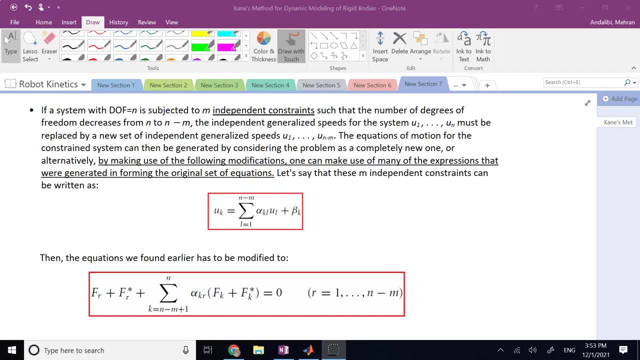 then you really need N minus M degrees of freedom in general, Not just Q2.. Not always It is easy to just find some based on some others and replace from the constraints. Sometimes the constraints are non-holonomic. Sometimes they are holonomic but highly nonlinear. 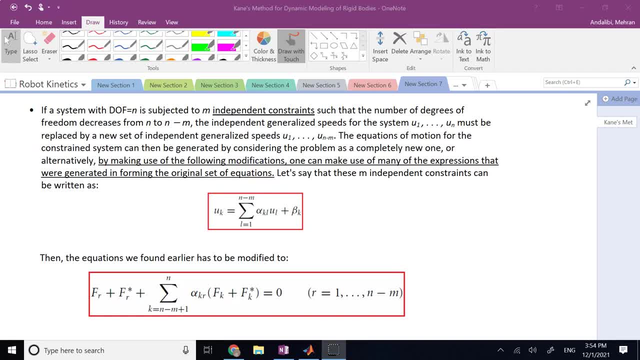 So the better way and the easier way to incorporate it is if you can basically work on the generalized speeds instead of generalized coordinates. Right, If you work on generalized speeds, U1 all the way to UN minus M, the N minus M, let's say use that. you might think they are the independent, basically generalized speeds. 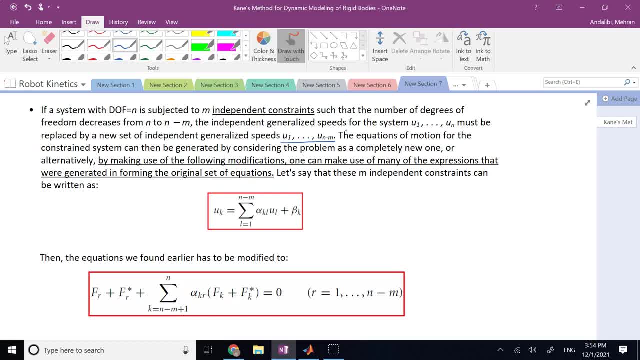 If you can find any other generalized speed in the system outside 1 to N minus M, which is basically from N minus M plus 1 all the way to N. If you can find all of those based on these other generalized speeds in a linear fashion. 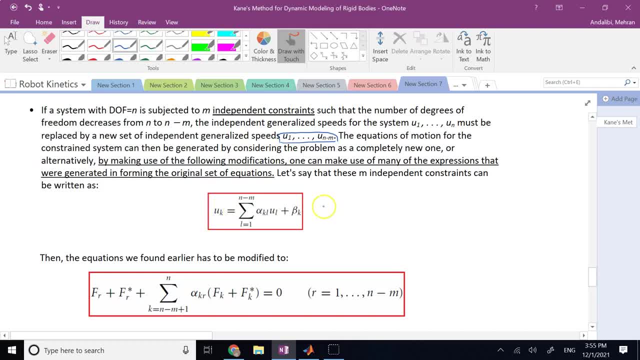 So UK here, where K can be any number from N minus M plus 1, all the way to N, You can find any UK based on the linear combination of those other U's which are from 1 to N minus M as well. So UK can be any number from N minus M plus 1 all the way to N, all the way to N. 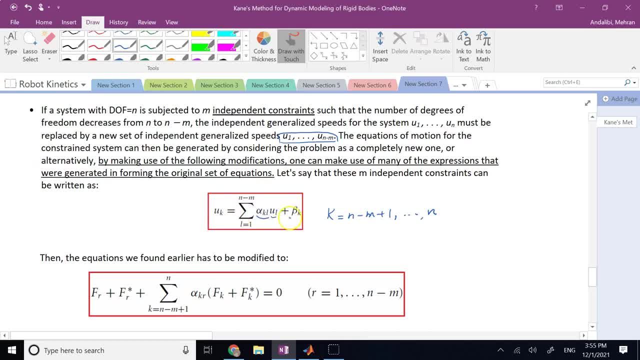 What As alpha, some alpha times, those u's plus some beta in general, So a linear combination of those u's plus, at most, a constant, If you can establish such a linear relation between those redundant generalized speeds and these independent ones that you want to consider for the equations of motion. 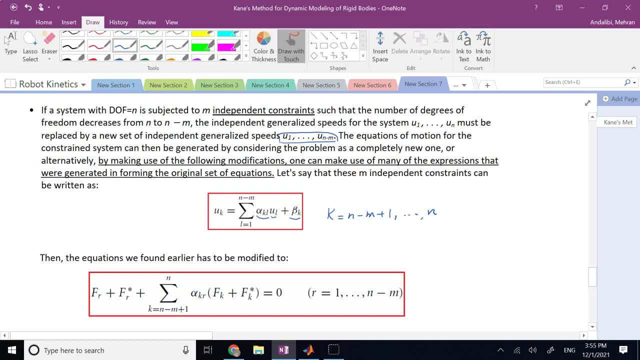 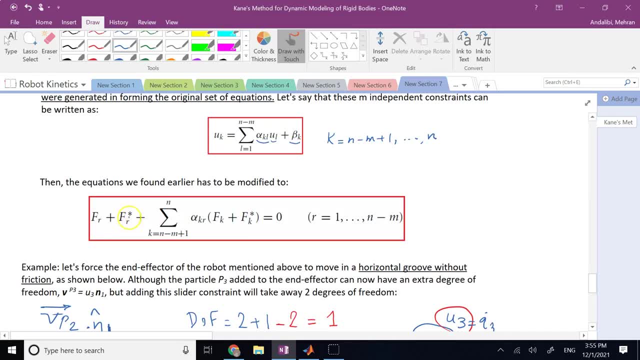 if you can do such a thing and determine these alphas and betas, then all you need to do to the previous equations of motion that were fr plus fr- star was equal to zero- is now you have to add a summation to it, And the summation is this: 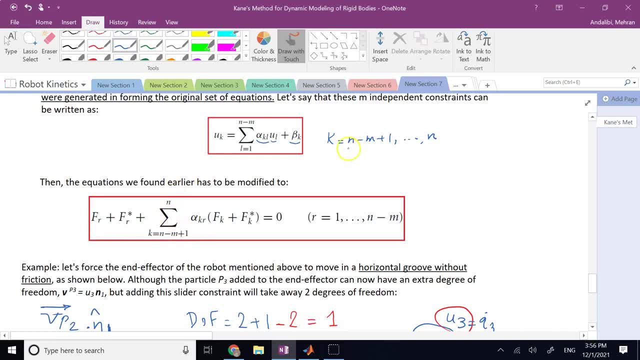 K goes from n minus m plus one to n. as I said, this area over those extra or redundant degrees of freedom, Of what? Alpha kr, The same alphas that you found, times fk plus f, star k, and then set it equal to zero. 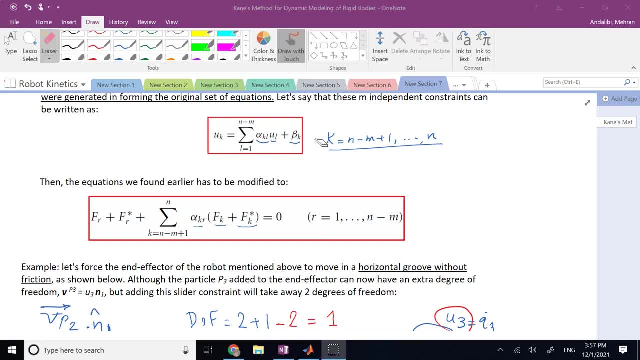 The constants beta of those relations do not play any role in the modified equations, And this is very advantageous because you have already this one set up. All you need is to find the summation terms, find these alphas, Of course. first you have to form this set of equations. 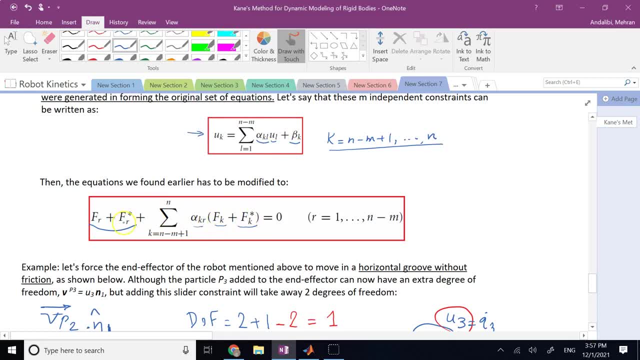 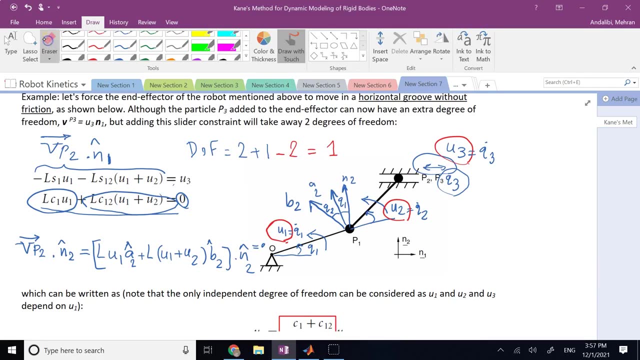 Find it, The alphas, and then add the summation to your previous set of equations and get what gets your new set of equations. For example, let me explain that with the example. if we go and look at this two degree of freedom plan or robot that we have, 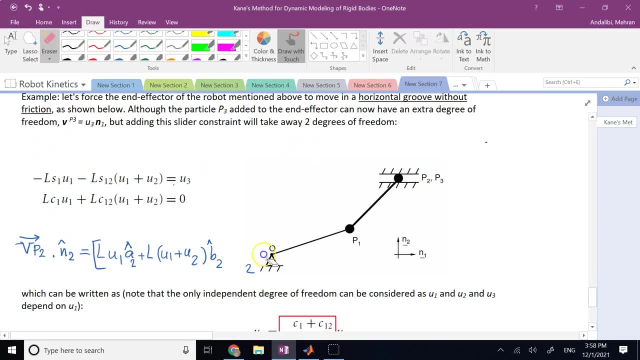 We just found that we can add this extra degree of freedom or this generalized speed, This extra generalized speed, You three to the system Q three or you three here, And that comes with two extra constraints right now. from these constraints we can easily find that two redundant generalized speed based on another one. 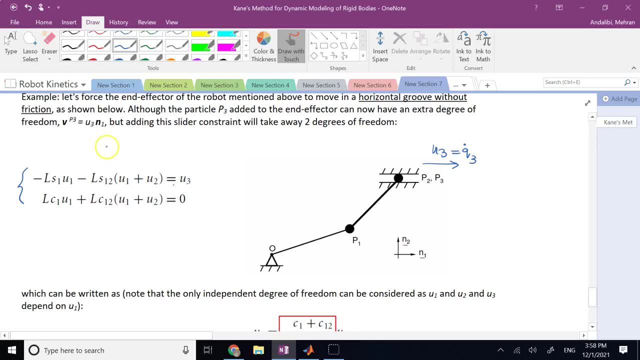 So here you're in. as I said, is what? and was two, But now you have one extra degree of freedom, So your end becomes three, but you have two constraints here, correct? Therefore, you really need one of these generalized speed to keep. 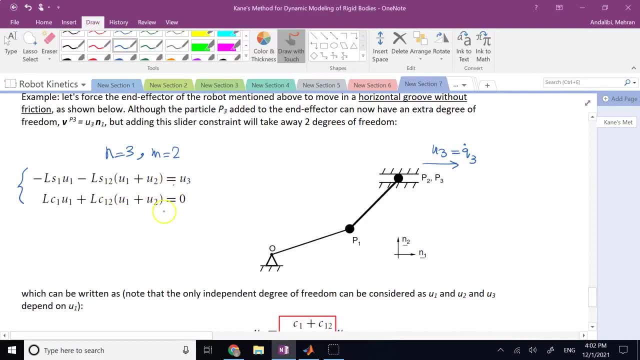 And you can basically determine the two others based on that. So in here, if I want to keep you one, then I want to determine you two and you three based on you one. How do I do that? Well, from the bottom one. it's very easy. 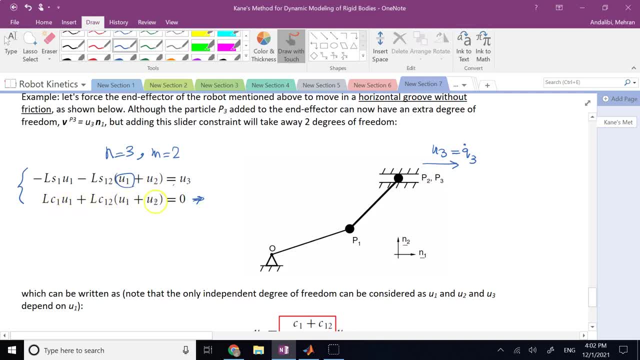 To see that l c one u one plus l c one two u one is l c one two u two. So you two can be written as: basically, if you eliminate the l's is going to be negative c one, negative c one two divided by c one two. 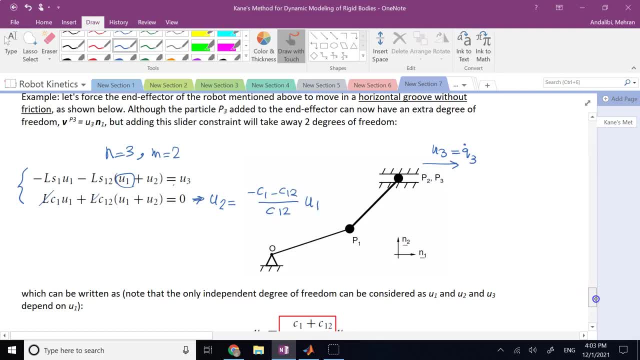 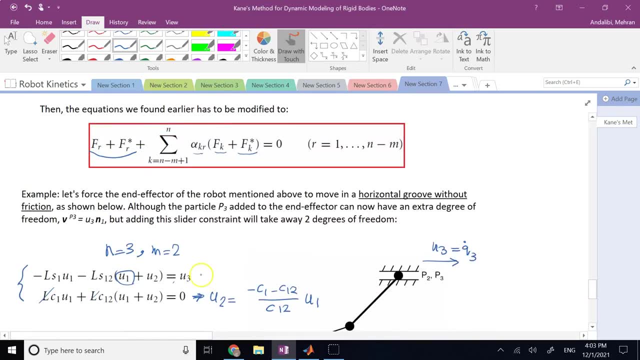 The whole thing times you one right, And that's what you can see down here, And from the bottom one, also top one. If you want, you can also find you three. So from here you're you three is gonna be a relation between you one and you two. 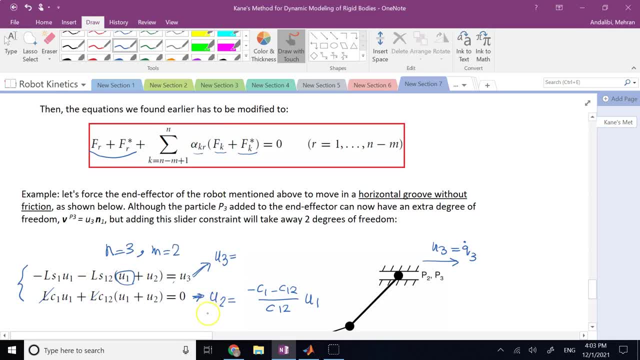 And from here you can really replace your you two relation that you had up here, And if you do that, then your U three. Yeah, Yeah, So you two is going to be really s one plus s one, two times you one, right, and then minus s one, two, you two, but you two. is this guy here so you can replace it? 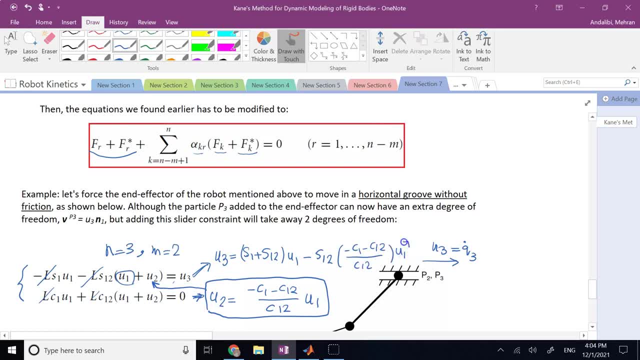 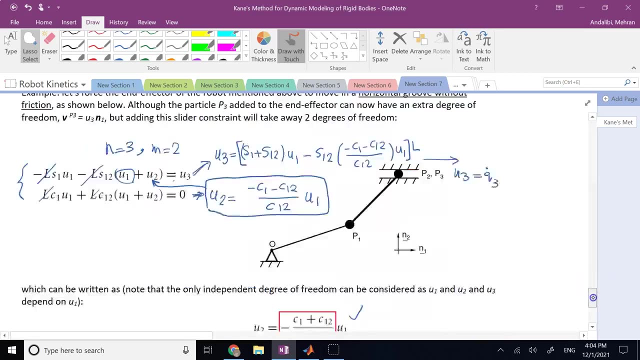 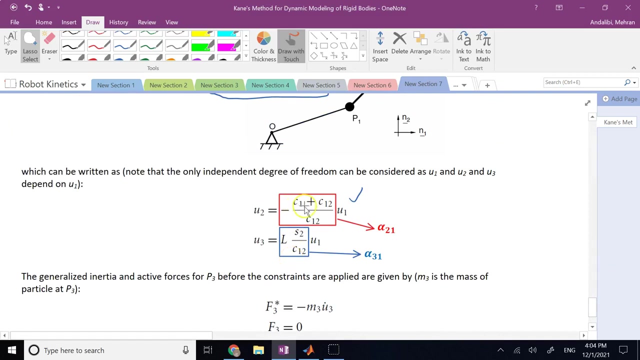 Then multiply the whole thing by l Right And if you simplify that, that should give you a relation between what between you two and you three and you one, and this is the simplified version of that. if you do a little bit of algebra, So you two and you three can now both be found as in 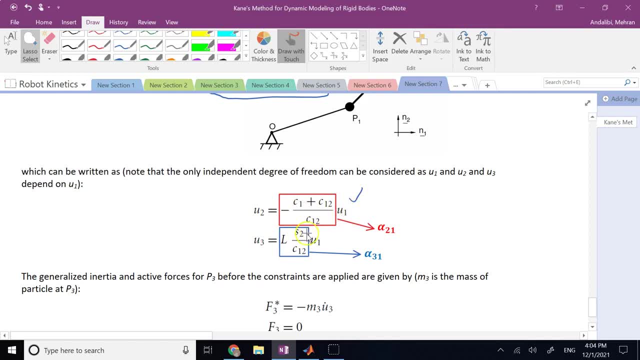 Linear relation of what of the other use that are independent. As I said, in this case, since N minus M, the number of required really degrees of freedom is one. All you need to keep is you one, So you have to find all other use based on you one. 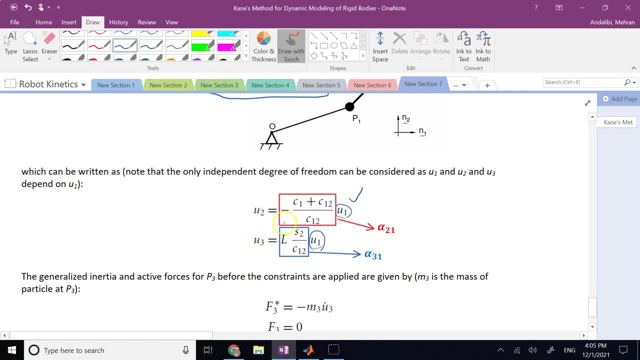 And we did that, And the relation that we found, your linear relations. When I say linear, it doesn't mean these coefficients that we call alpha here, Alpha two one or alpha three one. They are necessarily constant numbers. No, they can be, these alphas. 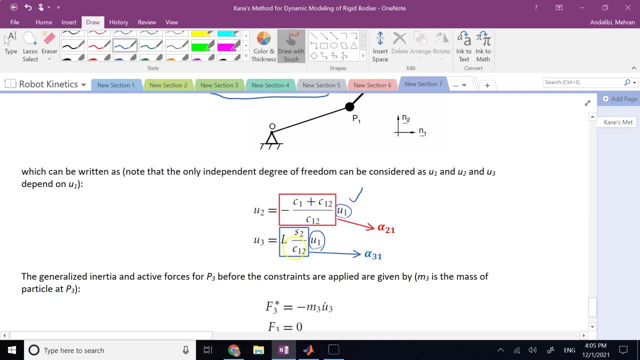 What functions of the angles? and you see they are. They are functions of cosine or sine of the angles. So this alpha two, one, is really a function of vector Q. The same thing with alpha Three. Okay, They are not constant. Even if you had a constant term- beta- you had some beta. 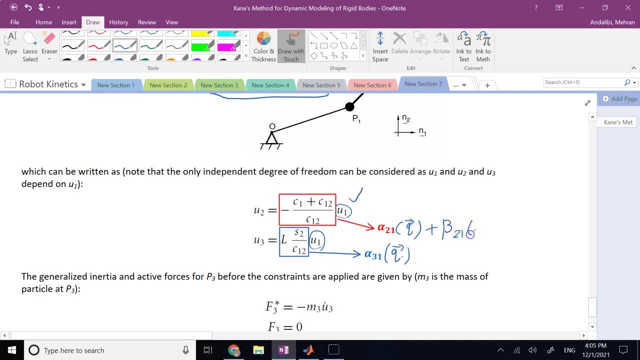 Let's say here Right Beta Two, one That could have also been a function of Q. So when we say constant, it doesn't mean really a constant number, It means it does not The alpha or beta does not depend on you. 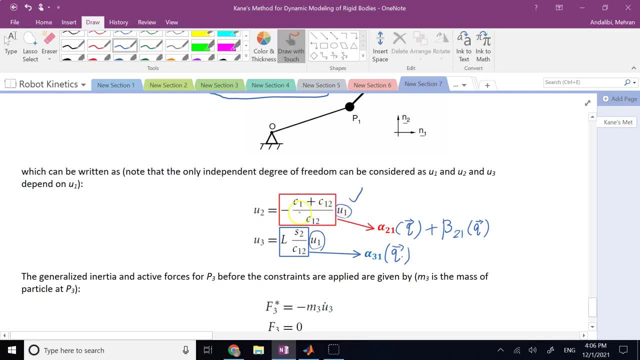 So the relation is linear in terms of use, not in terms of the cues. Okay, Now, in this case there is no beta, So all you have is just alpha two, one which is this term in the box, and alpha three, one which is the other term in the box. 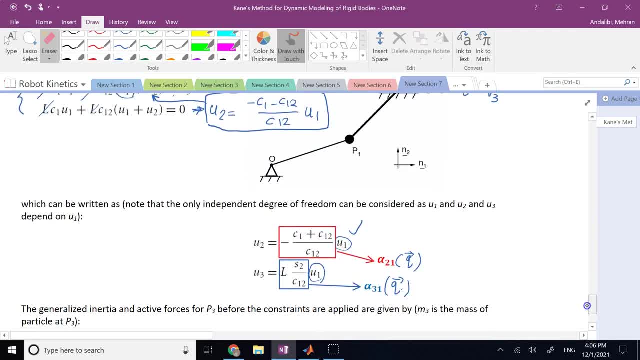 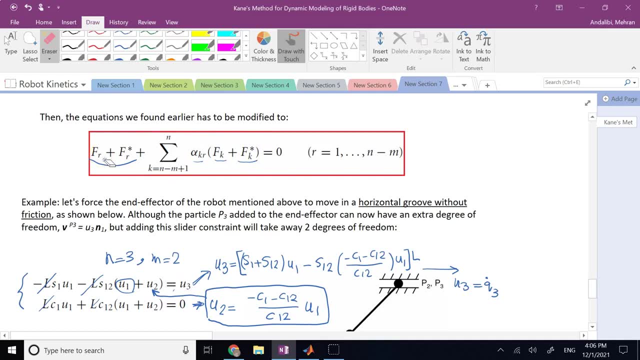 So keep that in mind. Now, if that is the case, I want to add this summation term for myself to my previous equations and see how that will change my equations. And the thing is this: This time your R goes from one to N minus M. 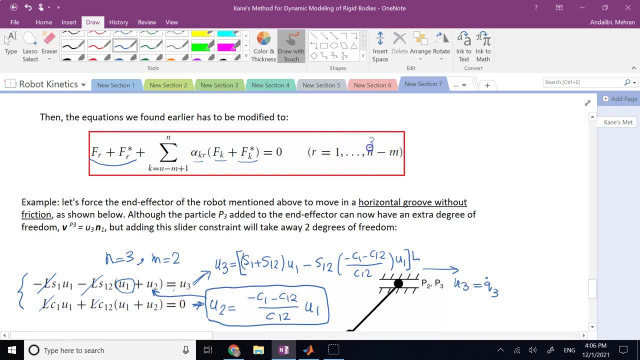 It doesn't go one to N, goes one to N minus M, and N is three, M is two, So it becomes one. So the only real R value that you can choose here is one. There will be no two. There will be no F two or F star two. 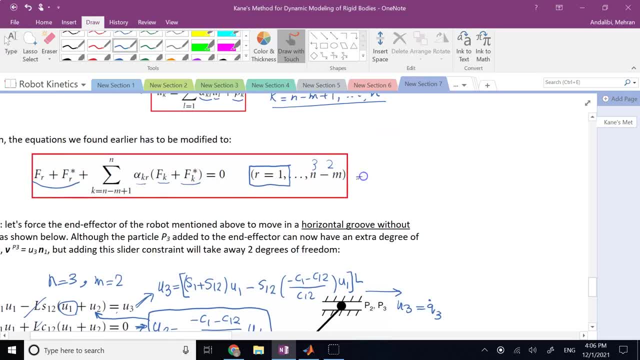 There is only one. So what's going to happen to this equation? It becomes F one plus F one star. The two terms that we already have calculated plus Summation of K goes from N minus M plus one to N. N is three here. 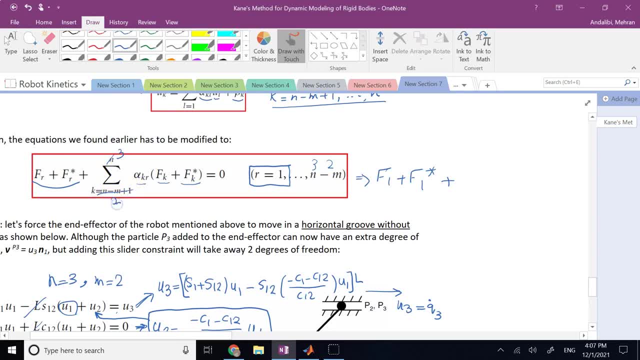 K N minus M plus one is two, So K goes from two to three of this. So it is going to become what? Alpha of K? K when is two? It's going to be alpha two. one times what F of two plus F, star of two. 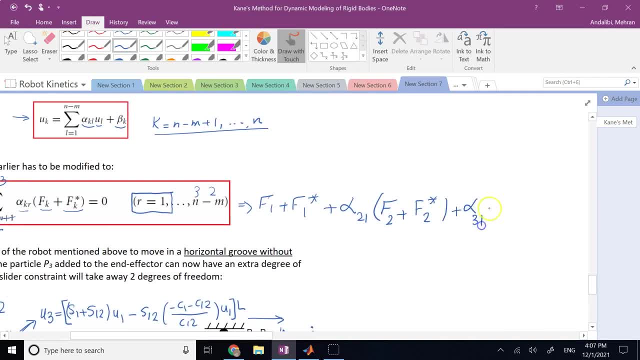 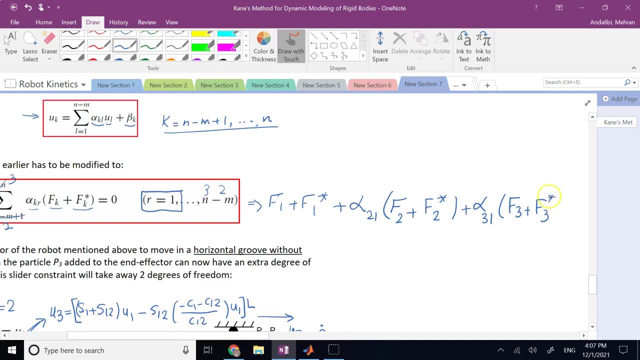 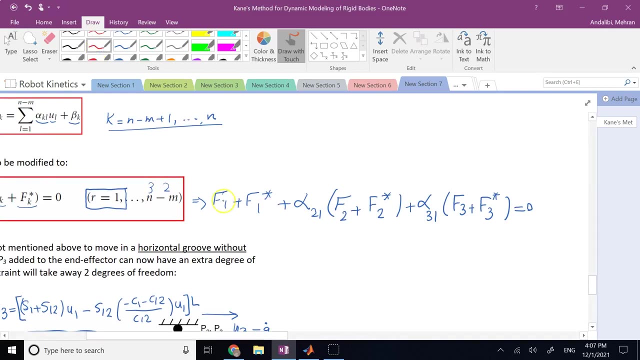 And then K becomes three. It becomes alpha three one, F three. minus F three star or plus F three star. This whole thing becomes three. Okay, It becomes equal to zero. Now, in the previous scenario I have already calculated for you F one and F star one F. 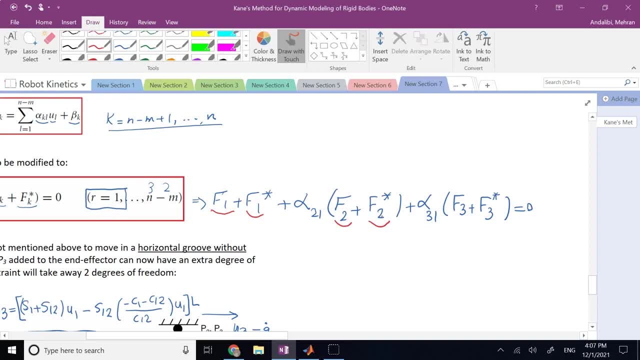 two and F star two. So I don't need to recalculate them. Alpha one and alpha two, I just calculated for you based on the constraint. The only thing we need to explain is what F three and F three star. If I know them, then it's over. 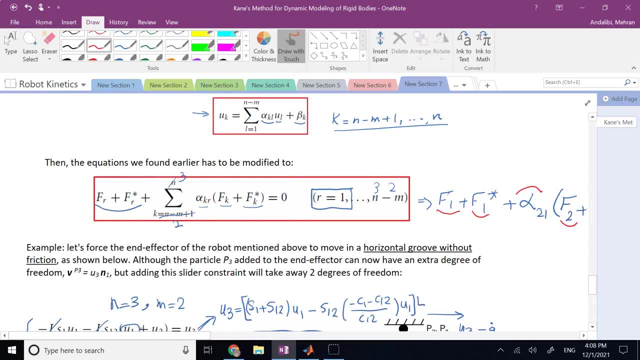 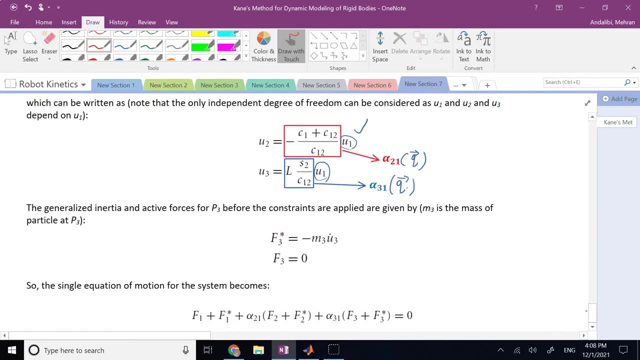 My equation of motion is done And the question is: What is F three? and what is F three star in this case? right? So F three in this case is zero. Why? Because F three means what Means the active forces, the generalized active forces on P three. 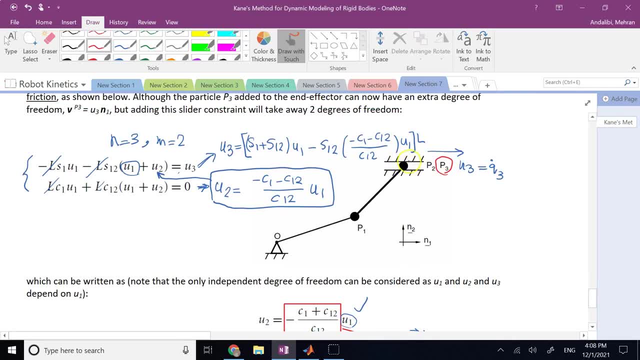 Well, P three, or this particle that we put on the end effector, There is no active force on it, because the only three forces that are acting on it Are what From outside environment Is M G, or M G is already actually calculated. 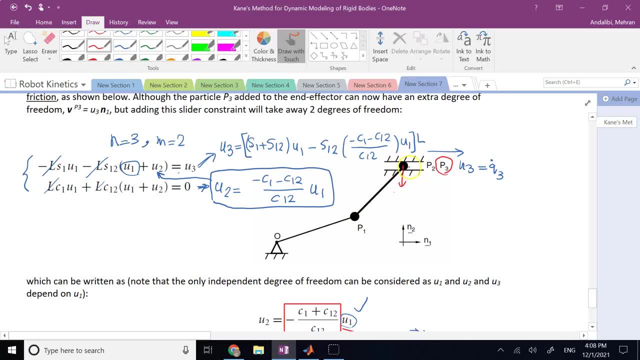 I don't even need M G for that, Because this is really this. This is like a massless particle, This P three. The mass of it is already considered in P two, So the mass that you associate with P three is actually really zero. 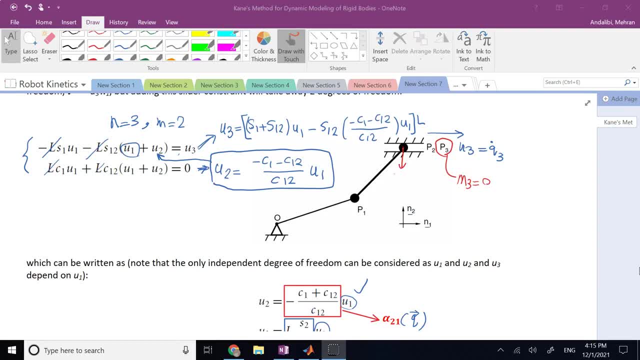 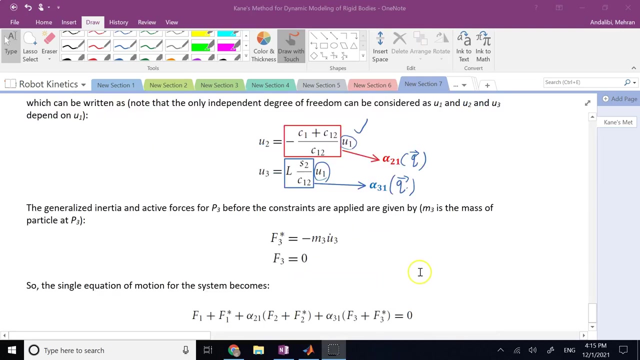 Unless this end effector here is to grab something In this slot and want to basically manipulate and move it. If that's the case, then yes, P three can be considered a separate particle with mass M three And you can consider that, as you can see here down in this equation. 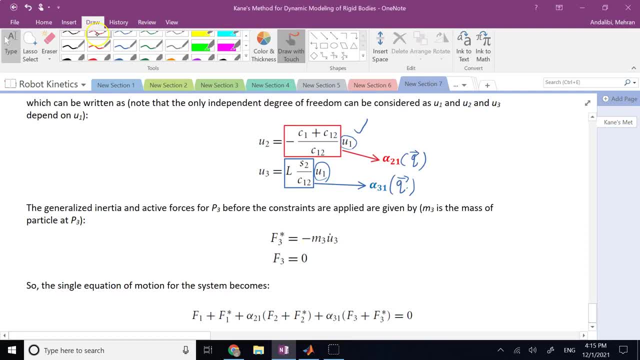 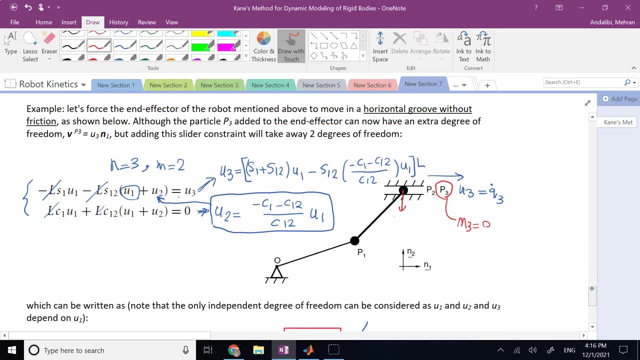 There is some M three is considered, And because in that case we are explaining or describing the problem In a different manner. We don't say we force the end effector to move in the slot. We say the end effector has gone into the slot to grab a particle of mass M three called P three. 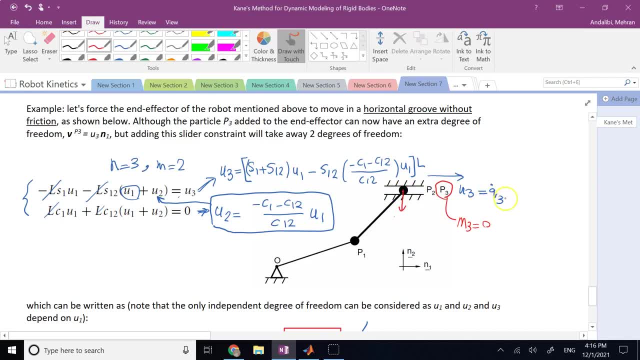 And now it is moving it. Okay, But again, if the end effector is just to move inside it without really grabbing some particle P three with mass M three, Then you can use zero for M three. So but even at most you have this M three. 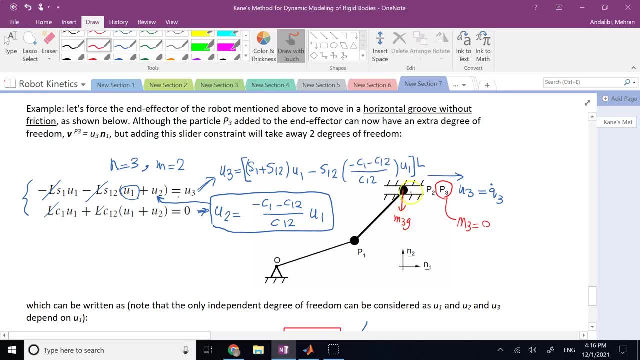 G, which is definitely not an active force. Why? Because the end effector here with that particle or itself, has to move horizontally. This force is acting vertically. The normal force from the walls also is not an active force. It doesn't do any work, right. 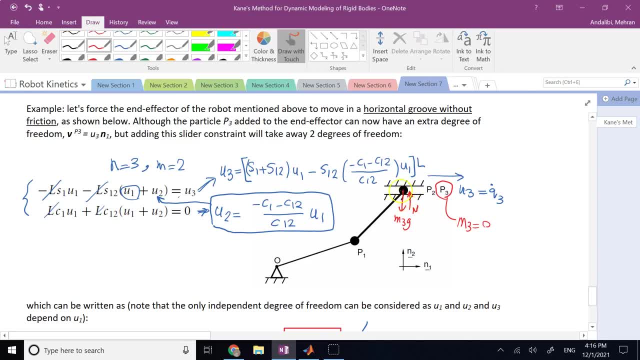 So there is no force. The only force that could have existed and had any contributing Active, general active force was friction, Which would be in the same direction as you three or opposite to that. But here I said there is no friction in the groove. 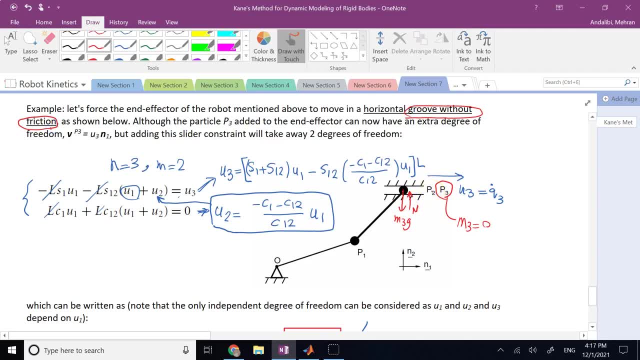 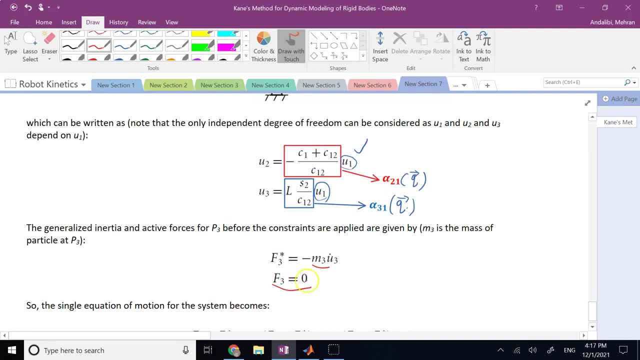 So that's it, And therefore there is no active force. Therefore I can say: my F three is simply what? equal to zero? If there was a friction, then you have to add The velocity Of particle three Right For the R that you have. 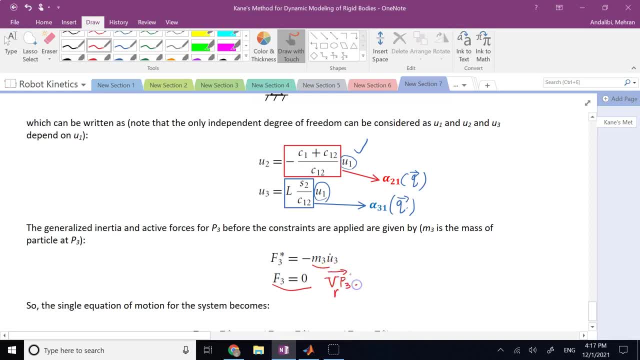 And here you actually only have one R And dot product, this with that friction force Which was equal to negative Of mu K times N, Which in this case is MG, And then in the N one direction. Okay, So then you could do it like that: 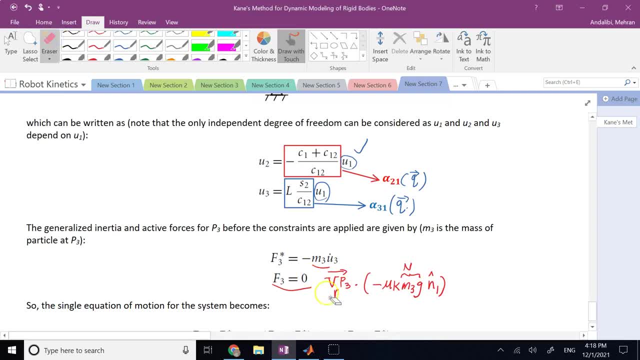 But in this case, since there is no friction, F three is equal to zero. And then your inertial generalized force, As we all know, is equal to negative M times A And A is U three double dot, Because U three is velocity. 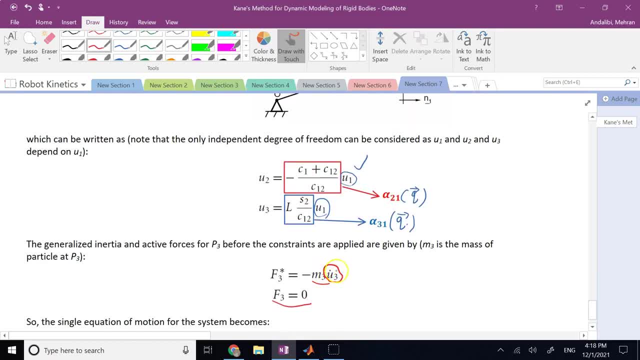 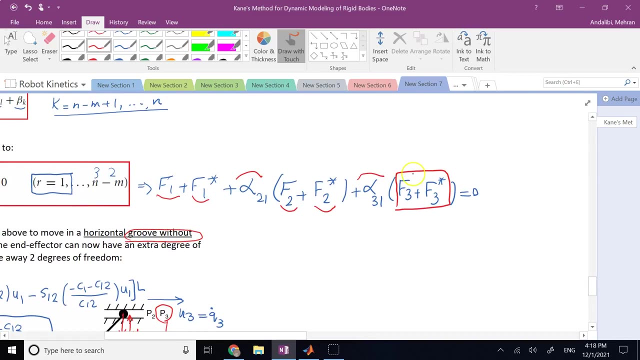 So acceleration of that block is U three dots, Which is like Q three double dot, So negative M three U dot is definitely what Your inertial force. So calculating F three and F three star Is also no big deal in this equation. 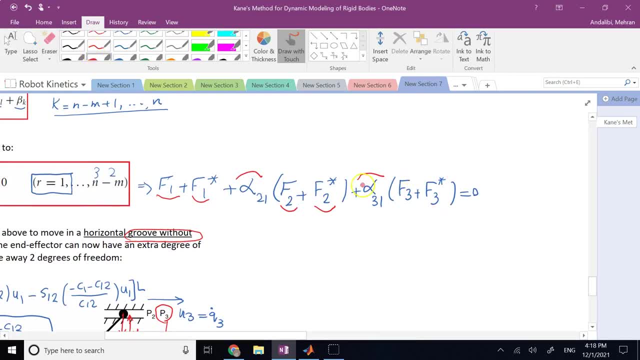 And once I have those Then I can combine everything together, But you clearly can see That I used something that I have already derived. All I had to add because of this constraint Were F three and F three star to calculate, And these alphas: 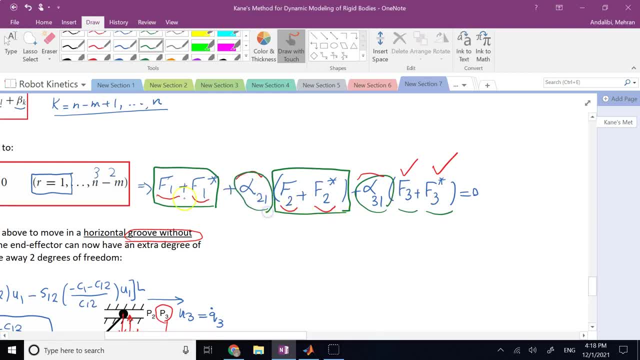 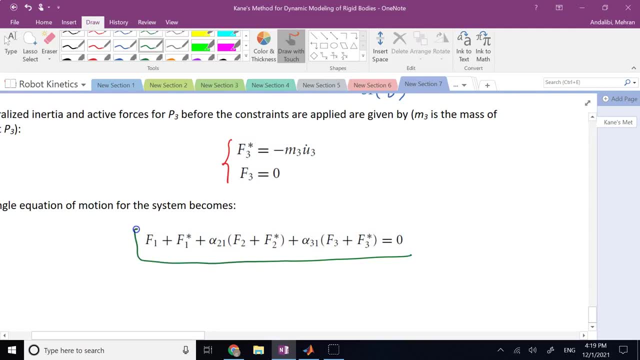 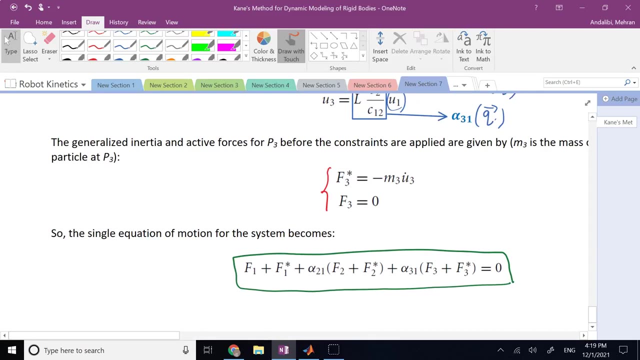 Once I can calculate these, I combine them with previous information And now I get my single equation of motion That I will have for the single degree of freedom For R of one Right Or U one basically here, Although U one alone will not be included.